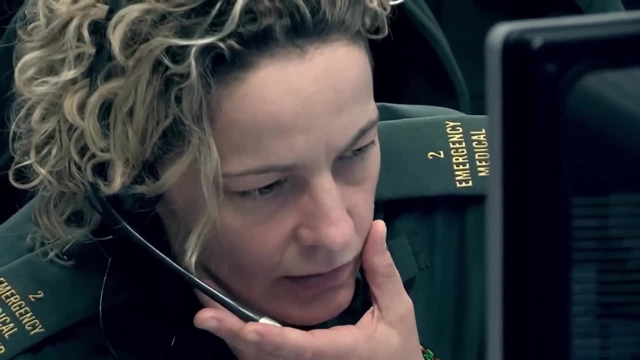 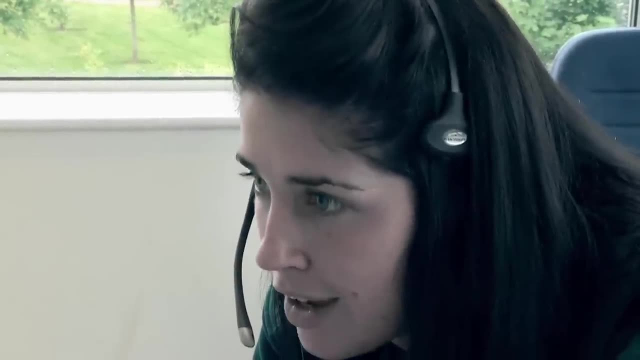 Okay, look at him close up And tell me if he's breathing at all. Filming with ambulance call handlers- You need to puff the chest hard and fast at least twice per second- And paramedics across Britain. I think we're going to have to go up, Neil. 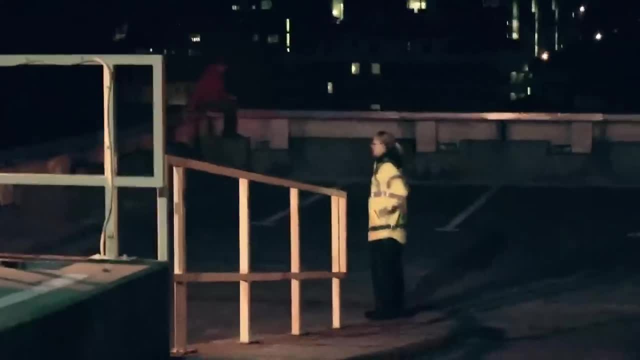 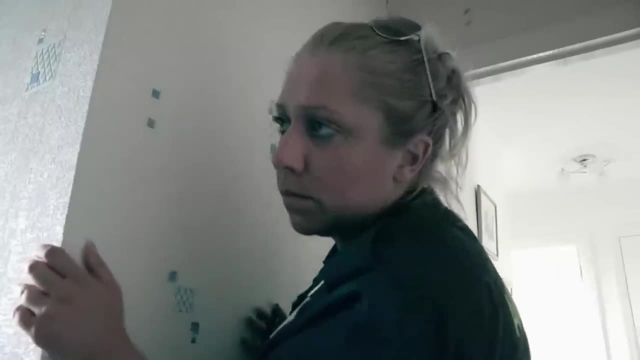 What are you doing out here? I'll stay back. No, I'm staying back. I'm staying back. I'm staying back. What's wrong, mate? This is the story of why we're in greater need of the ambulance service than ever before. 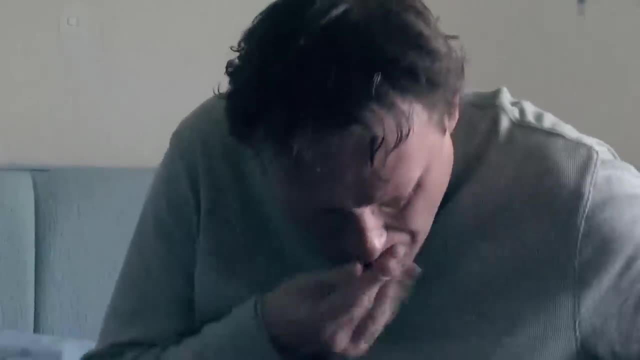 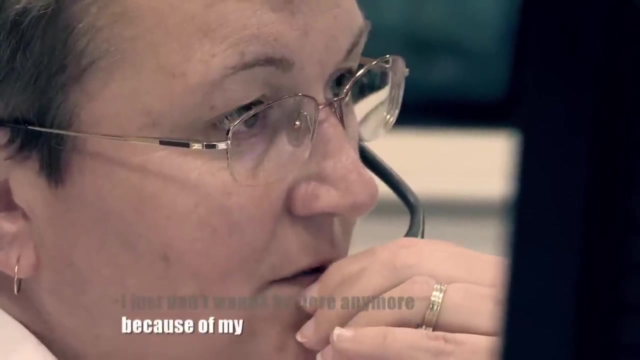 Mate, we don't want you to take an overdose. I don't give a shit. I'm desperate to get help. Help me. I just don't want to be here anymore because of my appearance. It's what's inside, though, isn't it, sweetheart? 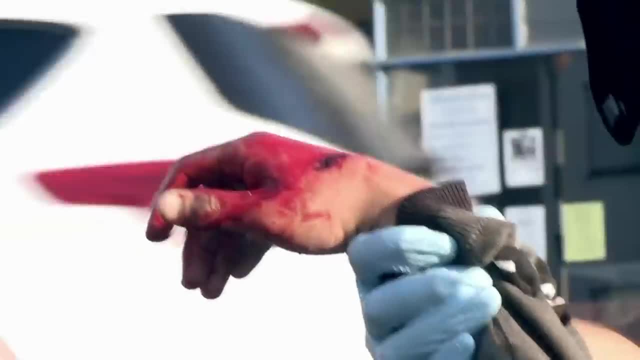 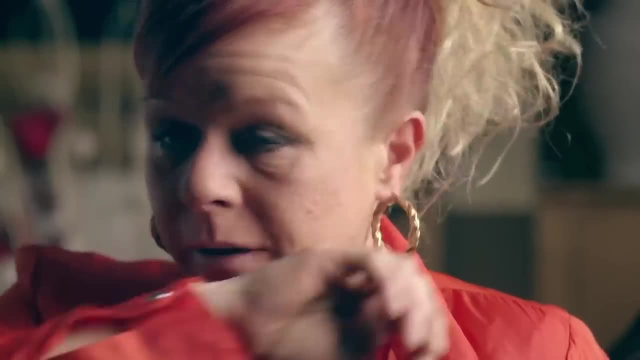 It's not me, It's my friend. He's been stopped Of emergencies that change lives forever. I just remember him laying down here and me then thinking that's it, Give me a hug. And what happens when the medical emergency is over. 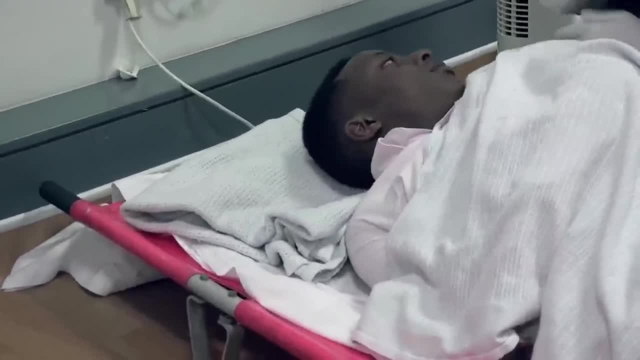 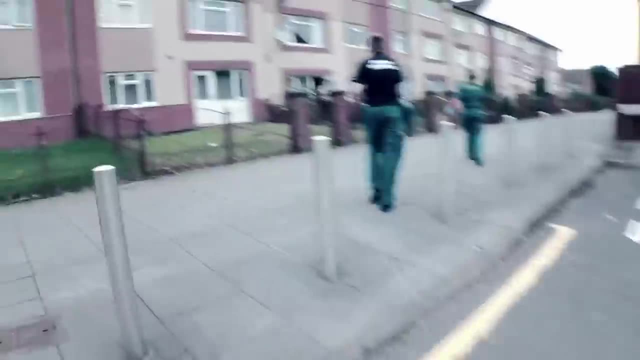 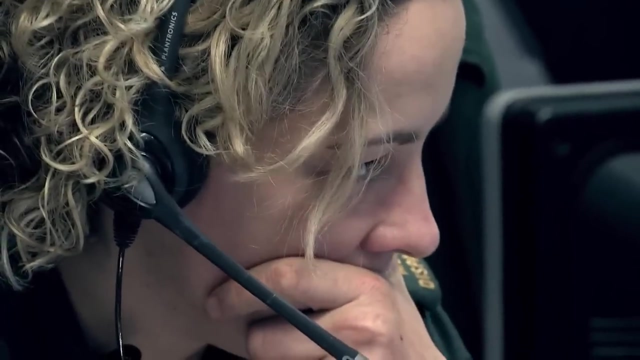 James lay down, mate James lay down, listen. And the paramedics have left. Don't worry. Where is he This time? patients found in the moment between life and death. He's not breathing And the toll it takes on the staff who must deal with them. 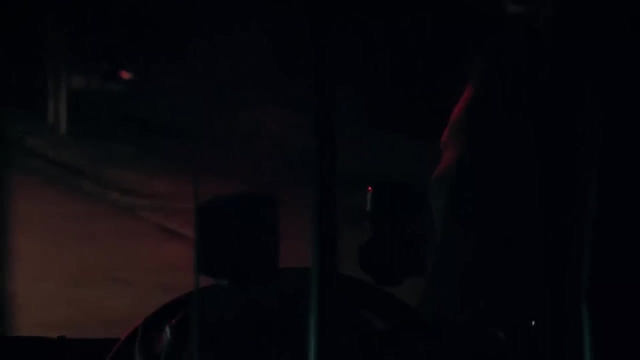 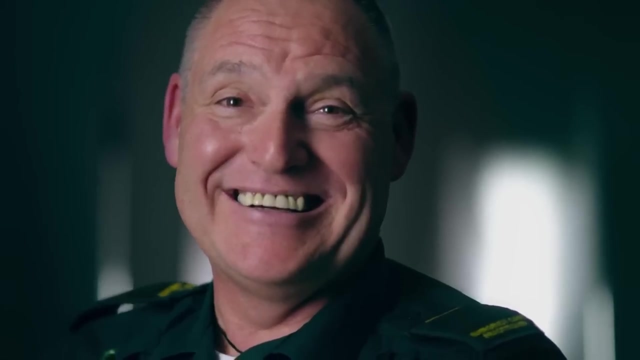 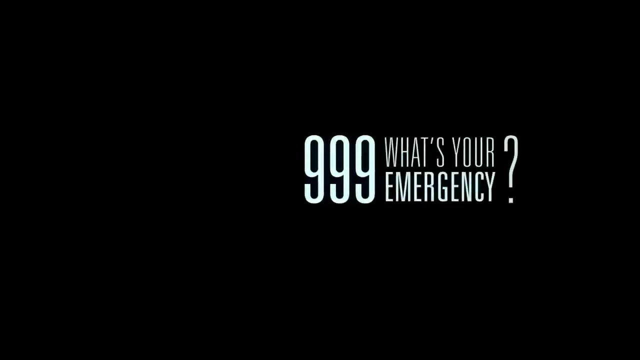 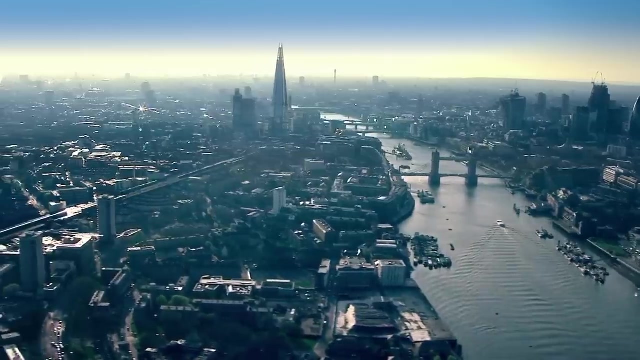 If you keep having these things thrown at you, what type of person must you become? The way I look at death, it's the last great adventure. Nobody's ever come back to tell me otherwise. Tell me exactly what's happened. He's choking, My father's choking. 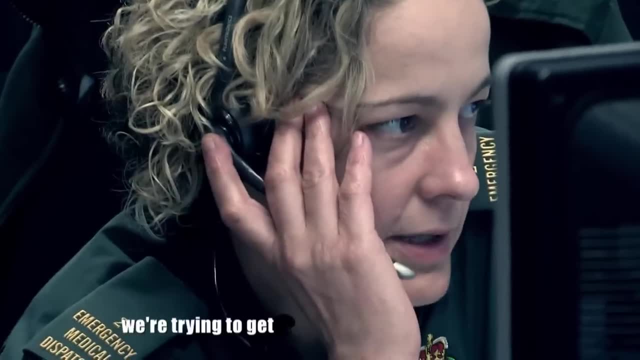 Are you there with him now? Yeah, yeah, yeah, he's dead. We're organising the help right now. How old is he? He's 70 years old. Is he awake? No, he's not answering. Is he breathing? 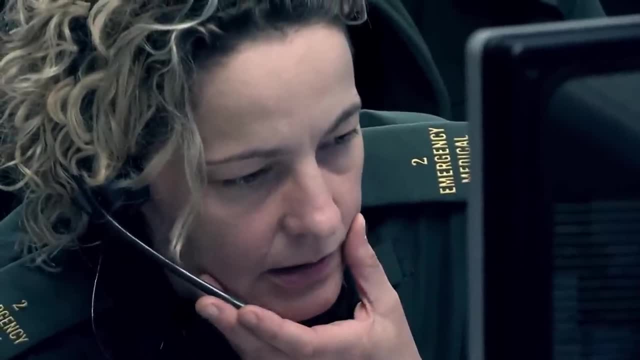 No, I don't know. OK, look at him closely and tell me if he's breathing at all. No, he doesn't look like he's breathing. Ambulance service, tell me exactly what's happened, please. My mum's collapsed. 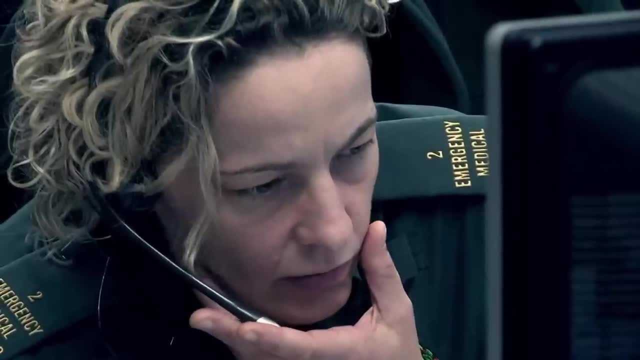 She has a hole in her heart and she's like laying across the floor. Listen carefully. I'm going to tell you how to do resuscitation, OK, OK. So make sure she's flat on her back on the ground. 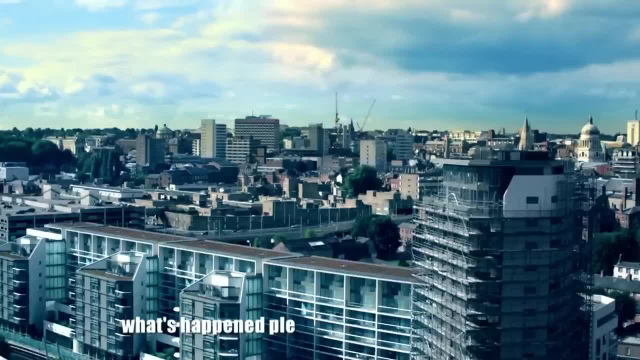 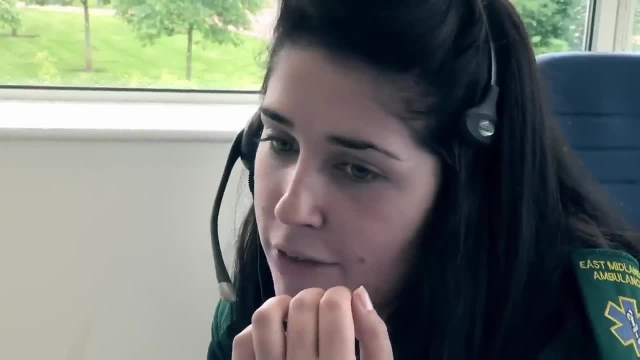 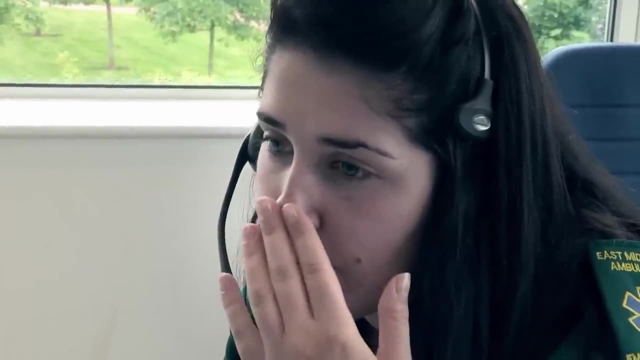 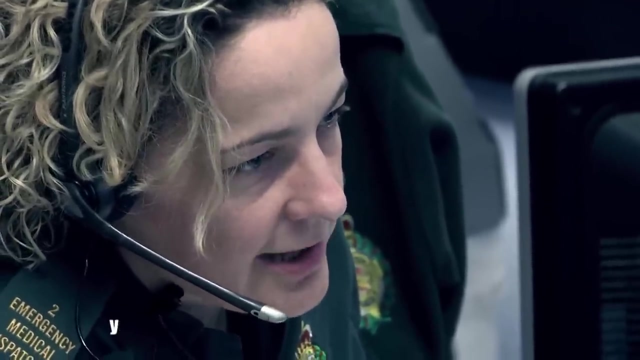 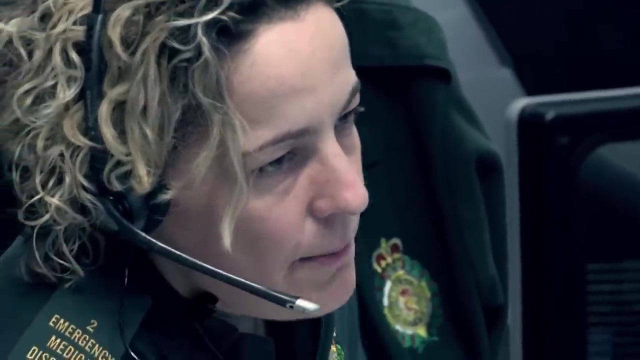 You need to place the heel of the hand on the centre of the breastbone, in between the nipples on the chest. OK, On the chest, Put one hand on top of the other hand and you're going to push down firmly two inches. 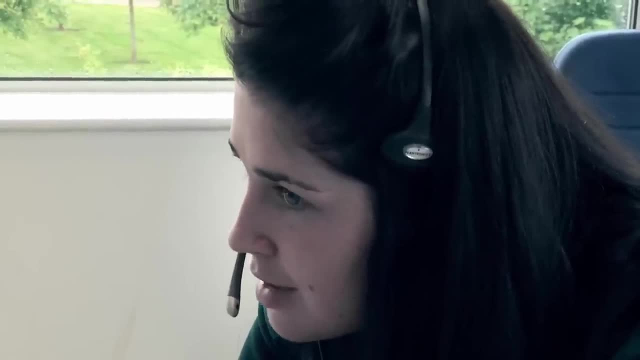 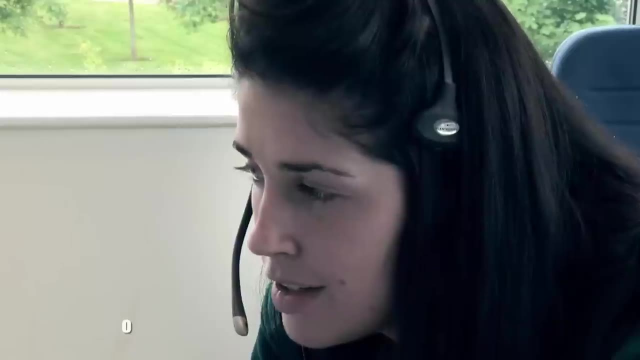 with the heel of your lower hand touching her chest. OK, Right Now, listen carefully. You need to pump the chest hard and fast, at least twice per second. OK, And we're going to do this 600 times or until the help takes over. 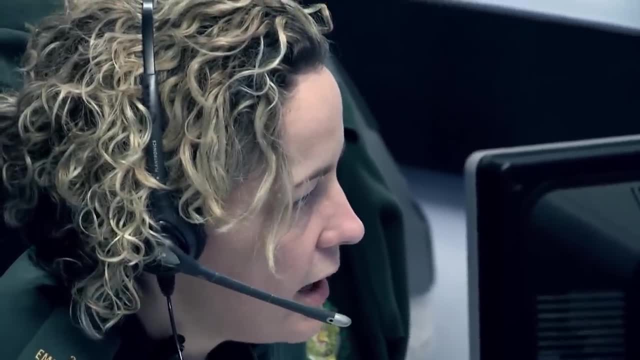 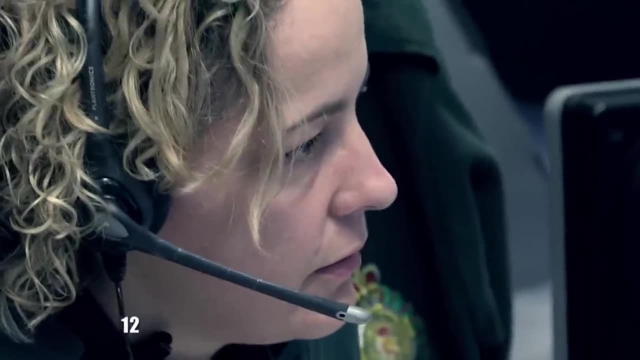 And I want him to count out loud to four And this is how fast we want him to go. OK, 1, 2, 3, 4.. 1, 2, 3, 4.. 1, 2, 3.. 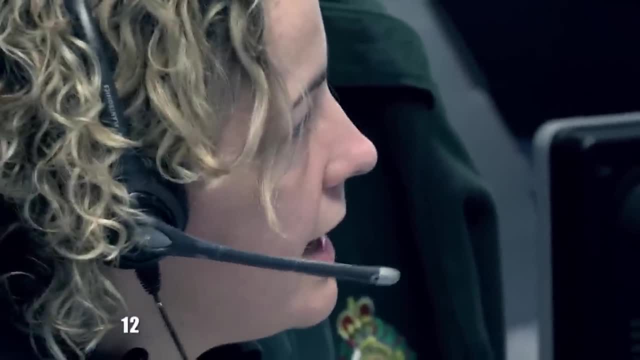 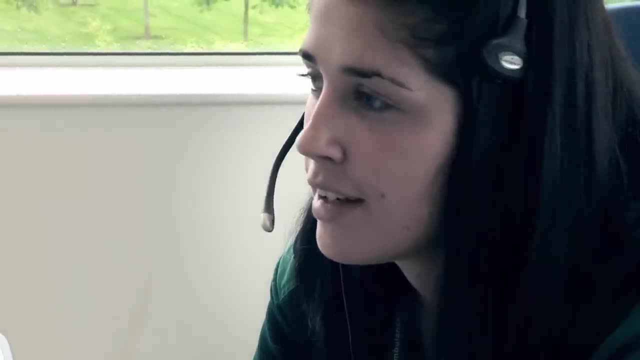 1,, 2, 3.. That's good, Just keep that pace and don't stop until the help takes over. Three, four, one. two, three, four, Brilliant. keep going. for me An adult here now, sir. 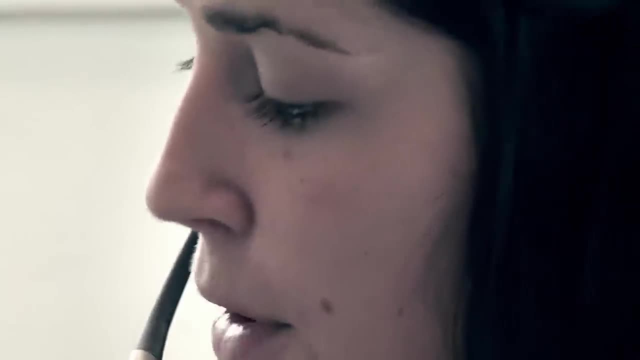 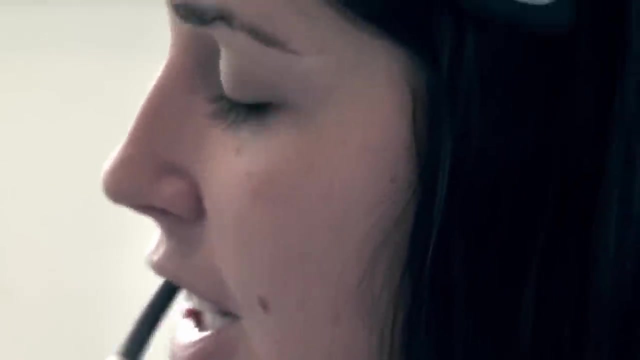 There's an adult there, Right? okay, don't stop. I don't want you to stop. Don't stop, Hello. Hello, it's the ambulance service, Right? he needs to continue with what he was doing, Right, What was he doing? 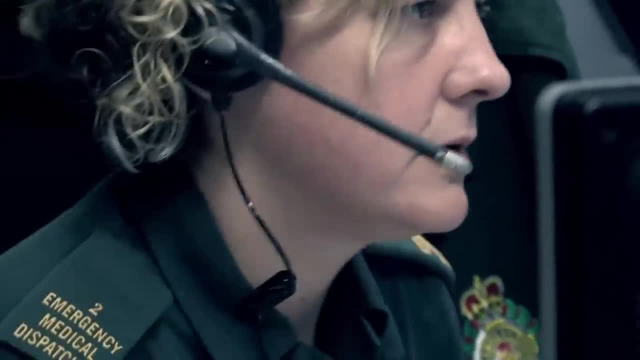 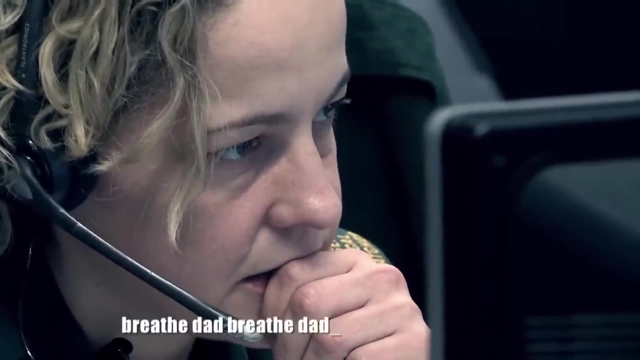 I'll tell you when. hello sir. One, two, three, one, two, three, one. Breathe Dad, come on, breathe Dad, Breathe Dad, breathe Dad, Come on Dad. 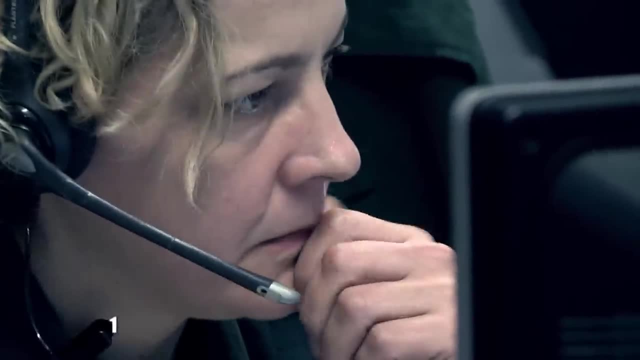 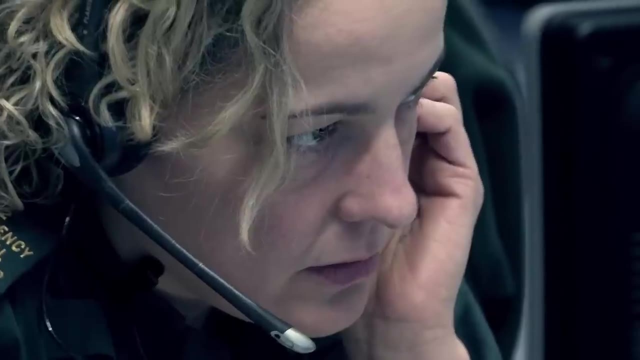 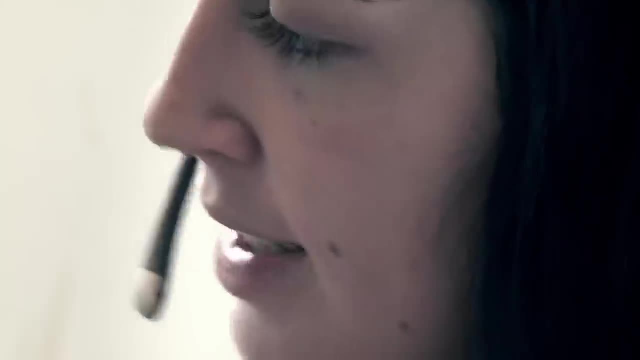 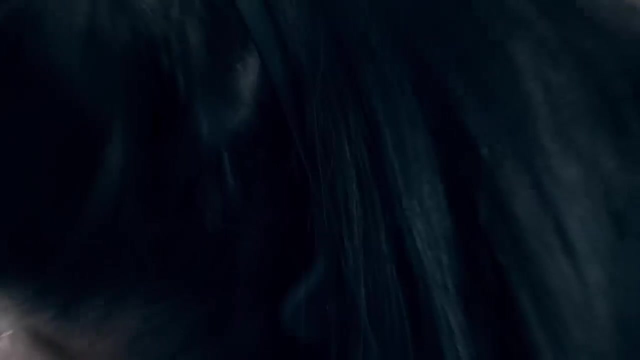 We can't stop in between Right. okay, So is he doing that Right now? No, Right, just tell him to go back to doing what he was doing so that I can tell you what to do next. It's really important. 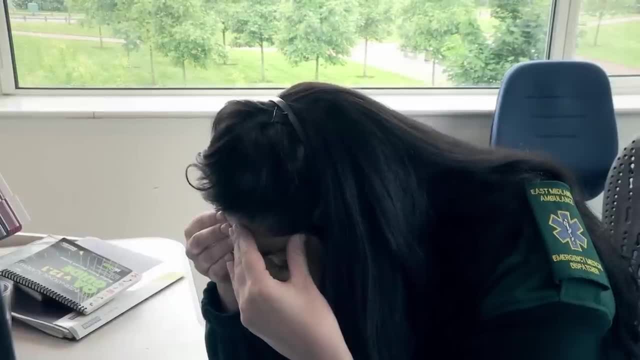 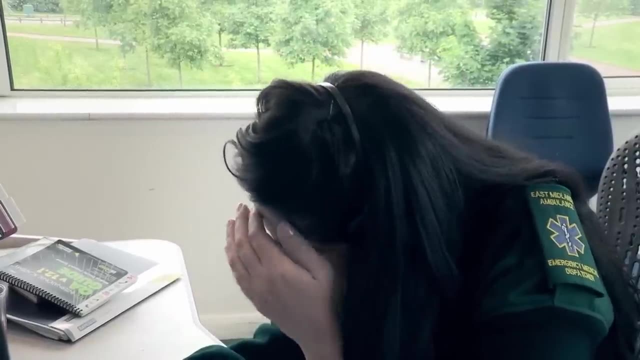 What are you gonna do? Move. It's really important. Go Right, I'll take that off like that. Just tell him to keep going, and now I'm gonna tell you how to do it. Daddy, Daddy, No, no. 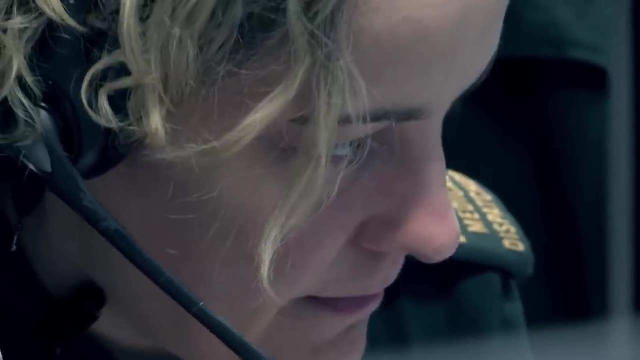 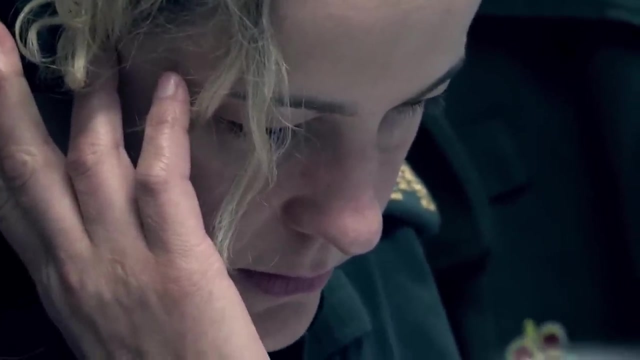 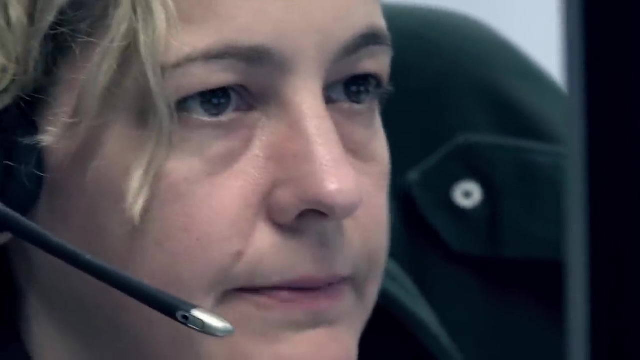 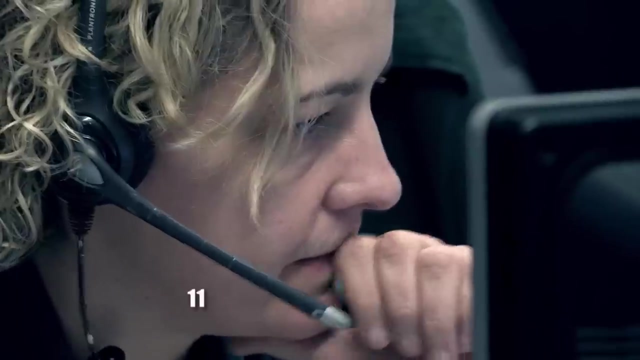 Oh my God, What am I gonna do? Please, please, Breathe. What. How long has he been like this? Oh, under a month. Don't do it, Can't see him. Thank you, Didn't? that was horrible. 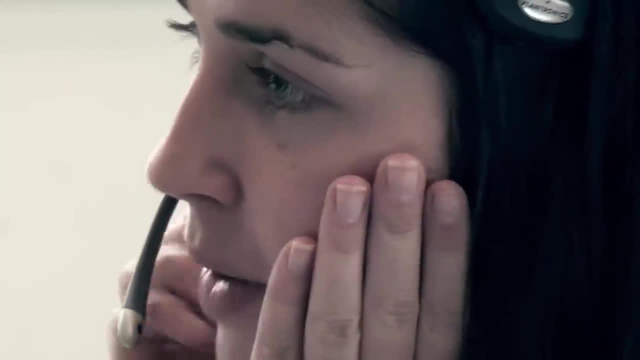 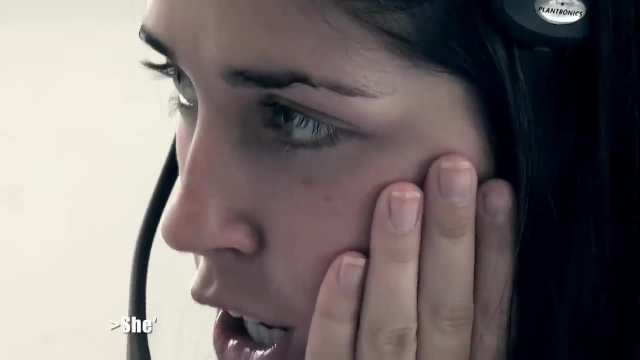 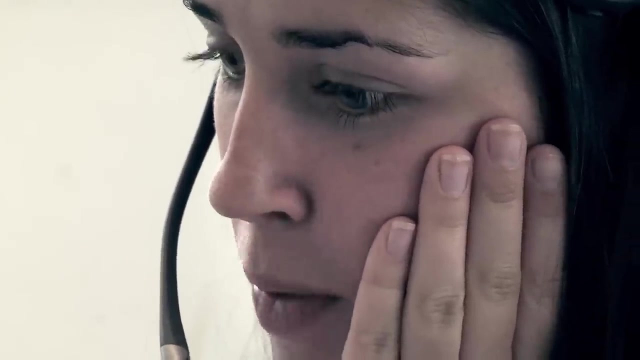 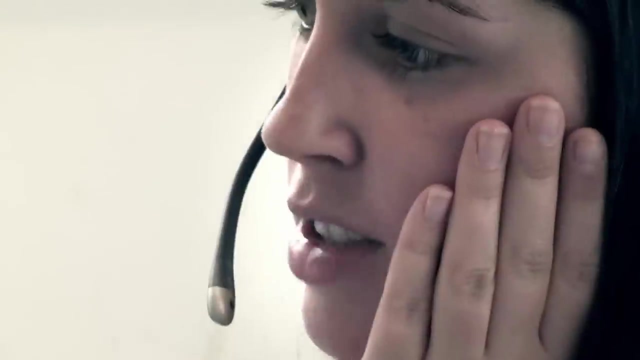 One, Two. No, that we're going to go at this pace. okay, one, two, three, four. one, two, three, four. one, two, three, four. she's coughing. is she breathing? she's choking? right, just turn her on the side for me. make sure she's breathing, okay, and is she breathing? yeah, right, okay. what i want you to do, then, is: 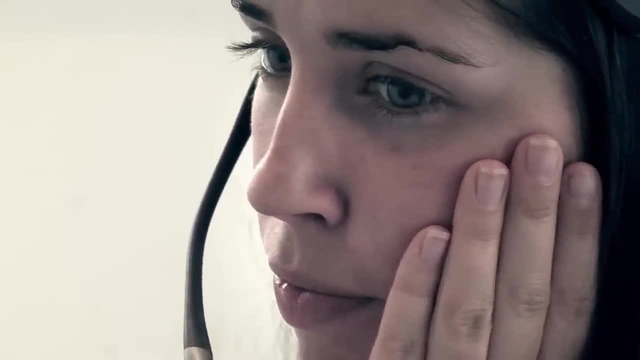 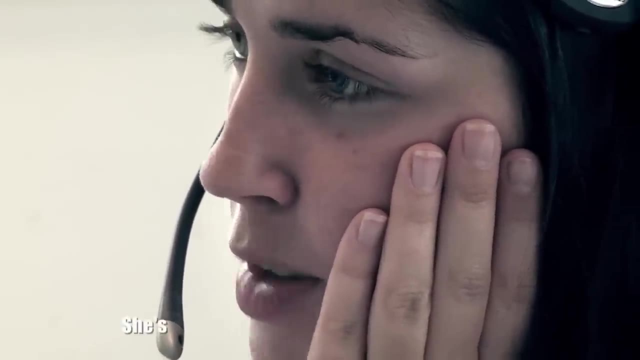 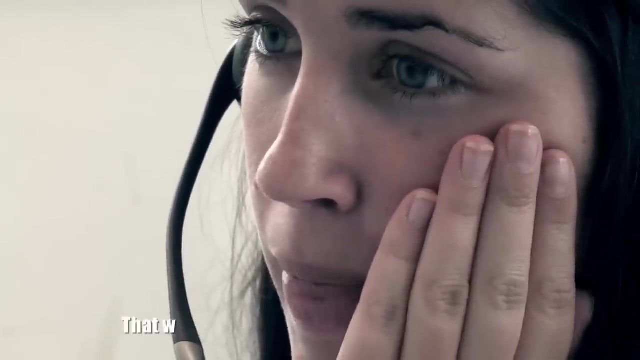 i want you to tell me every time she takes a breath: yeah, she's breathing now. okay, now tell me when the next one is she's breathing normally. now, she's breathing normally, is she? yeah, who was it that i spoke to first? that was her phone. that was her son. how old is he? 13, 13, he did really. 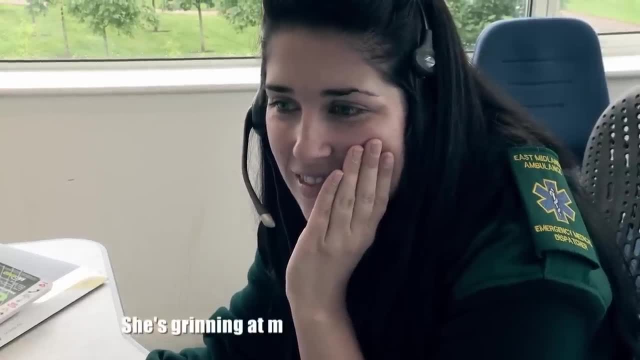 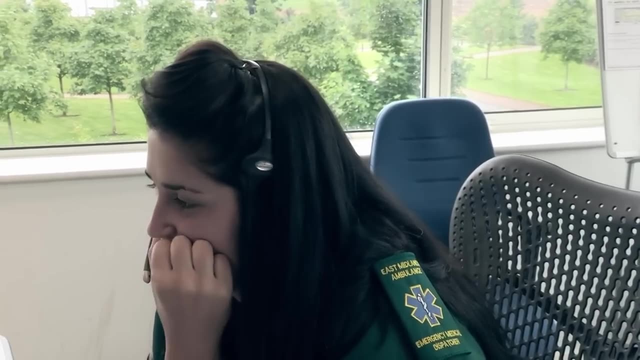 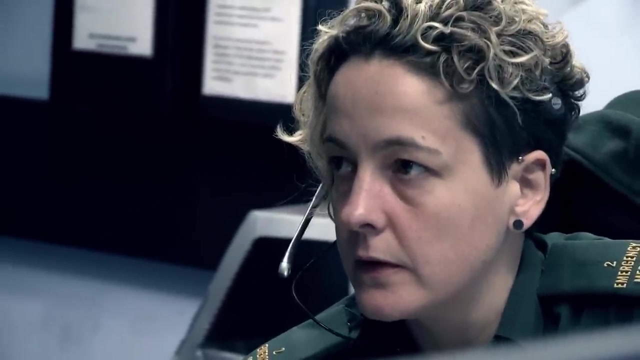 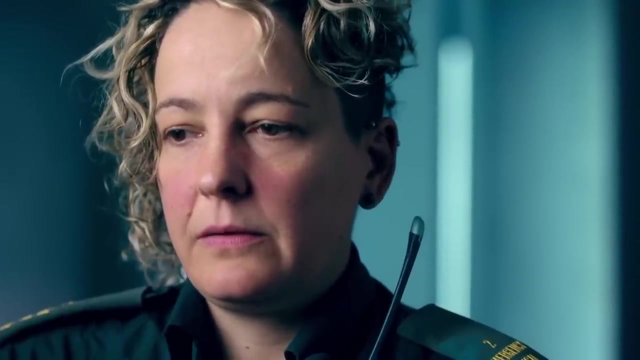 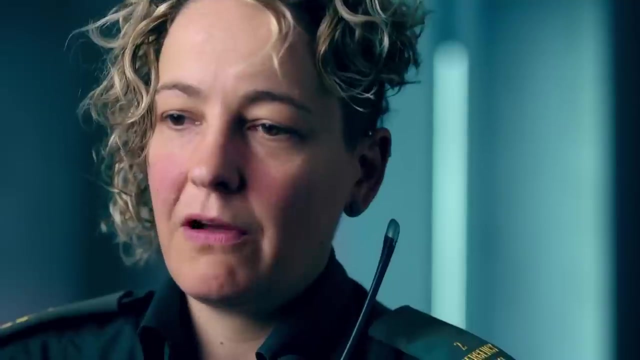 really well. she's just opened her eyes. she's grinning at me. now what's your answer? you just want to just carry on. i just want another call. i just want another call. it's just a mundane, everyday call, where someone's life isn't hanging in the balance, you know. 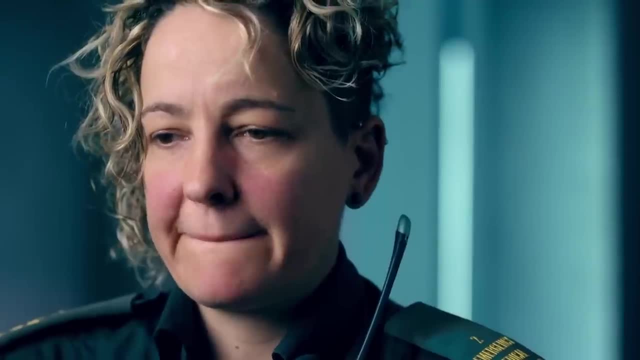 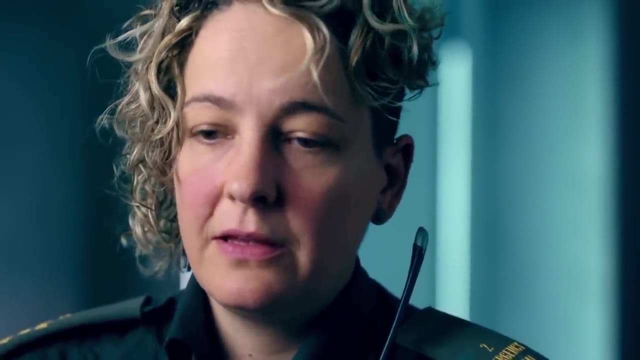 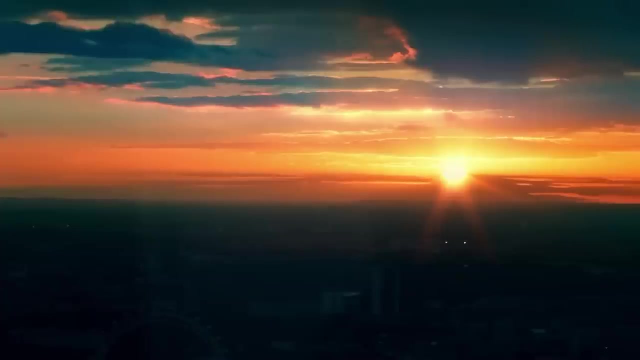 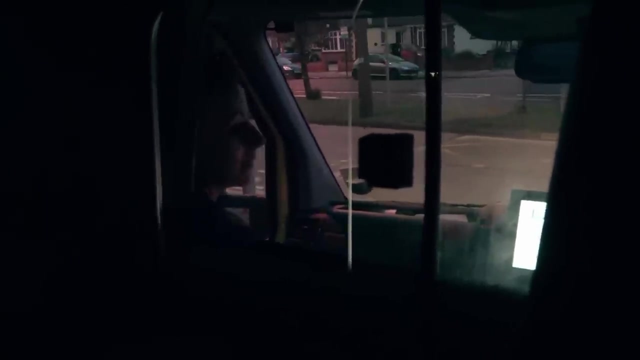 and i just try to um, leave that last call somewhere else and and not really focus on on it. otherwise I would just fall to pieces. Another day breaks short sigh. For some it will be the best day of their life, for others it will be the worst. 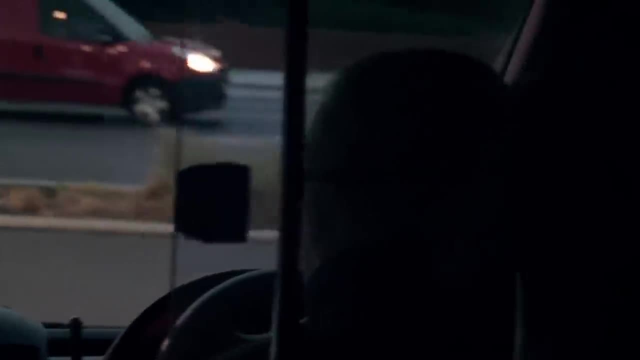 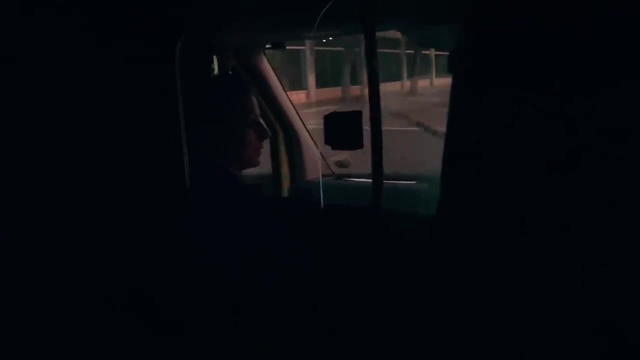 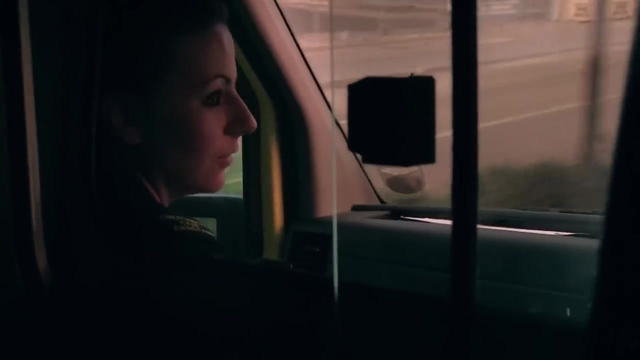 Ambulance service staff face more than 8,000 life and death emergencies every day. So once I brought a coffee from Starbucks- yeah, Medium-sized latte- piping hot- Back at my old work. So I'm on the terrace- yeah, I've taken the lid off to let it cool it. 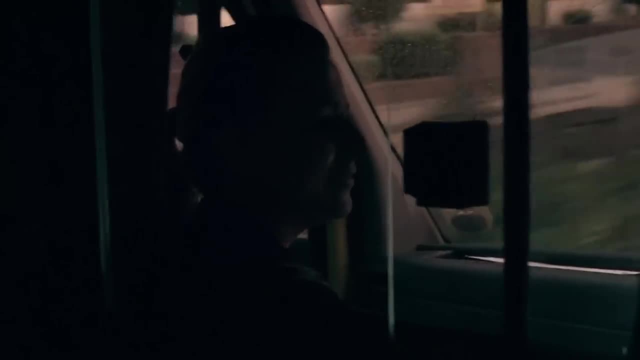 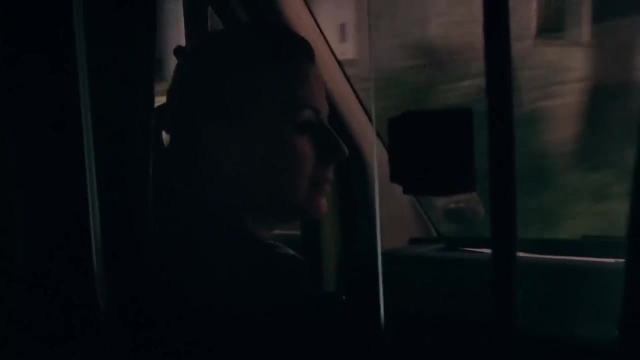 was that hot? It's a bloody seagull, which we called Stephen Seagull. Did you get that? Come down, got it and flew off with it. What a lid, A medium, yeah, What the whole drink. 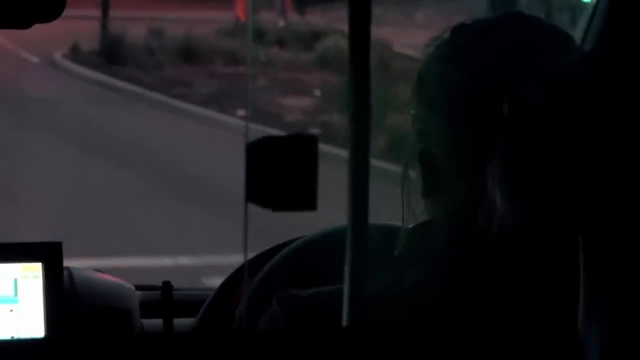 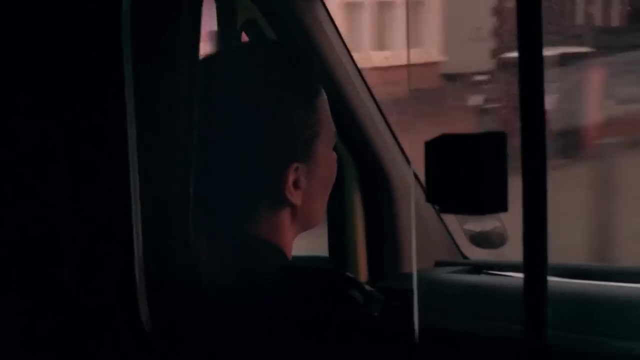 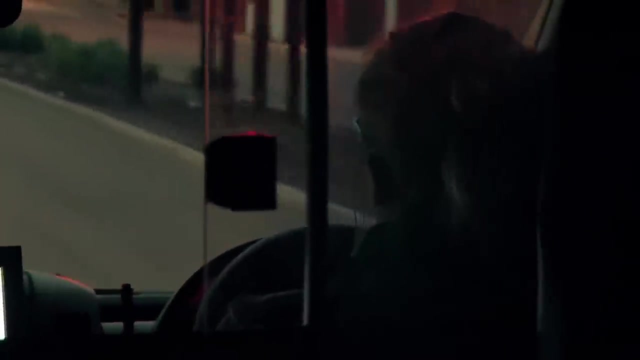 The whole. coffee, A medium-sized latte, brand new, Flew off, Went over the town centre, didn't spill a drop. Crazy mofo. Anna is newly qualified. She's been in the job less than a year. You need someone like that. You need someone to just think differently to you, A lot differently. 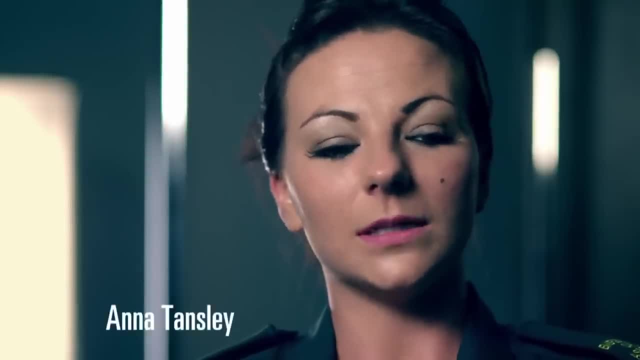 Do you know what? when I started, people were like: oh, you're excited now we see it all the time. give it a couple of weeks. a couple of weeks went, still excited. give it another couple of weeks, give it two after. 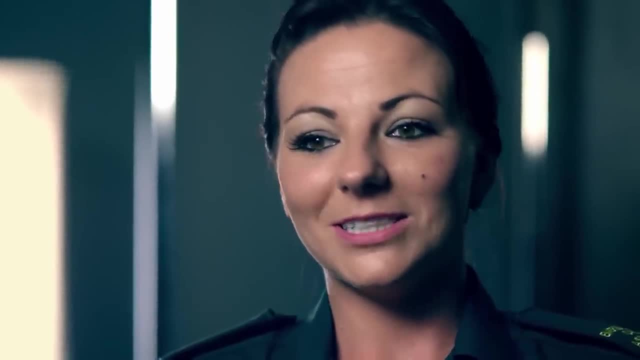 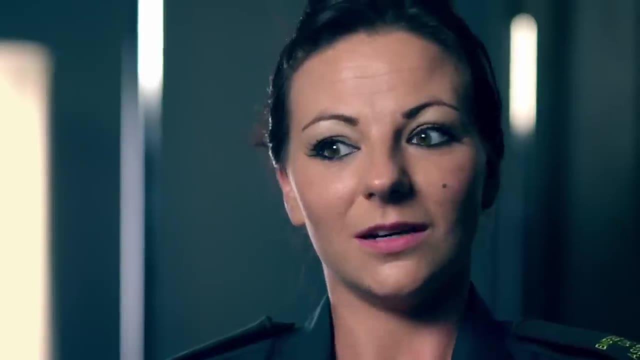 Christmas. once you've experienced Christmas, Christmas coming. I'm still as excited now as the day I got accepted And that's not going to change. People think I'm just. you know I'm crazy and something's not quite right, but everything is right up here I. 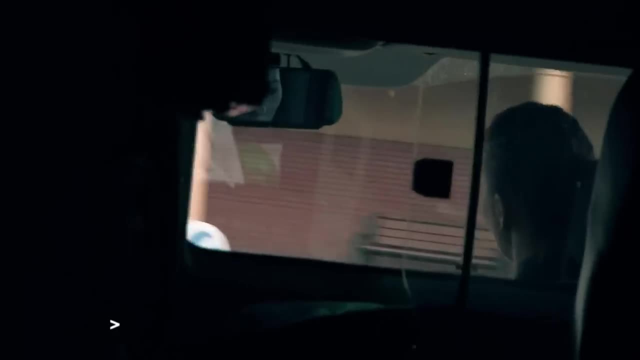 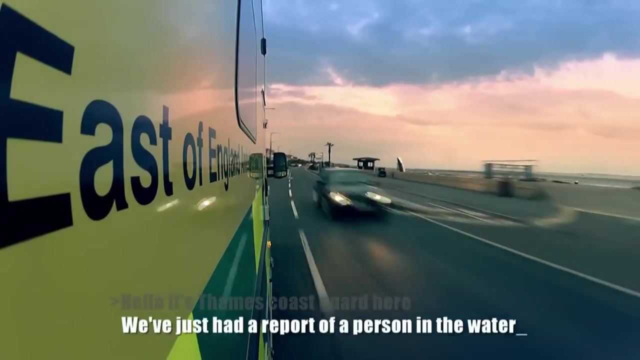 just love this job and I love what I do. Ambulance emergency. Hello, it's Thames Coast Guard here. I've just had a report of a person in the water, So he's actually in the water on the surface. On the surface, yeah. 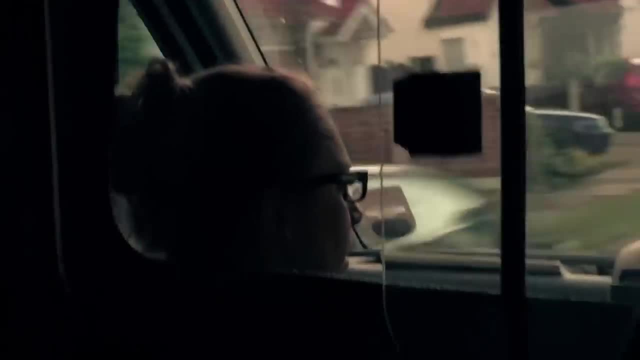 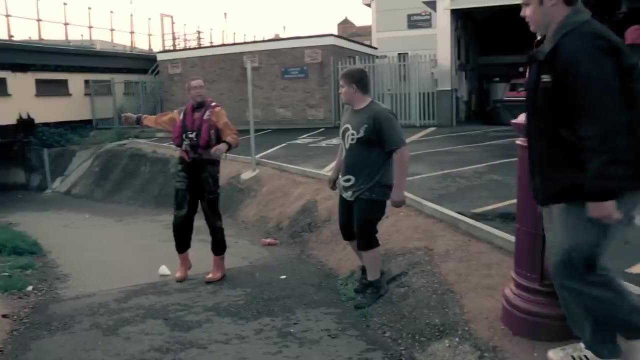 Yeah, that's right. And it's now come to a sprout. Oh yeah, we've got a lifeguard going out. We've got him just on the wall around here. Is he breathing? No, there's no CPR on him. 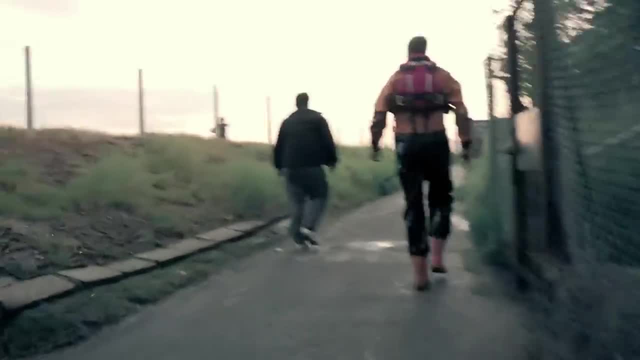 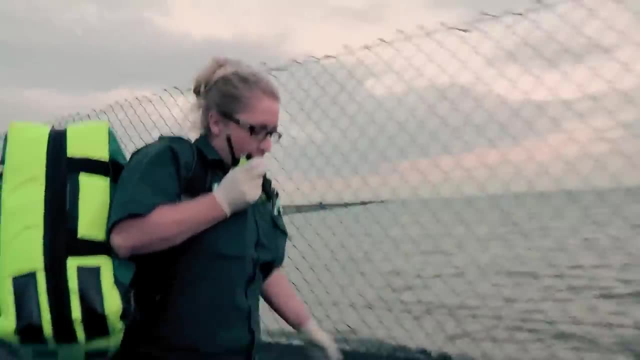 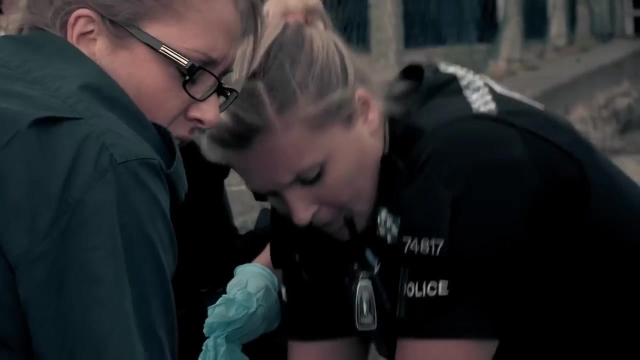 A young man in his early twenties has been pulled from the sea Unconscious and no longer breathing. Yeah, cardiac arrest, CPR has been carried out by the police. Are you all right? Yeah, I'm fine. Thanks, mate. Hey, look if you can get that suction working, because it's just not sucking up. 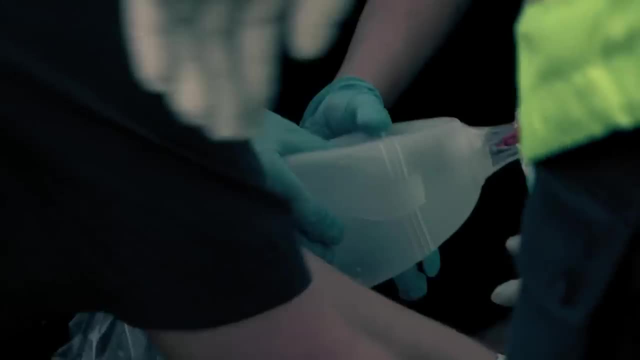 You all right for that, Are you sure? Just a regular go on and then out? Yeah, Cool, well done. I'm just going to tie that tube on. all right, You've just got to do everything you can for them. 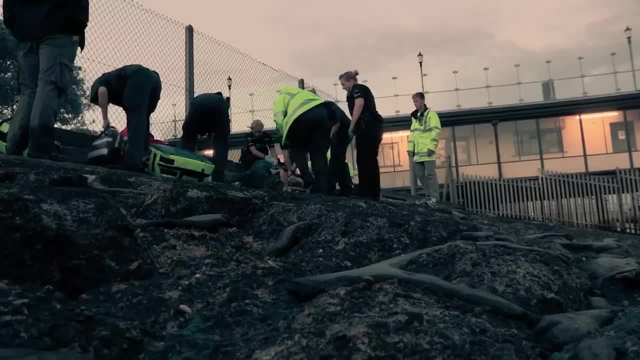 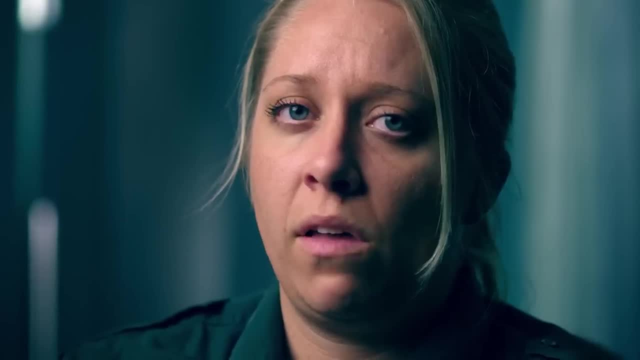 Second, adrenaline going in. okay, Yeah, All right, You know they haven't died of a condition, They've died through drowning- Drowning. there is a possibility it can be reversed, Yeah, And You can maybe save their life. 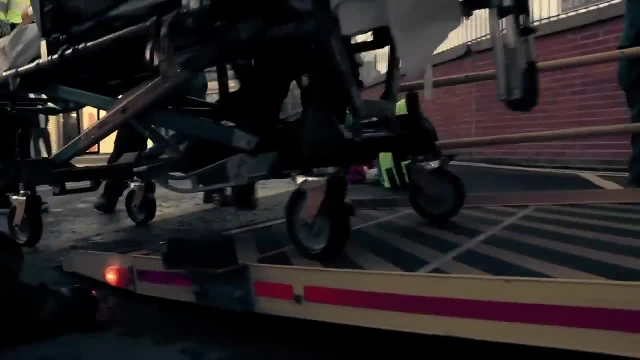 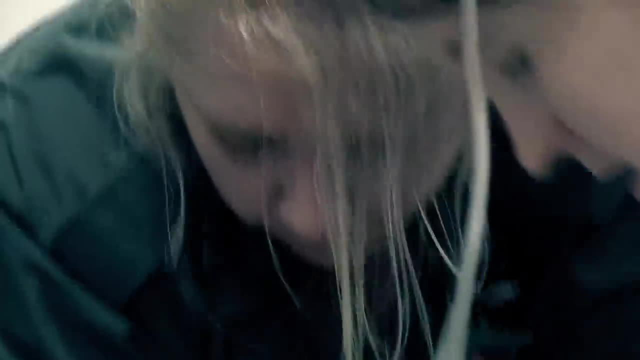 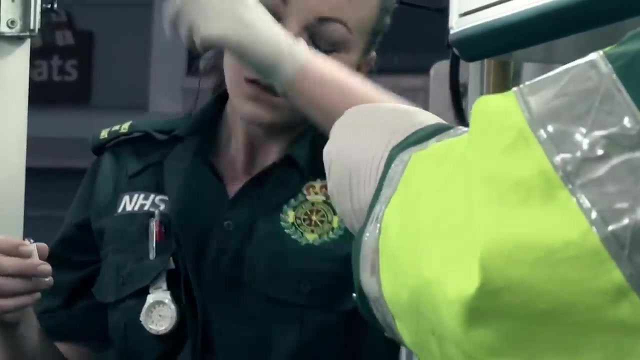 These jobs that you deal with. they are sad, some are horrific, Some are messy. It's something that people shouldn't have to see. It's just something that you have to start doing once you're in the job, and I don't think, unless you do the job, that you'd understand. 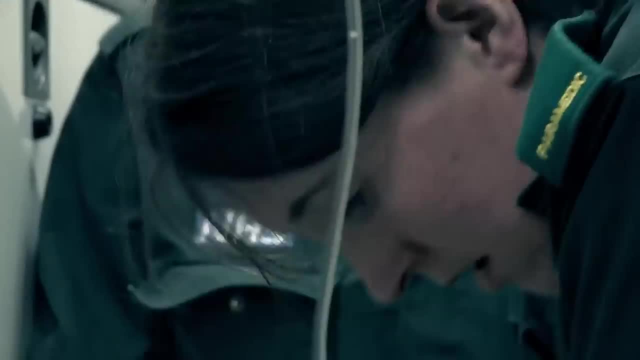 Yeah, Pulse check please. Yeah, we've got a pulse. It's very weak. As you say, it's very weak. We want it to show that we're not slapping at all now. Yeah, Do you want to start again? 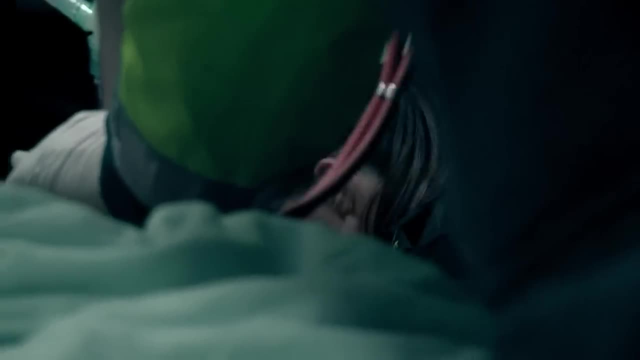 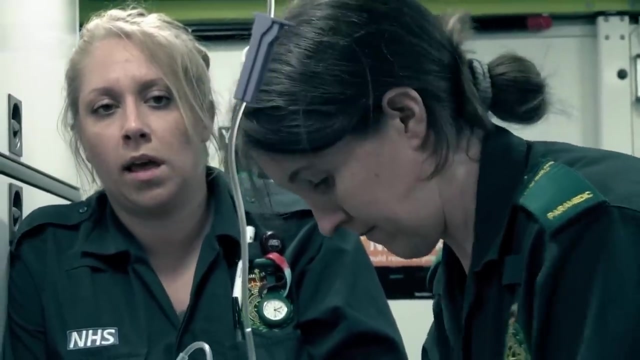 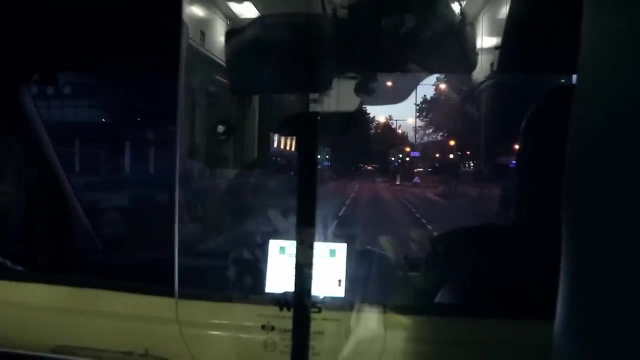 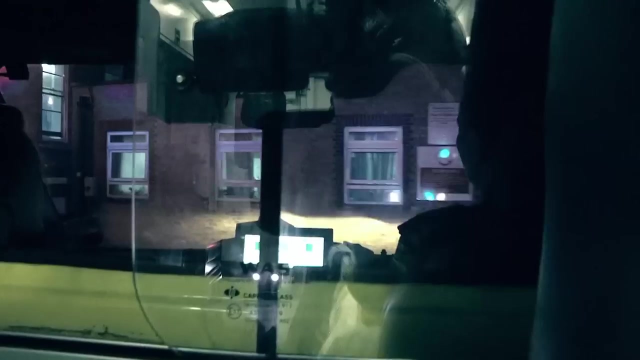 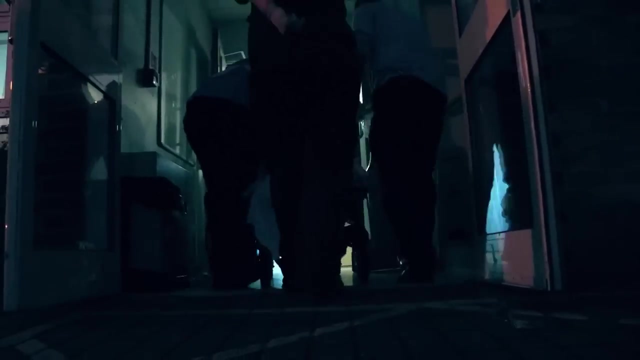 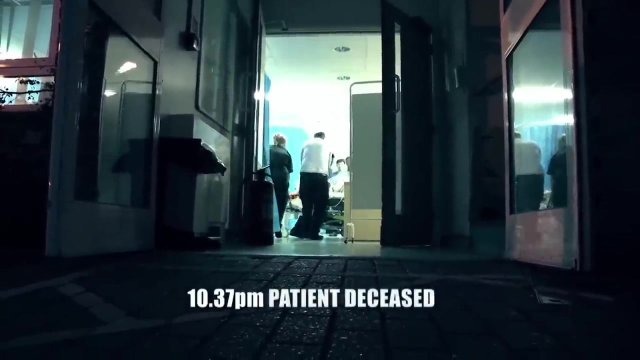 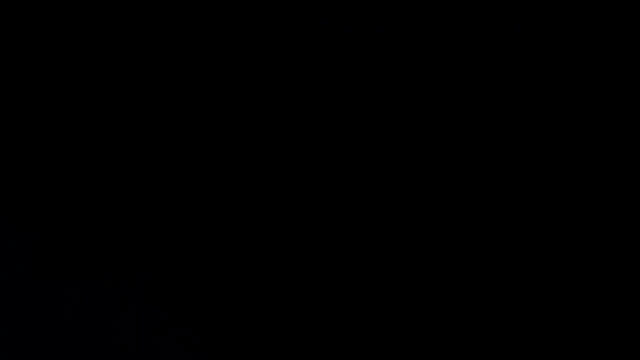 Yeah, Yeah, Just get ready to go, mate. He's been shot three times and he's had four. lots of adrenaline. Oh boy, I'm still so early in my career. there's going to be so much that I am going to remember. 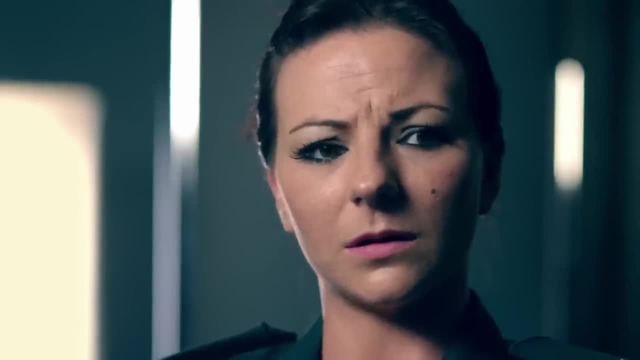 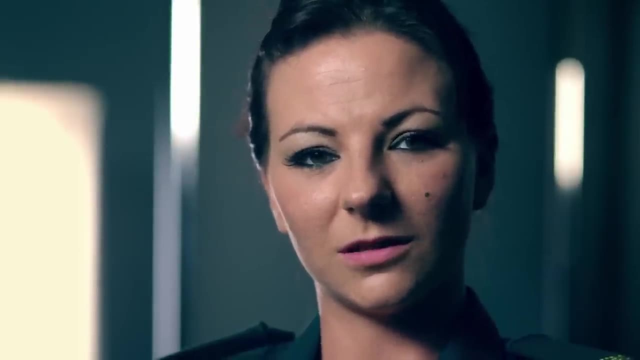 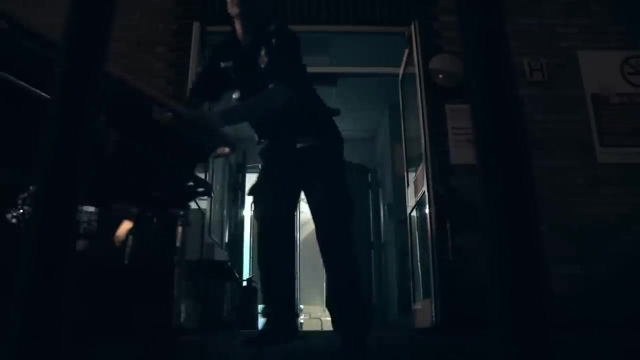 isn't there, and that does scare me sometimes, because I think I wish I could just know what I'm going to be facing, just to prepare. but you just can't. On my first ever job I went to a cardiac arrest and that was the first time I ever. 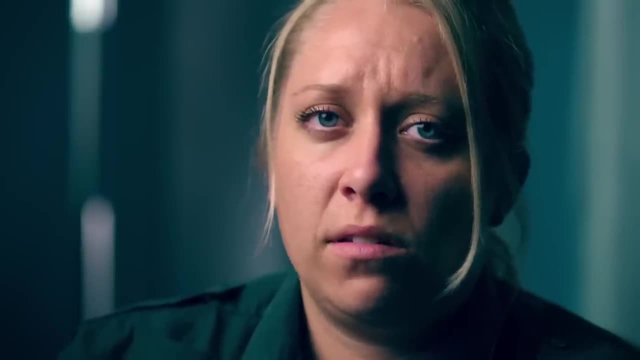 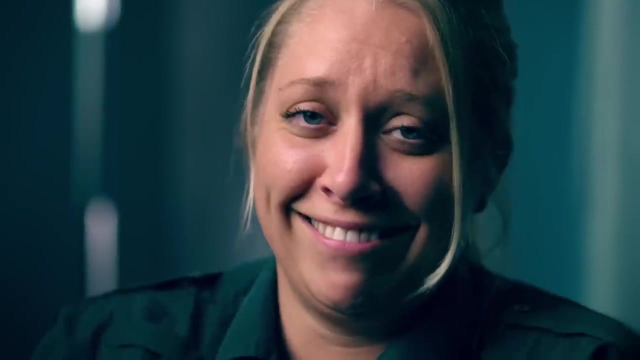 saw a dead body. To be honest, I was so nervous about going out on the first job on my first ever day that I think I shit myself when the radio went off. Then when I got to a job and someone was dead, that just topped my day off. I should have gone home there and then. 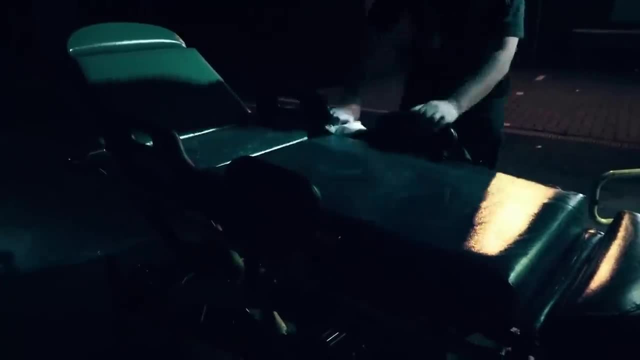 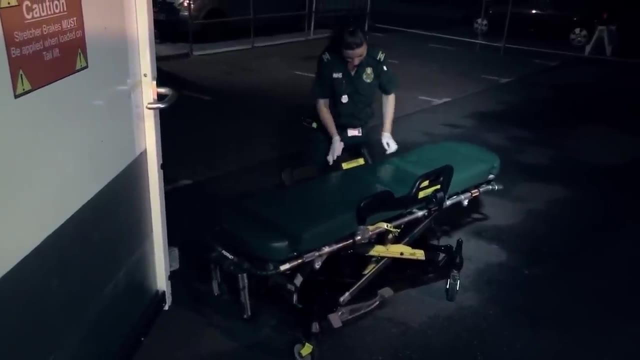 It's a shock, but as sick and twisted as it sounds, you get used to it. You couldn't say, oh, after seeing ten dead bodies, you're fine. After seeing twenty dead bodies, you're fine with it. Everybody's different, Everybody's got their limit. I don't know what point I became fine with death. It wasn't like an 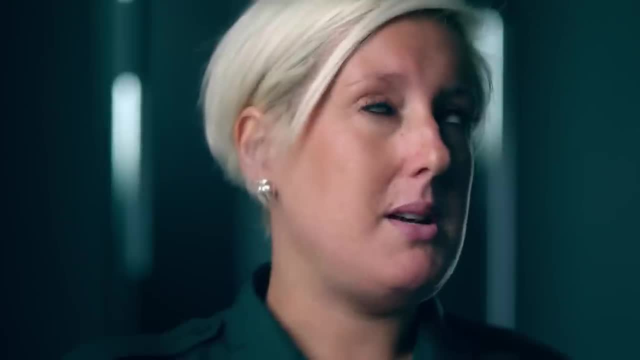 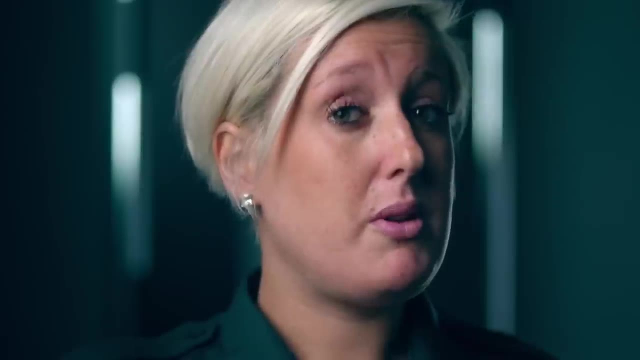 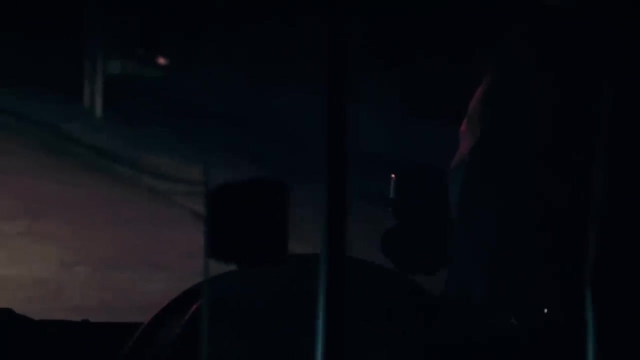 overnight thing that one day death upset me and then the next day I was absolutely fine with it And it could be just you could be rolling along fine and then one job that you could slightly relate to could really upset you. You know, if you keep having these things thrown at you, like in your career, what type of person? 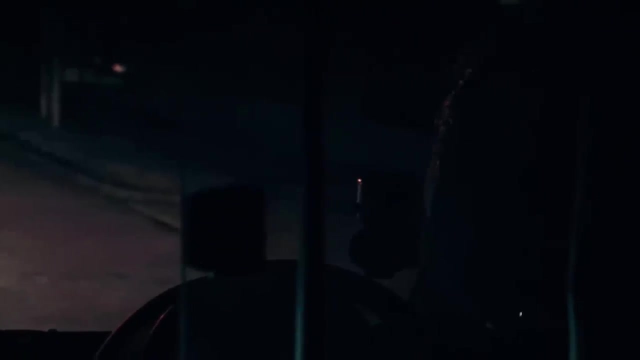 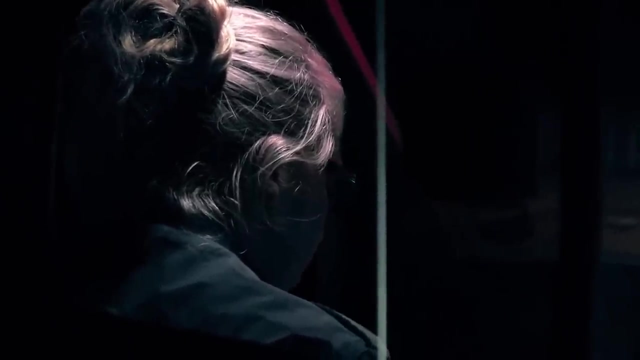 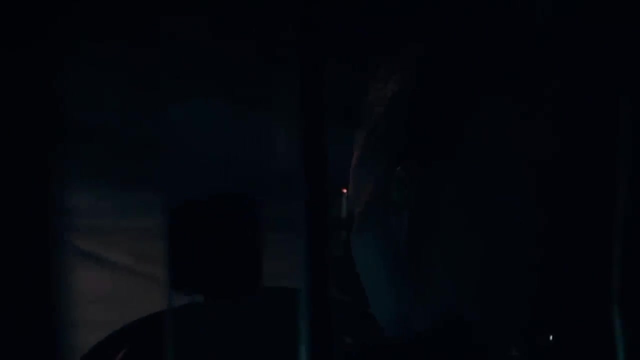 must you become? I wouldn't say it gets easier. I think you just you learn to deal with it. I suppose there's a certain point of you where you sort of switch off and you do what you've got to do. There's still jobs that I remember, that I've been to, that I won't ever forget them. 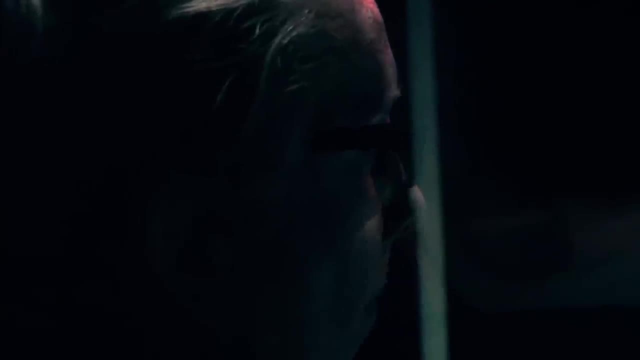 Yeah, but then isn't your brain going to be filled up with all these things, so you're going to put them to the back of your mind, don't you? Yeah, but in ten years time you're going to have this massive amount of time and you're. 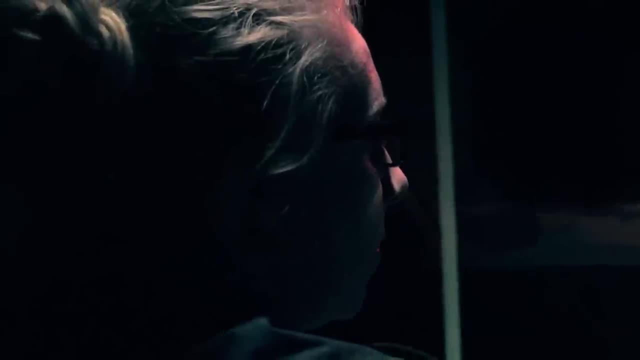 going to have to deal with a lot of things? Yeah, but then isn't your brain going to be a massive collection of things in your brain? Yeah, but you're human. you're going to remember it, aren't you? Yeah, but then what happens with a massive collection of things? 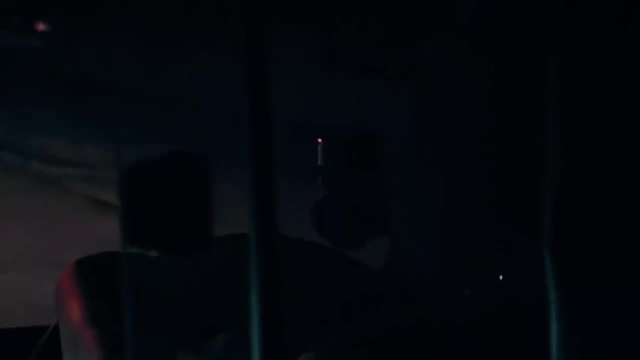 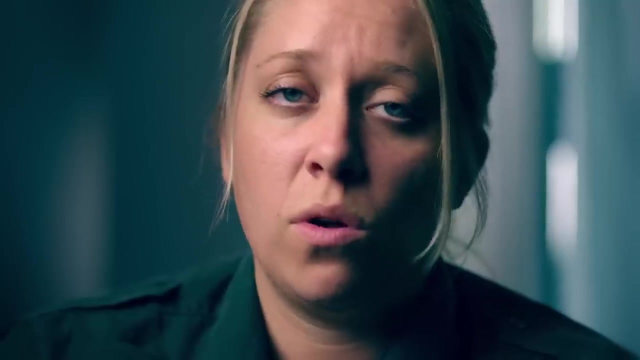 Well, I don't know, They go in the bin. Yeah, I think you've got to understand that, that horrible things do happen. You've got to put it to the back of your mind and move on. If you don't, what's going to happen to you? 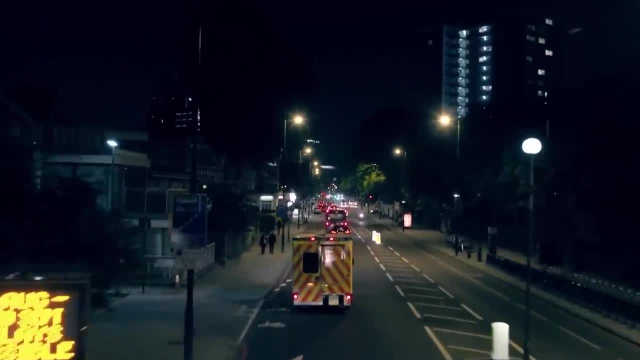 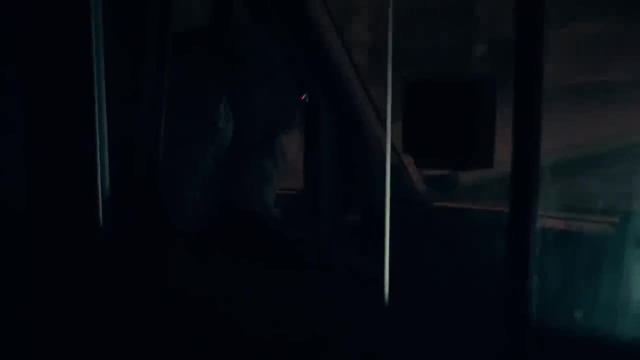 if you don't just get on with it. Oh, there's a dead cat Shat in the road, A black and white one. It was probably a badger mate. No, it was a cat. I thought you were supposed to report it if you run over someone's cat. 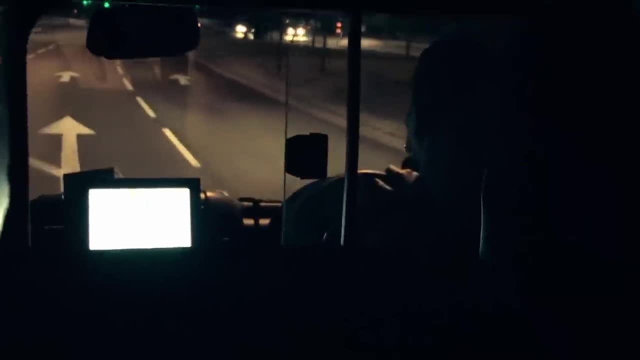 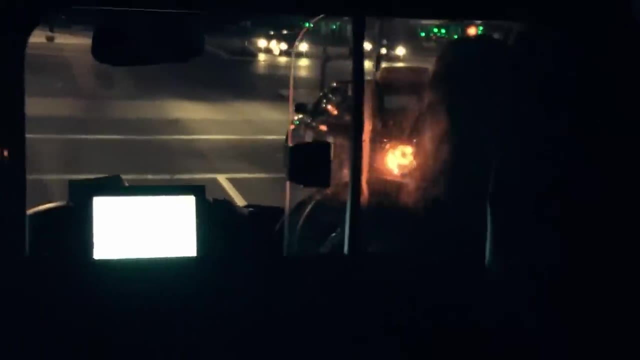 No, I knew a dog. Oh, I was late for work once because I ran over someone's cat- Apparently it was deaf- And it went across the road. If you think about it, I'm driving now a deaf cat walks across. 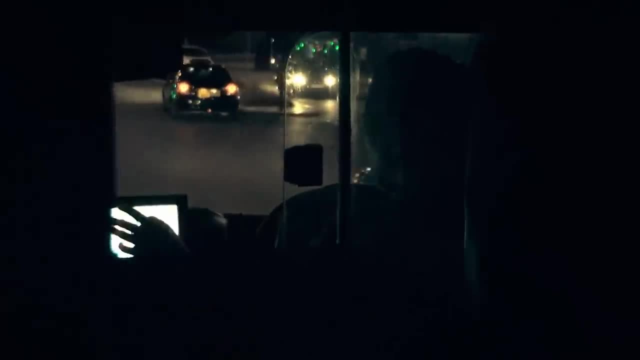 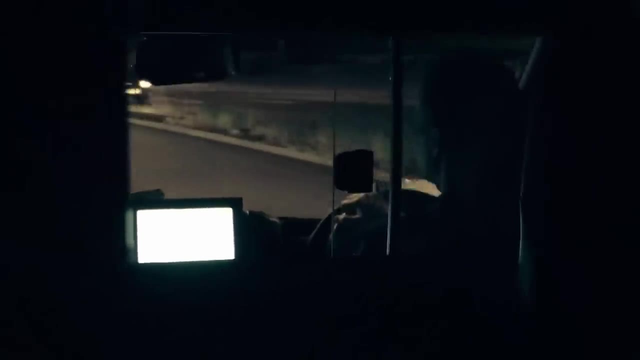 How will I know it's deaf? I don't know. The vet told me it was deaf, Yeah, but OK, yeah, I'm inventing something here: A little stripe on its tail, like on a stick, A little orange fluorescent band. 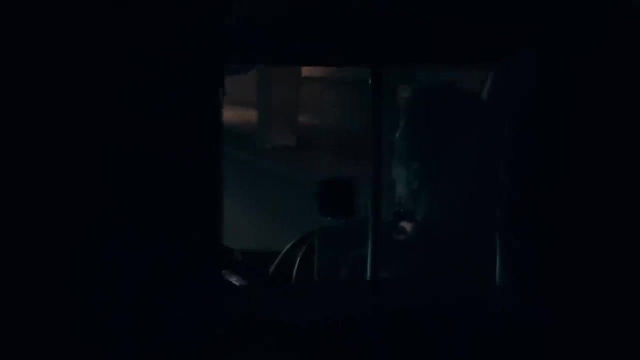 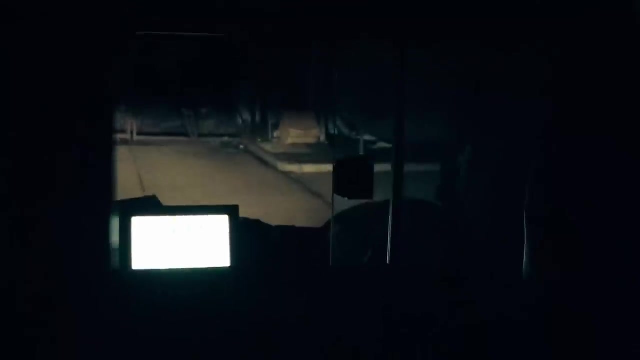 What to say? that this cat is deaf, Deaf And then an orange and yellow one. if it's deaf and blind, Shut up, as if that's not a good idea. Don't broadcast that, because I might take that to Dragon's Den. 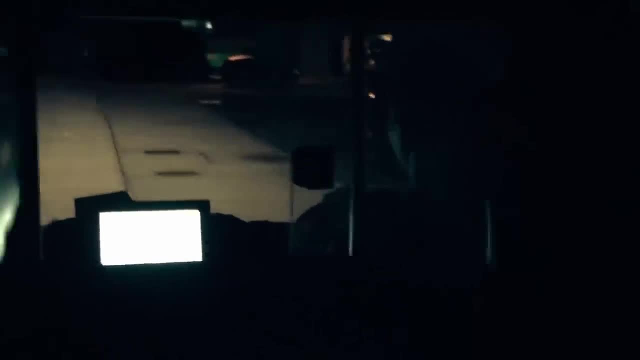 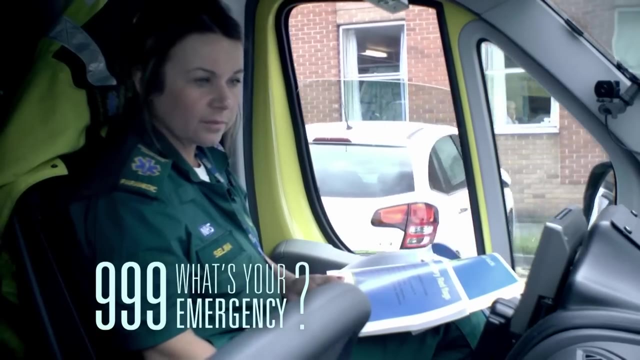 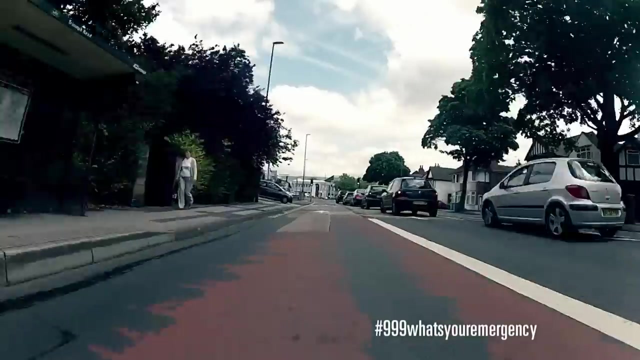 Fucking brilliant that is. That is quite a good idea. Yeah, thank you, Thank you. Collapsed making funny noises. Uh-oh, Fucking hell. Ambulance, tell me exactly what's happened. Er, this man's literally collapsed on the floor. 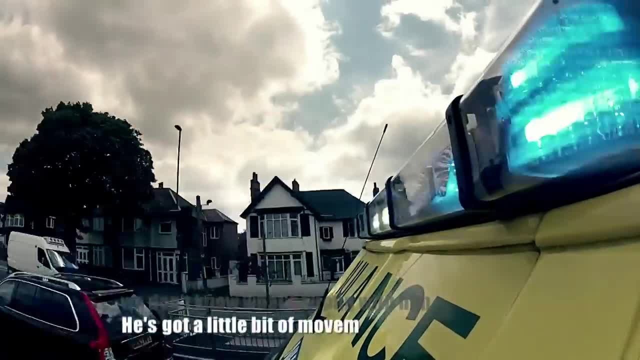 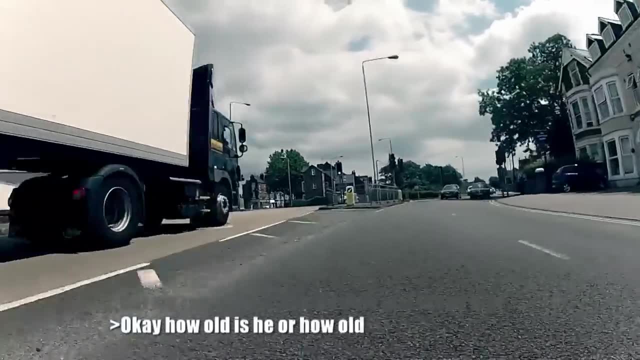 We don't know what's wrong with him. He's got a little bit of movement and he's like making weird noises. I think he's had a heart attack, but we're not sure because we've only just found him. OK, how old is he? or how old does he look? 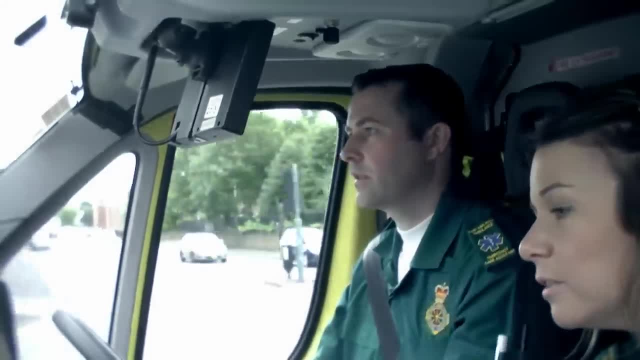 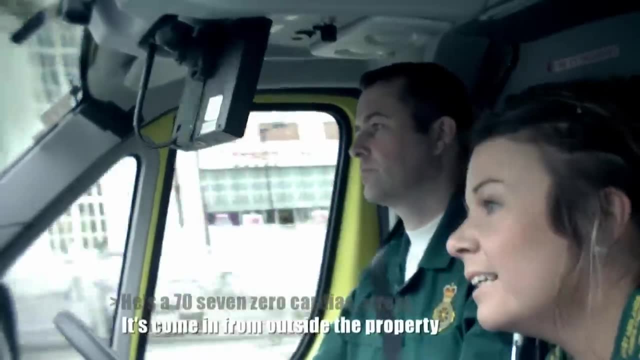 He's around about 70. Yes, 3-3-2-1,, go ahead. This is a 70-70 cardiac arrest. He's coming outside the block, please. Yep, we see I've got a feeling he might be. 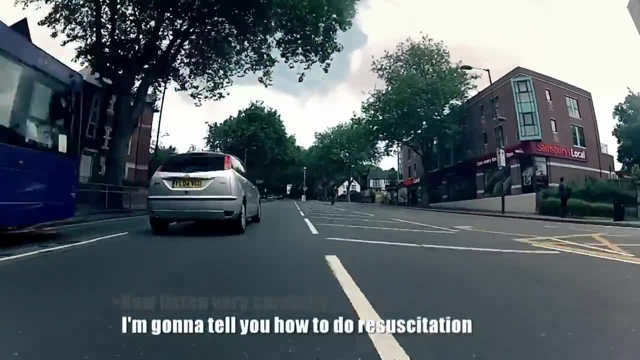 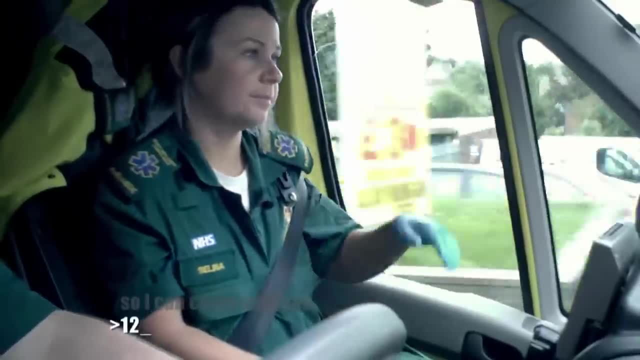 Now listen carefully. I'm going to tell you how to do resuscitation, Right? OK, Let the chest come up all the way between the pumps and count out loud so I can count with you One, two, three, four, five. 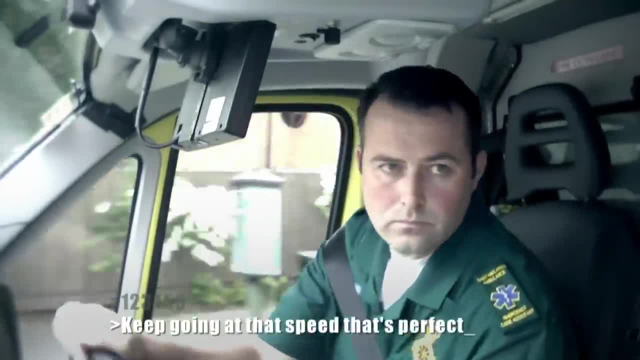 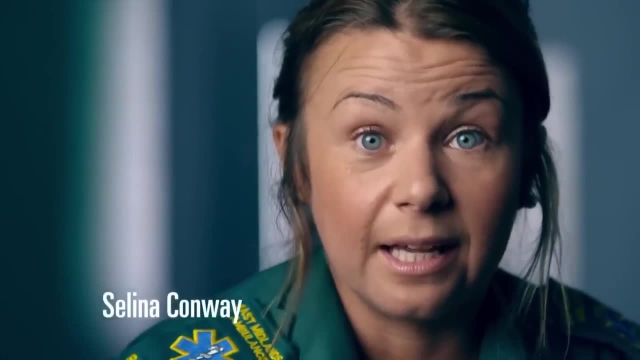 That's perfect. Keep going at that speed. That's perfect. Six, nine, ten, 11,, 12.. Cardiac arrest is probably the worst job there is to get. We only have four minutes until the brain starts to die. 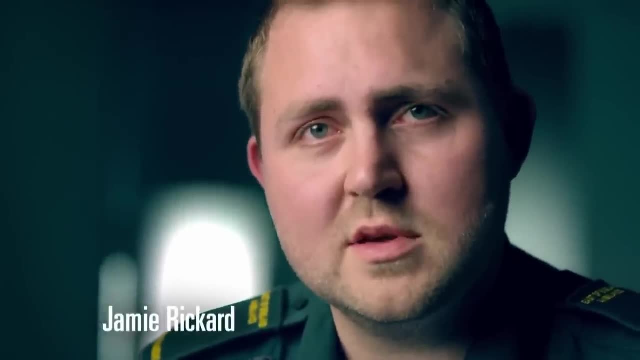 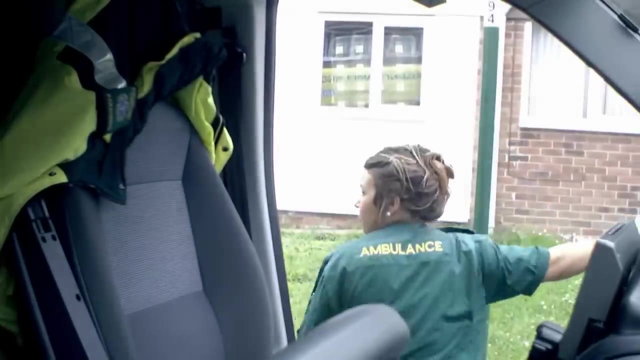 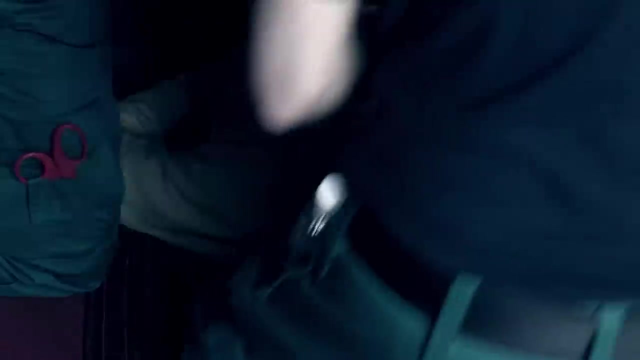 There's not many times where you could say that every second counts, but in a cardiac arrest, every second really counts. Grab the green bag. Where is he Inside? He's getting away. Did you guys just bring him in, did you? 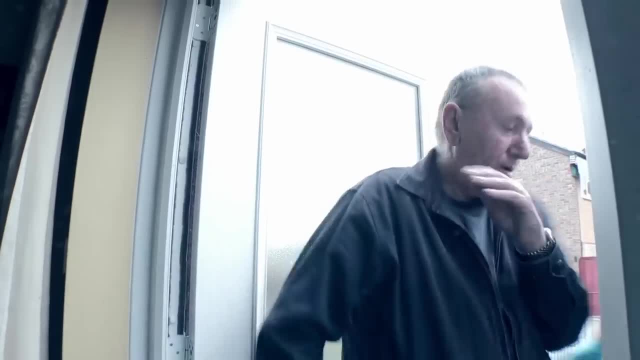 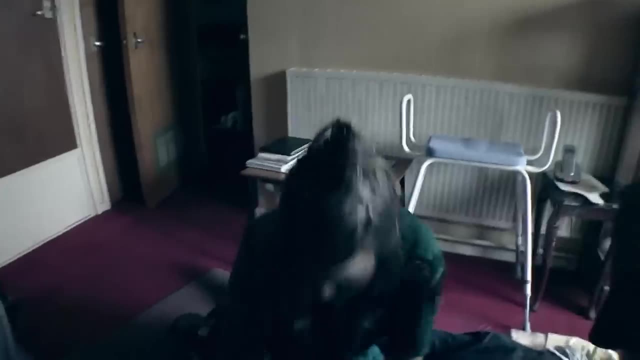 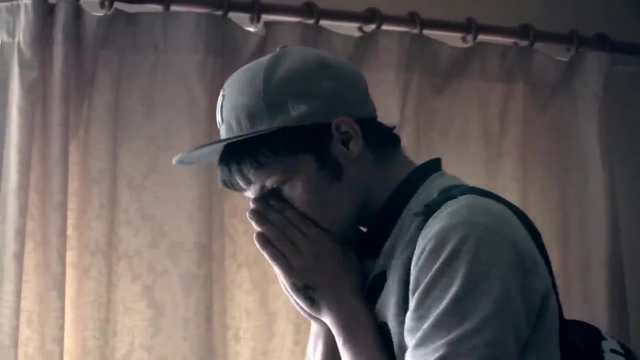 We picked him up and moved him in from the form bush, So nobody knows him, do we No? OK, I'm going to do CPR, I'll sort out the leafy. OK, Give me that. Analysing now. 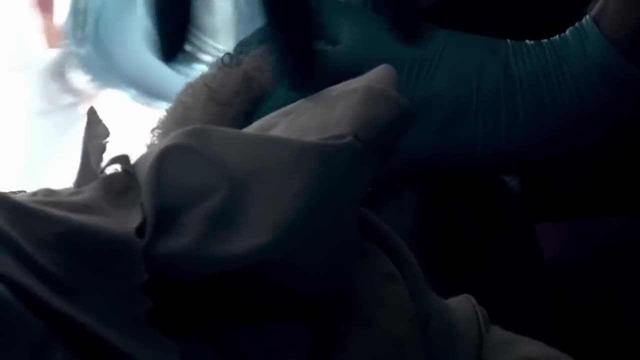 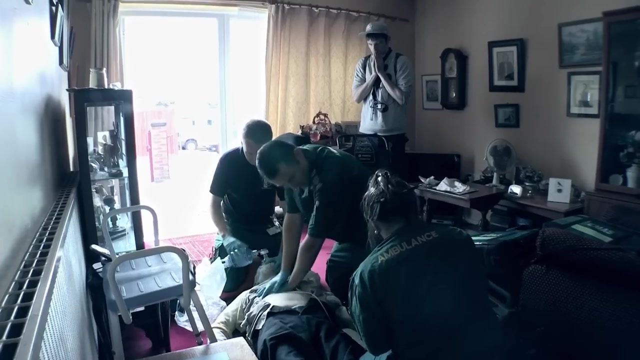 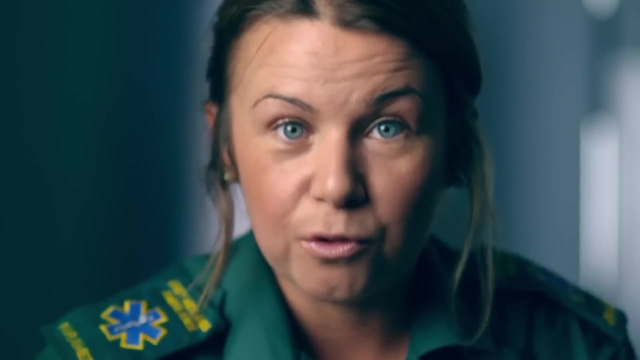 Stand clear. No shock advised. Carry on. Check for pulse, Check for pulse Armour, please. No Carry on then. It's violent. I've broken people's ribs before. You have to be really, really forceful with your compressions. 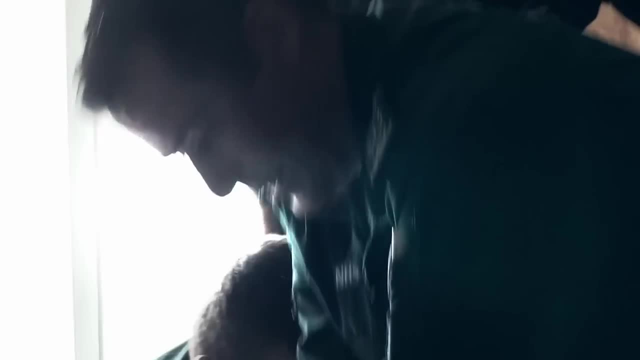 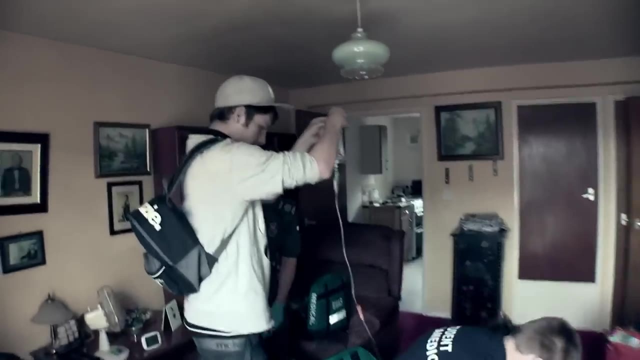 because you are beating a heart. You're attempting to keep that person alive. Lad, just hold that for me. Hold it up in the air. that's it. Are you all right, fella, Are you all right? Yeah, Bit of shock. 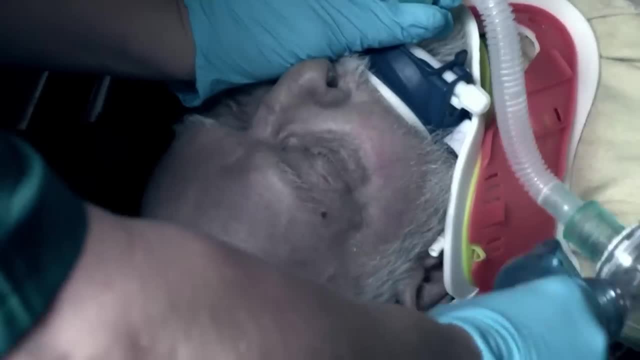 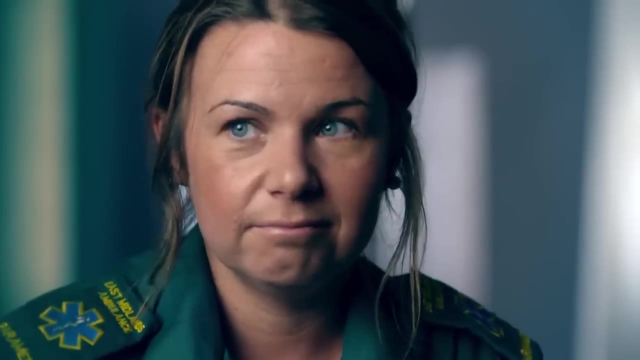 You're doing. really, really. You did the best thing you could. all right, Everything else can be treated, you know, Broken ribs will heal, A punctured lung will heal, But if you're dead, you're dead. Come on then. 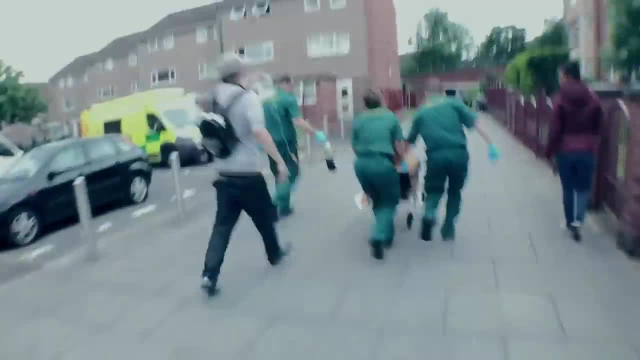 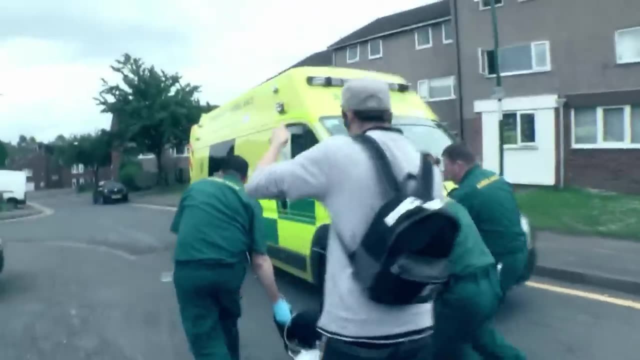 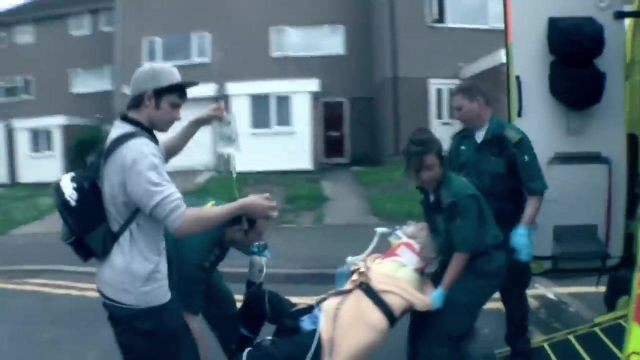 There we go right, Go, go, go. Until I did this job, death was just death. There was nothing explained in it, and I don't think you become aware of what death is until you see it, Until you see it yourself. 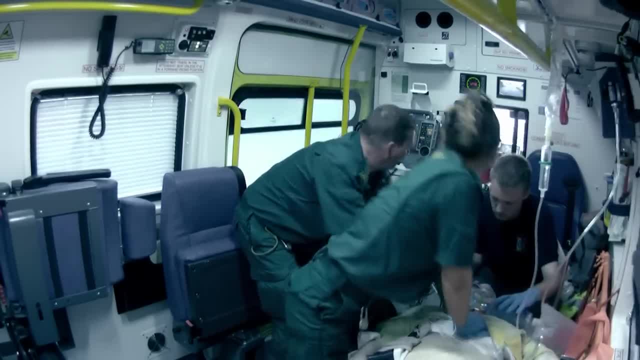 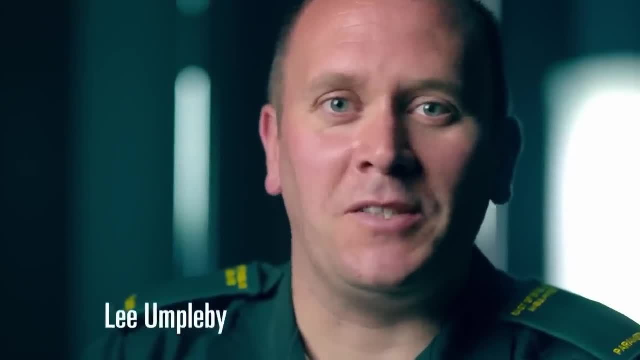 It's not all drama. It's not all arms being thrown. There is no. this is how death will be. There is no manual to the correct way to die, And nobody. Until you see that, I don't think anybody is aware of that. 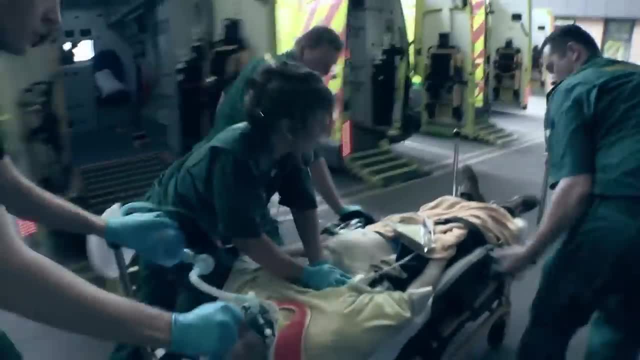 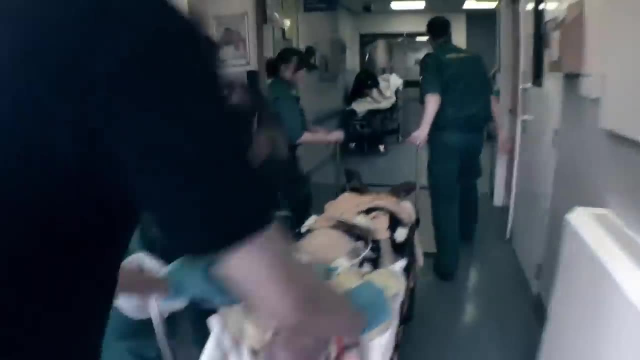 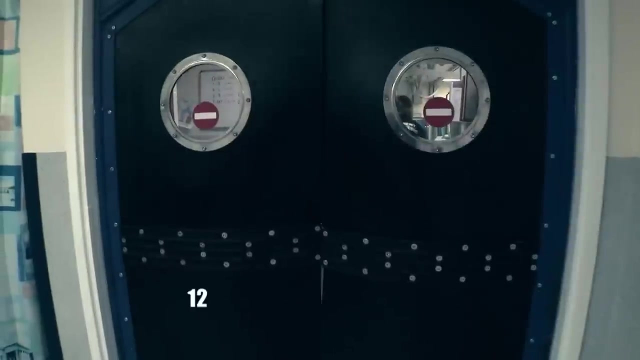 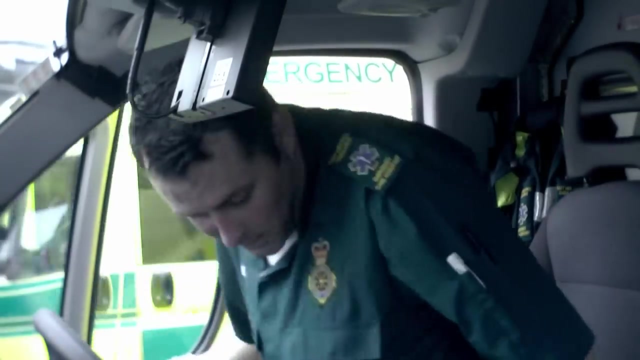 Definitely no way, You don't. you're doing this really to yourself, I think. No, no, no, I don't really know how to go about it myself. I haven't written anything, I haven't himself. The tough jobs, the hard jobs. you know they're draining. 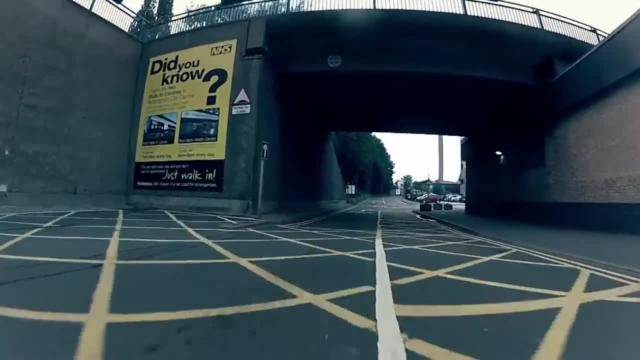 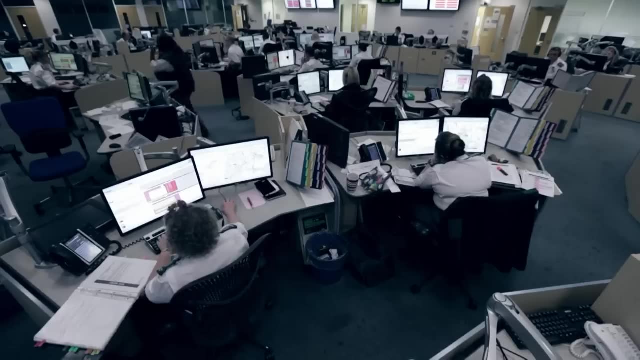 And you don't really think about the severity of the job you're in until afterwards. That's when you're like: could I have done this better, could I have done that better? You know you critique yourself a little bit. Ambulance: tell me exactly what's happened. 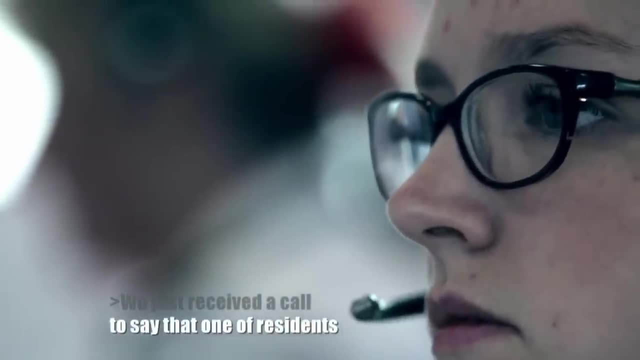 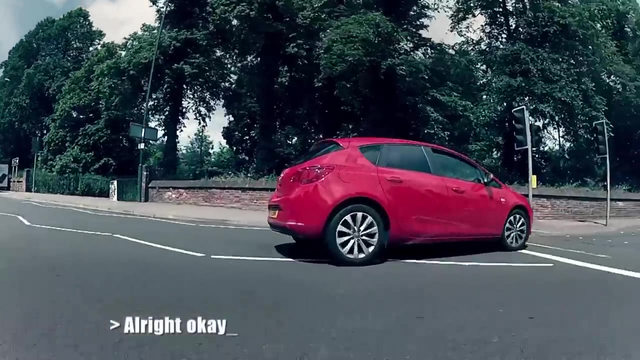 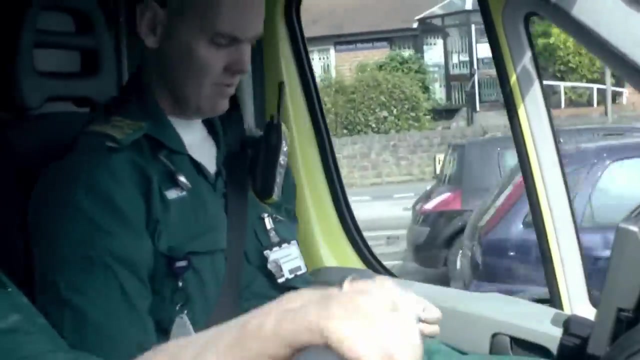 We just received a call saying that one of the residents has died. you see, OK, how old is the patient: 16 years of age. All right, OK, In the UK, one person dies every minute. That's over 1,500 a day. 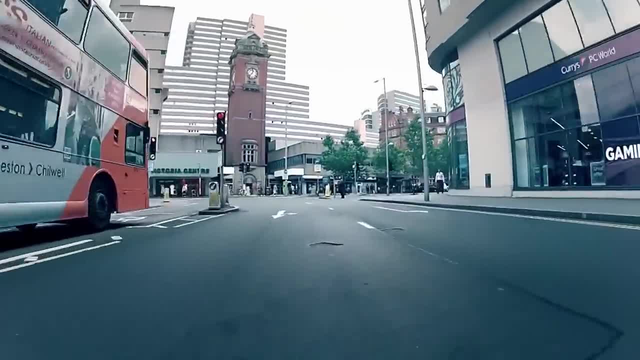 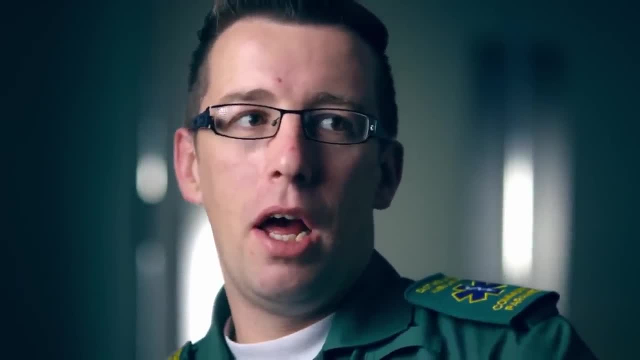 It's strange. I know they say in the films that you watch somebody, you know they all pass away and it's really dramatic and you know they roll their head back to one side and then open their mouth, etc. You don't get that, but you do get the sense of. 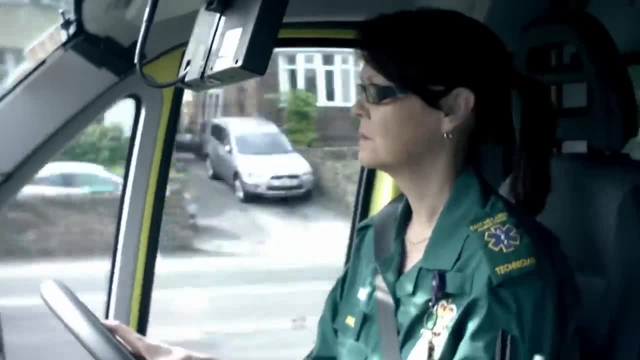 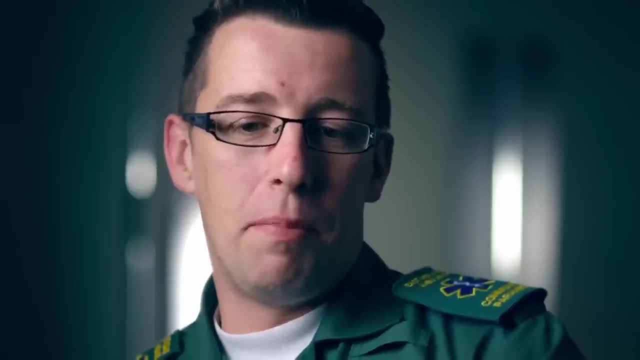 I don't know the sense of somebody's not there. I can't explain it. I really can't explain it to you. You have to see it. I wouldn't say I'm a believer in God. I wouldn't say I'm an atheist. 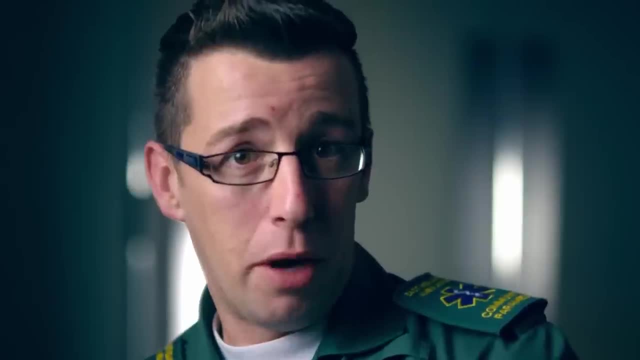 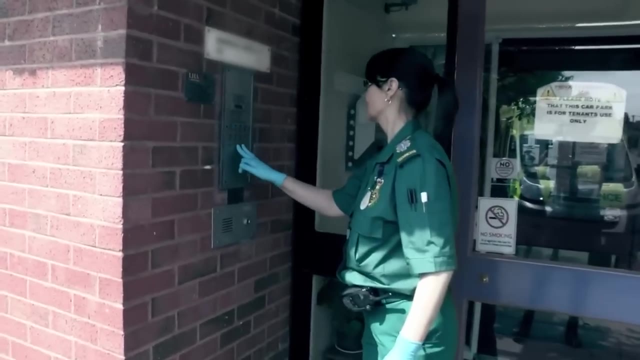 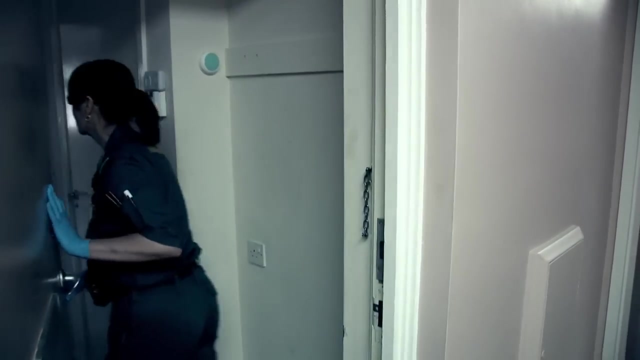 but I believe that something is there and something goes Where it goes. I don't know. There's certain jobs that you'll see death and you just couldn't possibly even imagine what had happened. I went to a job once. it was absolutely horrendous. 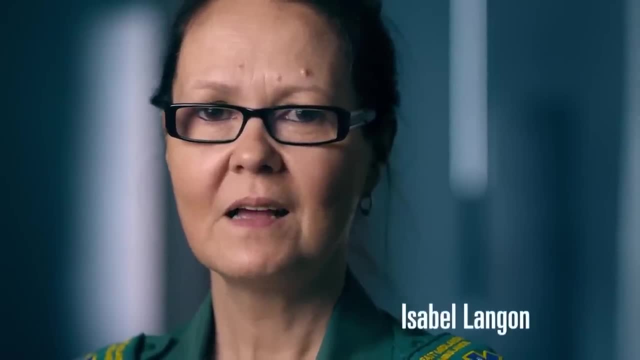 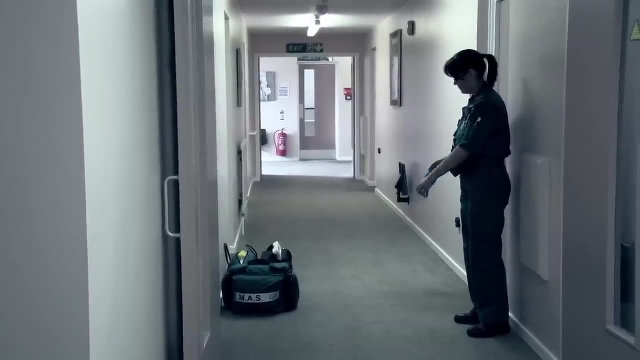 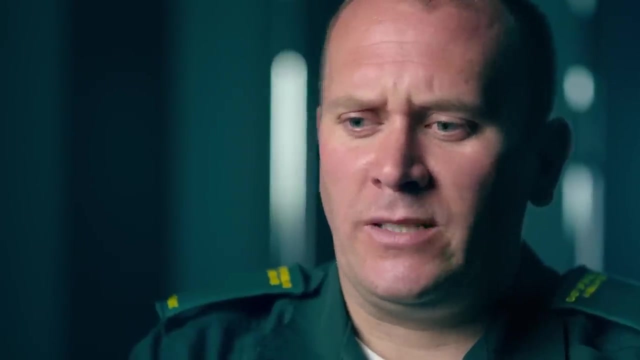 This poor gentleman had literally coughed up his lungs. It looked like somebody had opened a couple of tins of tomatoes and just thrown them around the room. A patient that I've been to had been dead for three months and the body had basically decomposed into the carpet body fluids. 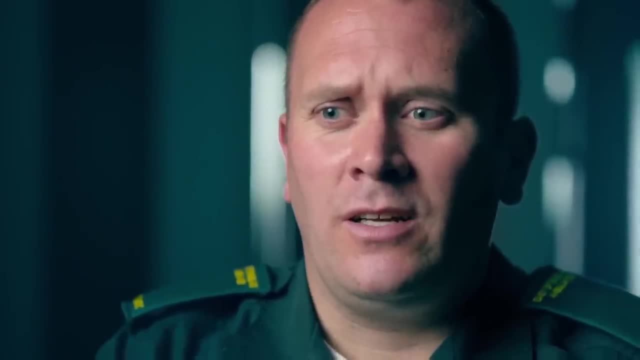 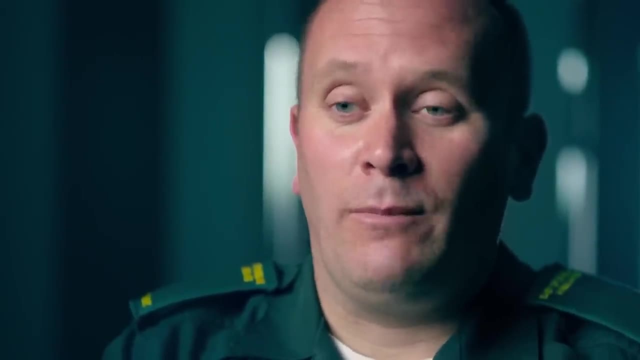 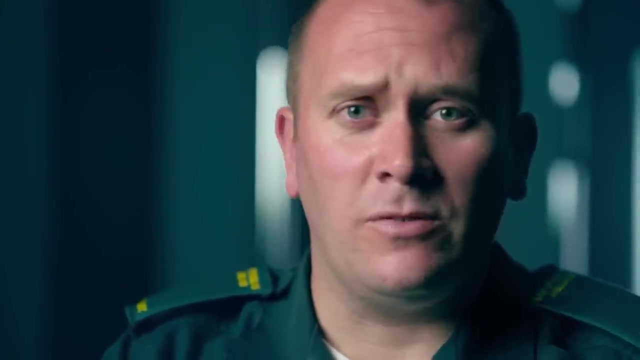 When the police smashed the door down to get into the house, the smell hit the police officer literally. You saw the police officer jump back and my colleague who nearly vomited because they weren't prepared for that smell. The smell is just phenomenal. 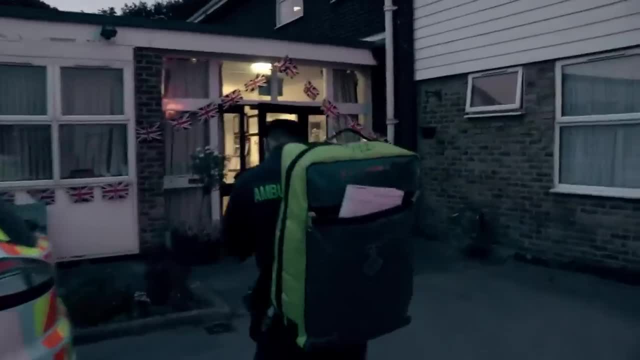 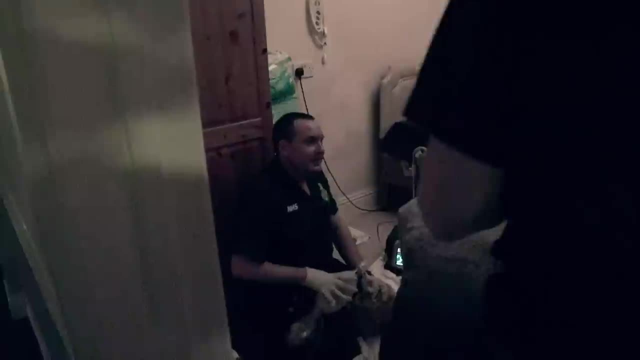 I'm taking a grab bag in case I run out of oxygen. It's 4.30 am and Dil Patel has been called to a care home where paramedics are with an elderly resident. We've got a 90-year-old- 90-year-old on the acting rest. 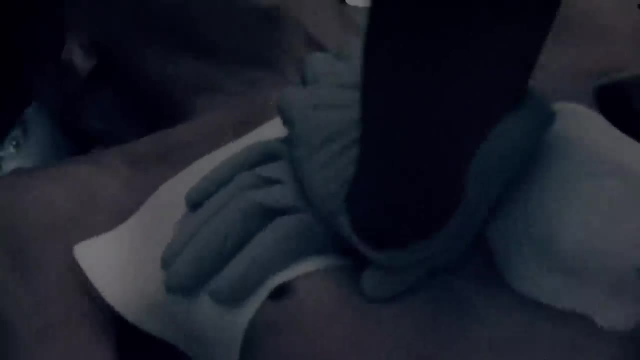 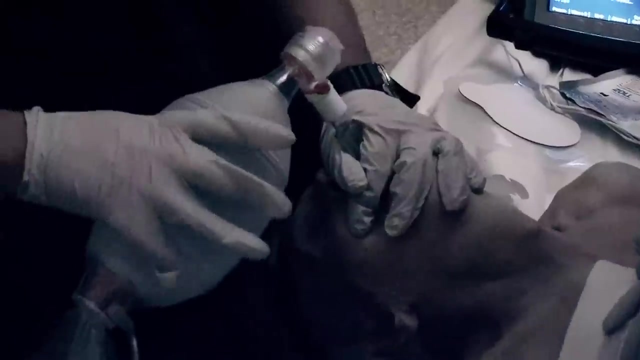 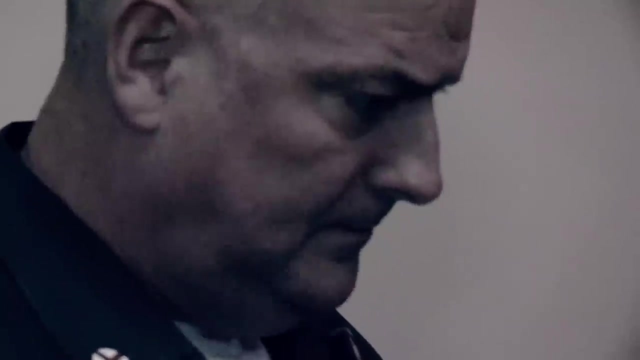 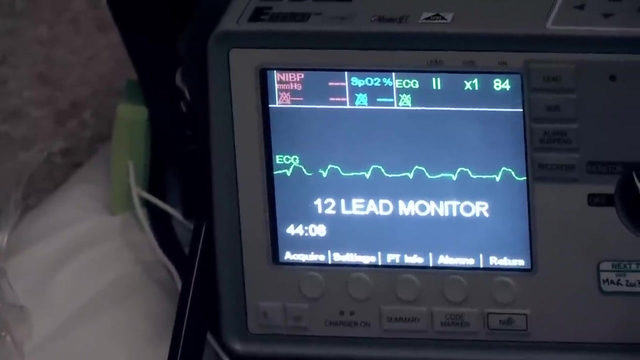 Thank you. We're not reacting, are we? Thank you. Is that adrenaline? Yes, Is that so? Thank you. The first paramedics on scene began CPR 45 minutes ago. Just come off a minute. Yeah, I've got a pulse. 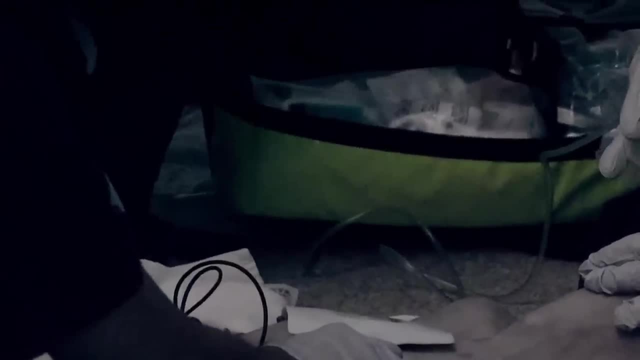 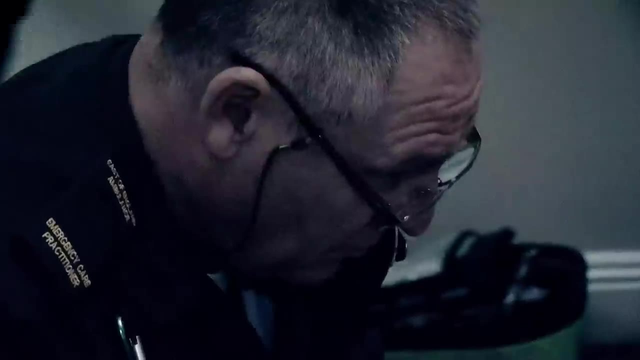 He's making respiratory effort there. I was just watching there as well. He's starting to make respiratory effort. You've done CPR and they're hard to believe. The heart is working now, but they're not necessarily alive, are they? 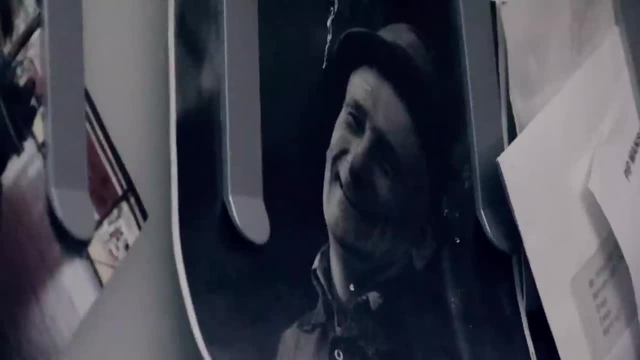 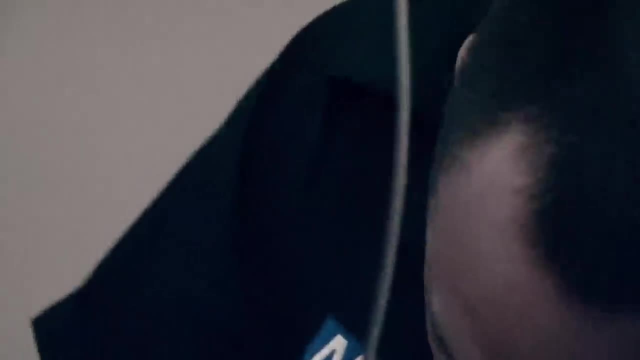 Their heart and lungs might be working, but is there a person there That's getting fainter now? Yeah, Yeah, We're losing that. I'm sorry, I can't feel it. It's gone. We'll start CPR again. 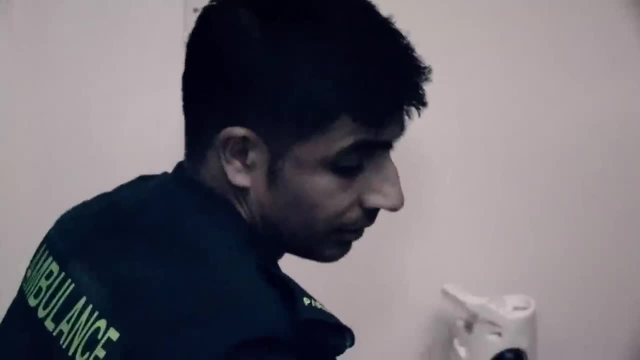 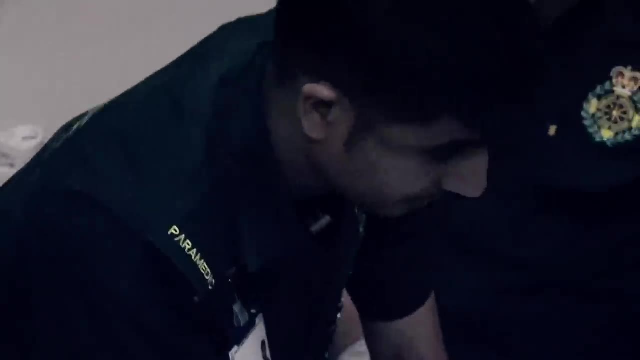 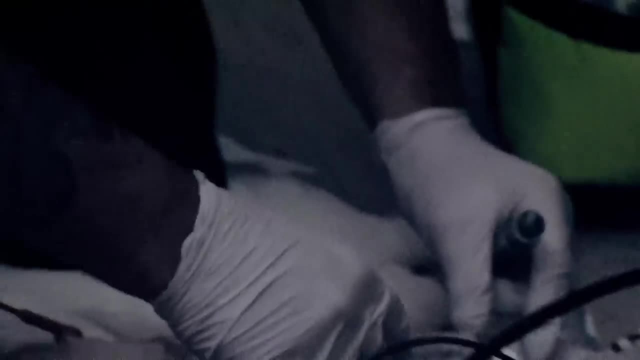 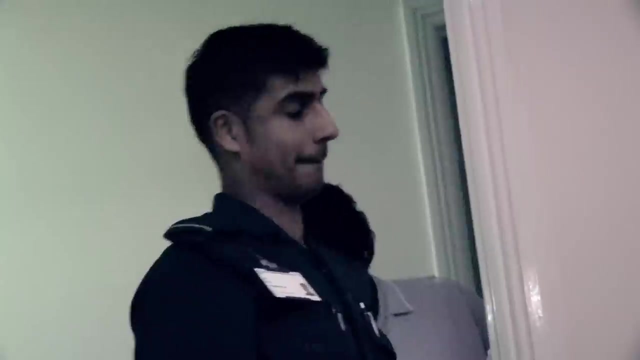 It's a fraction of the efficiency. Another adrenaline as well, Mick. So when you do it for that length of time, it's just not conducive to life. A decision will have to be made. Yeah, let's get clinical advice, because otherwise we're just 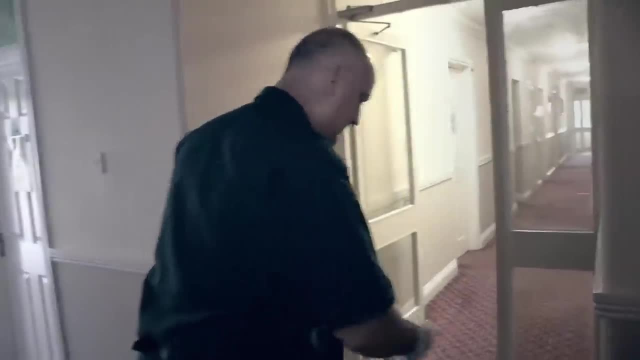 Is that my judgment call, then? to do that? I'm happy to do it. I'm happy to do that. I would have done it a while ago if I was here earlier, but I wasn't, so, Or something, Okay. 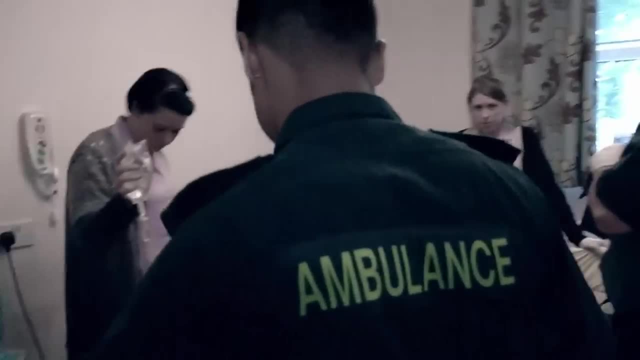 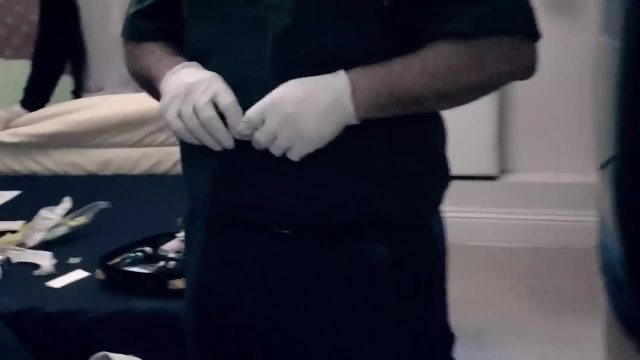 Okay. so if he loses it now, it becomes our decision whether it's ethical to continue. He's lost it. I personally don't think it's ethical to continue. Will you all agree with him? Yeah, Yeah, I'm giving him the best chance possible. 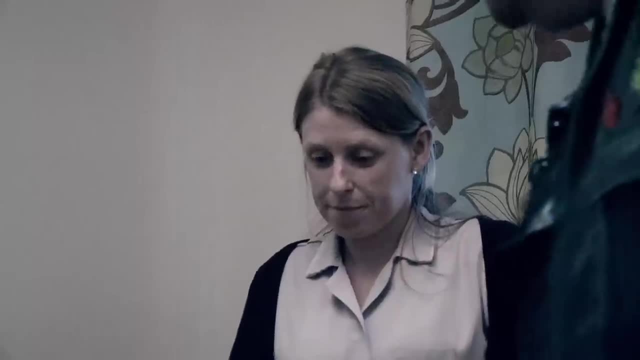 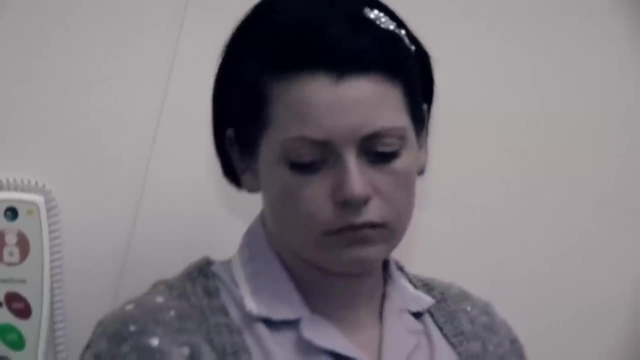 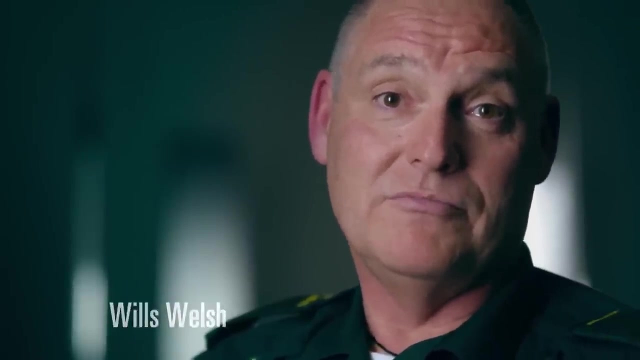 Yeah, Yeah, Okay, Okay. It's very difficult when you've got to that point and nothing's going to happen going to revive them. You've given them the drugs, you've done the CPR, you've given shocks if it was necessary, if they were able to take the shocks, and nothing's going to. 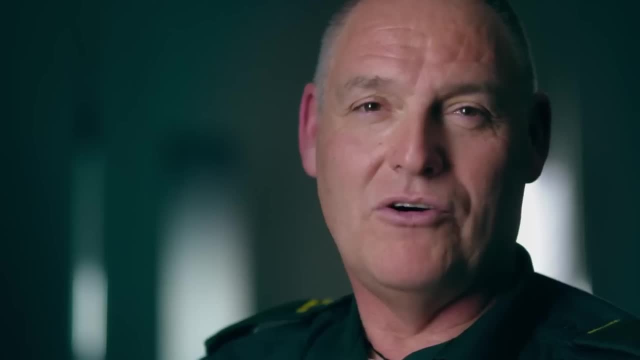 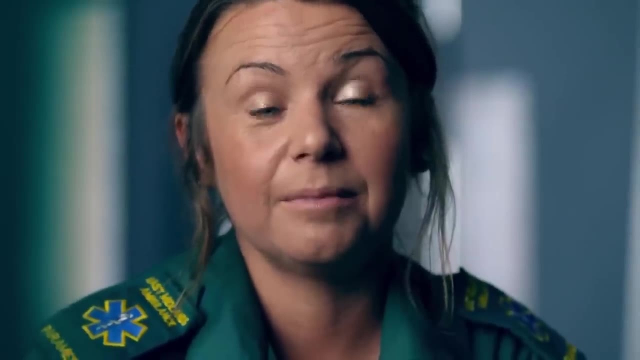 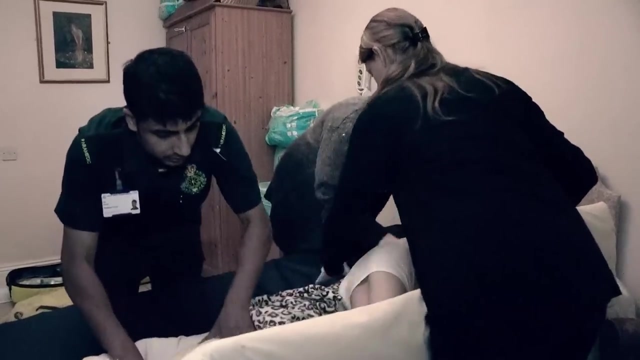 bring them back. It is hard, I know. if it was me, I would prefer to pass away in my sleep and not have an ambulance crew jumping up and down on my chest for 20 minutes To actually intervene with a cardiac arrest, even though occasionally there's a good outcome. 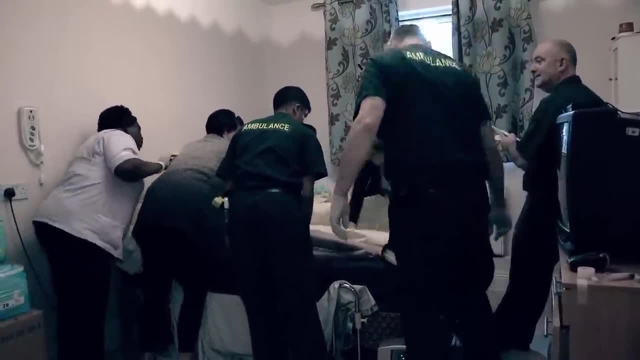 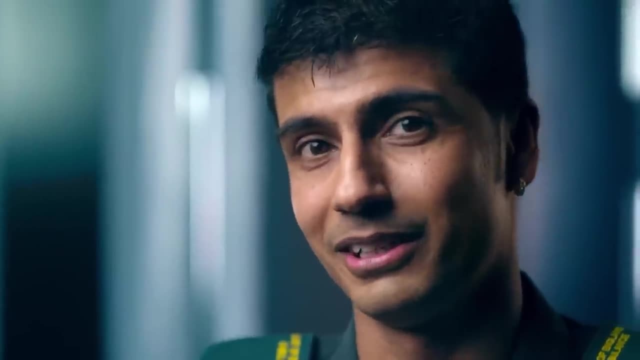 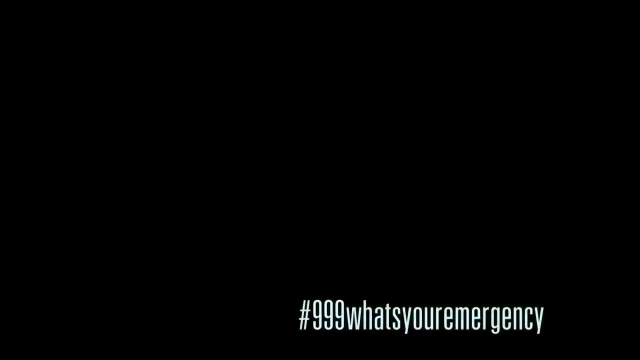 I think that's the ultimate interference, if you like, with nature. I think it's an unnatural process and you know, death is as natural as living. As sure as you're alive, you'll die. You're alive, You're alive. 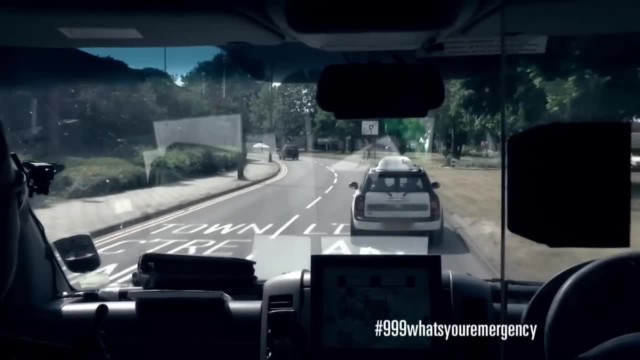 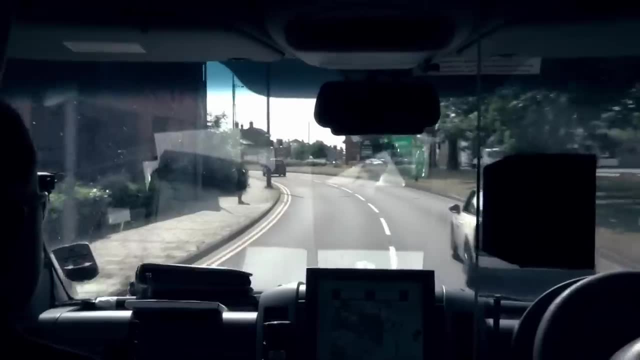 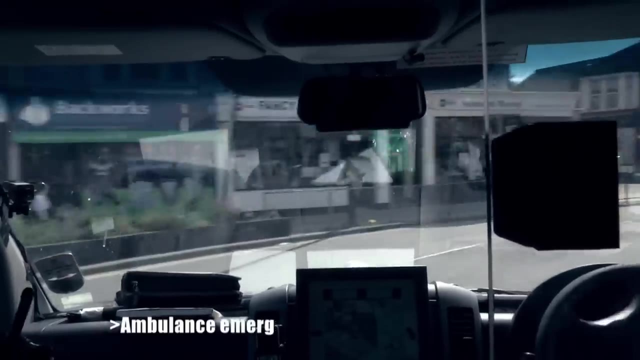 You're alive. You're in the car. tell him to pull left. You can't tell him to do that. Idiots, aren't they? What a fucking driving instructor. Ambulance emergency. tell me exactly what happened. Well, I have a district nurse here. actually, I don't know if you want to speak to her. 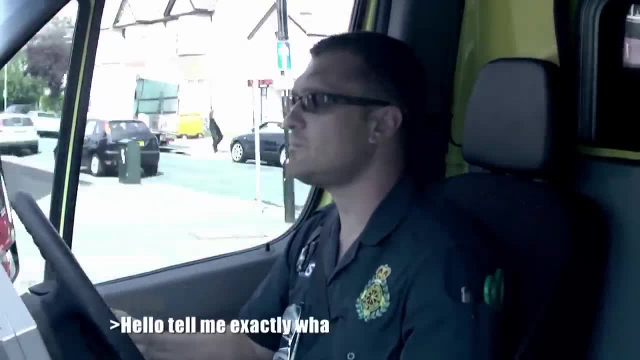 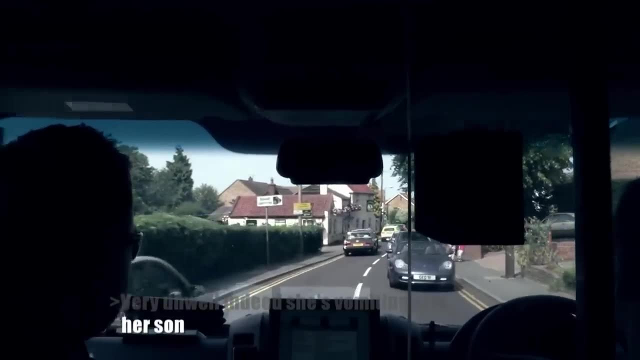 Please, she's there. yes, please, Hello, Hello, tell me exactly what's happened. She's terminally ill, Right, Very unwell indeed. She's vomiting. Her son is not able to cope, She's so horny. 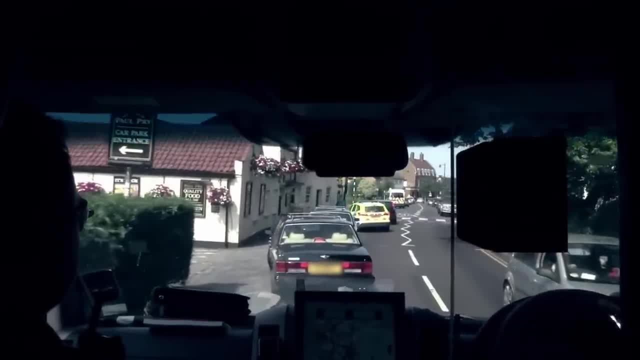 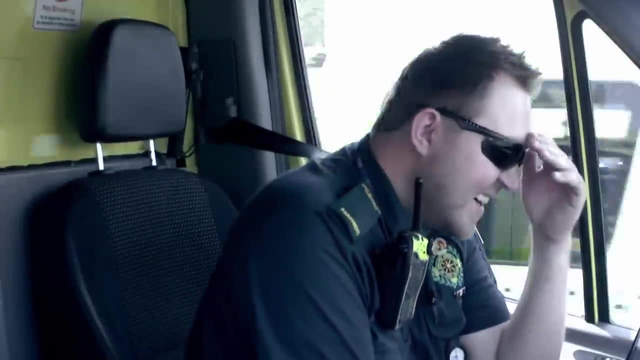 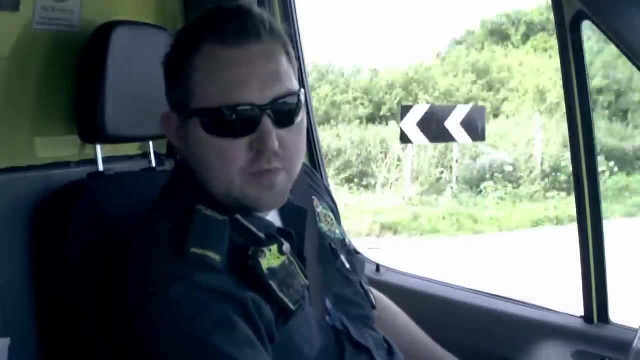 Am I Okay? That's it false of funeral cars off the road. Too late for him With mourners in it. Too late for him. There's nothing I can do about it. So it's a 90-year-old female palliative care who's got a liver blockage, jaundice and constipated. 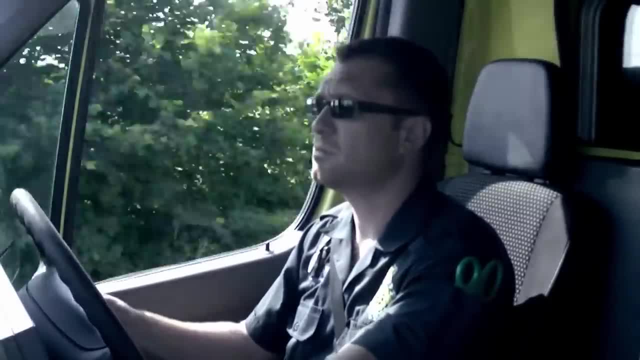 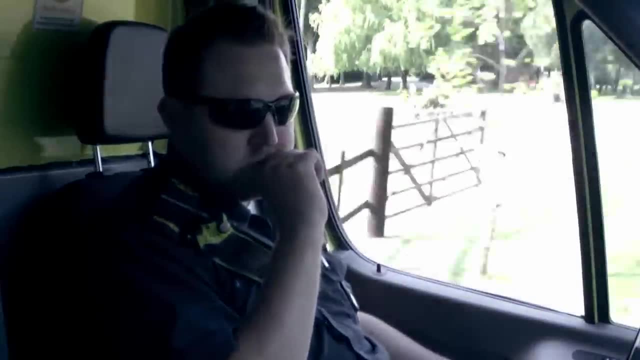 and vomiting. It's really difficult for us because we We are programmed from the minute we join the ambulance service through all our training to save lives. So the biggest thing for me, I found, was when I go into a patient who's terminally ill is. 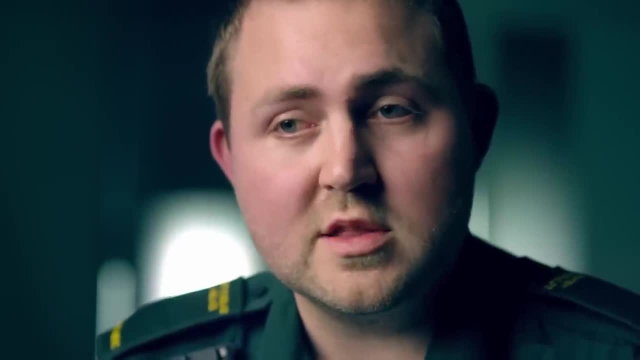 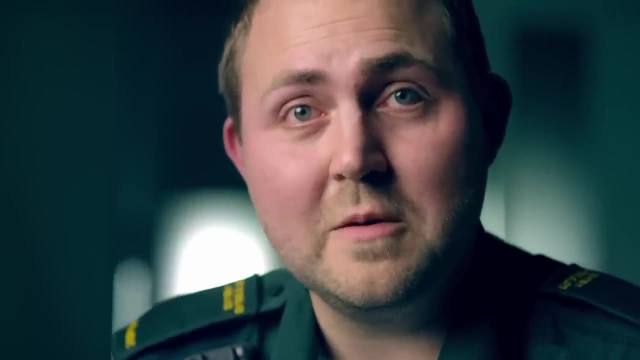 to actually think, to look at them and to think you know what they look at death's door, and then to suddenly try and get it into your head. well, of course they're at death's door, They're terminally ill. 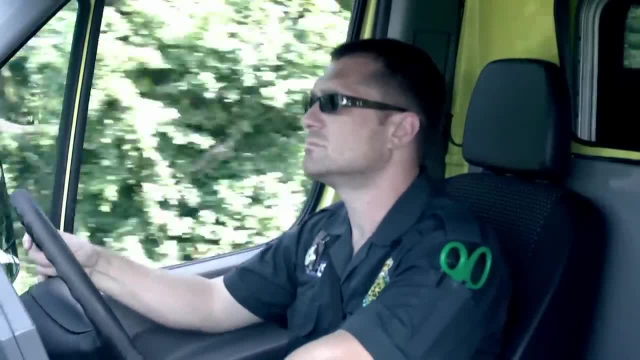 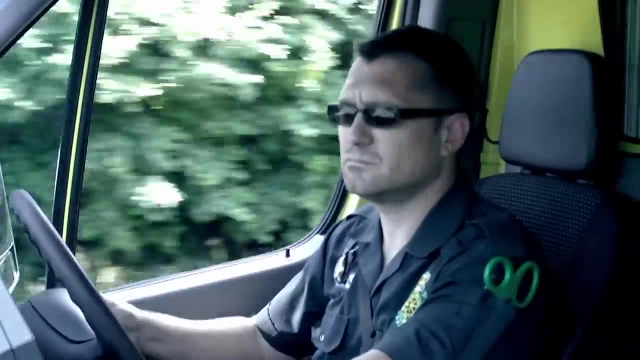 This is what's going to happen. I'm just thinking ahead about this job. Yeah, You know palliative care and all Yeah, And that this lady is probably going to die in this fashion. Yeah, Now, if the situation allows, we can subtly suggest other, maybe, forms of care. 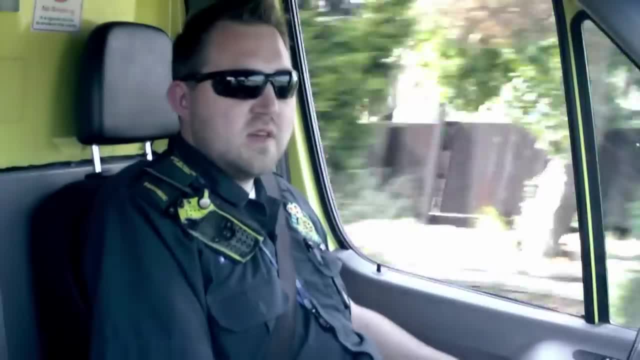 Basically doing everything in my power not to send this woman into hospital. This has all come on pretty quick. It was fine until two and a half, three weeks ago. Yeah, The jaundice has come on quick. Took her into hospital, gave her a CT scan. 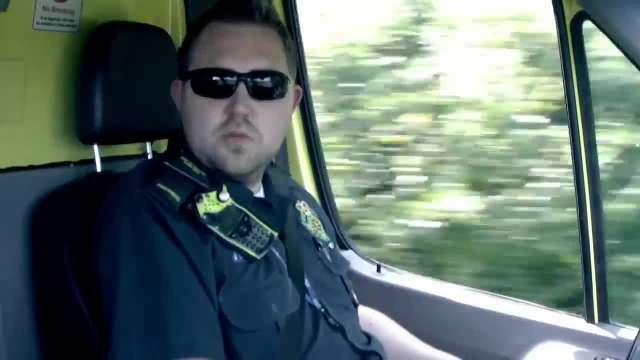 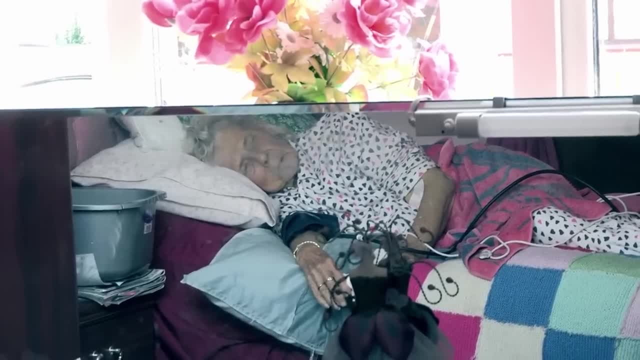 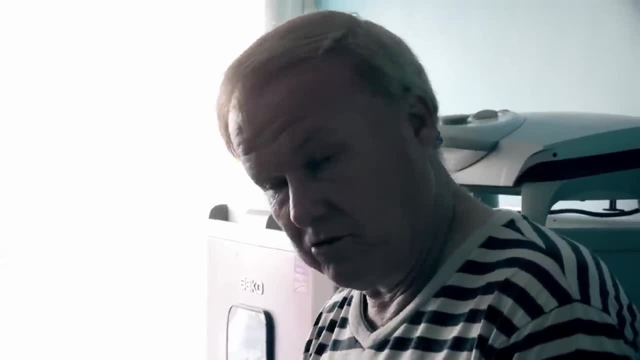 Took her into hospital, gave a CT scan- Exactly 10,. what's wrong? But I don't know. There was a little blockage just outside the liver: Mm-hmm Total blockage. Have they given a timeframe at all? 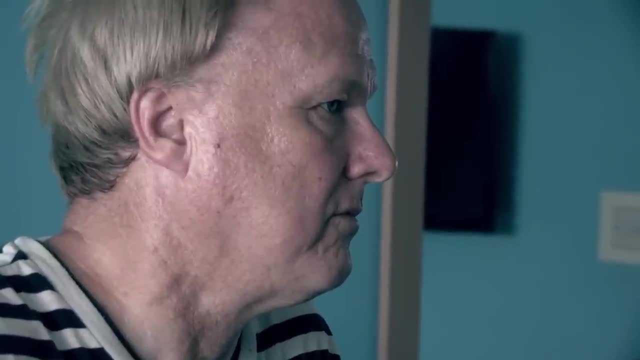 He said maybe a couple of weeks. Like, we'll see. Our concern would be that if we take her in, there's always the possibility that she may not come out of hospital, which is what I'm just thinking, trying to think just a little. 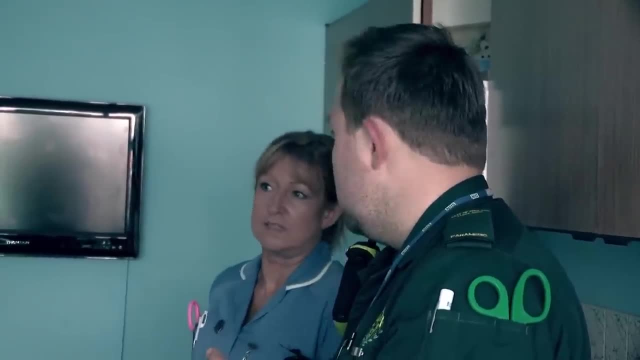 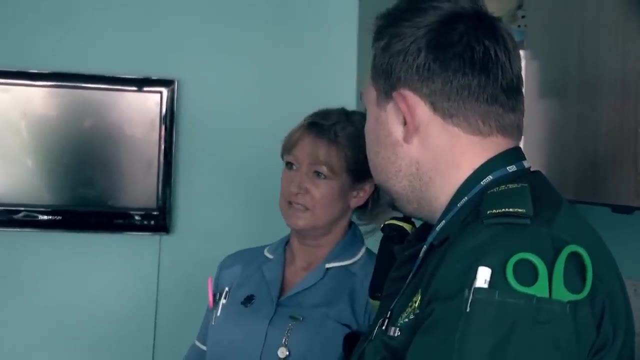 bit further ahead than the hospital. She needs to be in her right place. Well, the hospice, I think, would be the ideal. Yeah, Yeah, They're very limited on their beds. This is the problem I know. look, this is pretty terminal. 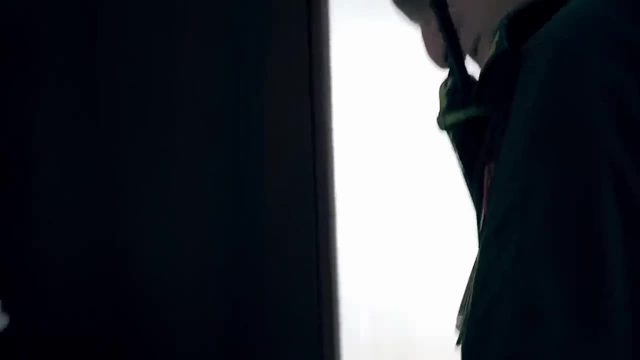 I don't mind the pain, that's the main thing. No, no, of course not. Look at me, Betty. Hello, I'm the ugly one. you have to look at me. Sorry about that. That's a bit of a smile. 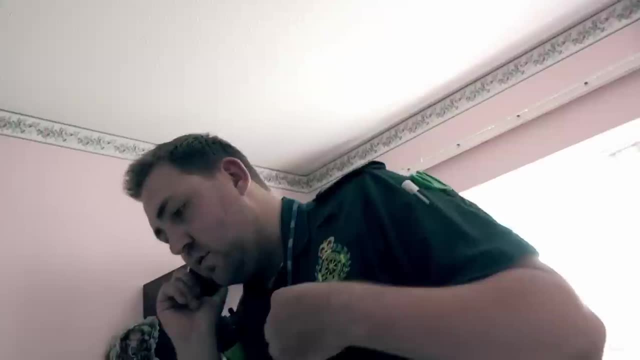 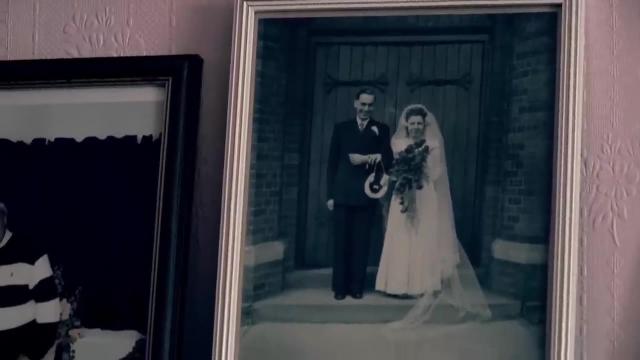 We're currently with a 94-year-old female who has a recent diagnosis of terminal CA of the liver. Is there anything that can be done with regards to the hospice Right OK Hospital is somewhere that most people don't want to be. 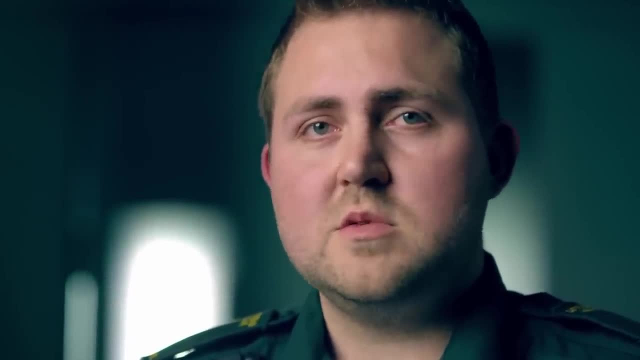 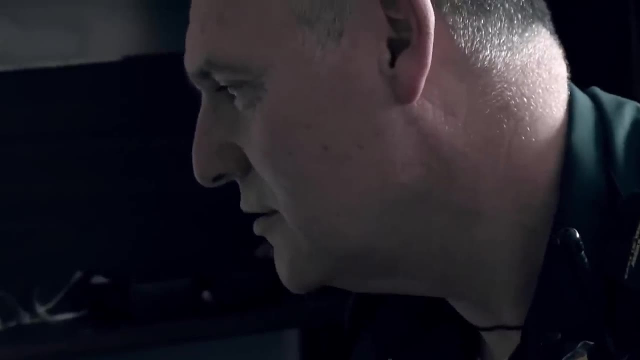 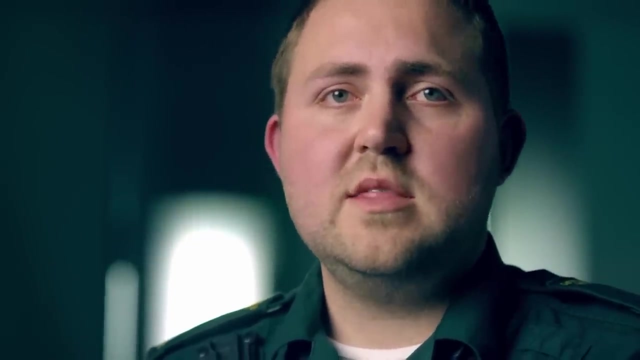 and it's certainly somewhere where most people don't want to die. I'm trying to find a proper place for you today, OK, one that can help you. It's not always possible. There are times where hospices have no beds and actually, in that case, sometimes hospital is the only place. 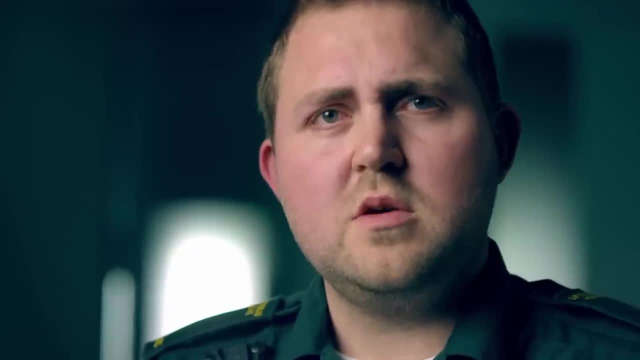 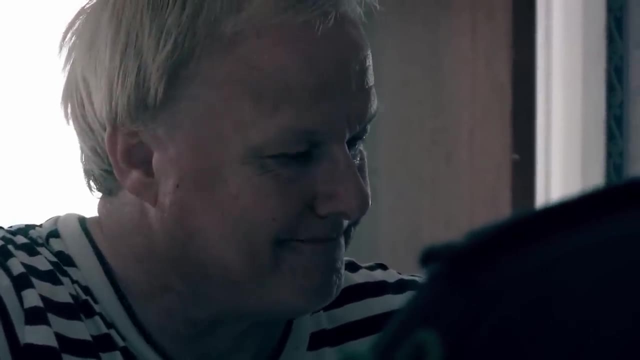 But at least you've, I think at least, as if I've tried, then I've tried. I'm happy. It's just not great. Let's go to the hospital. It appears to be: yeah, Betty, Hello, We've got a chair for you, OK. 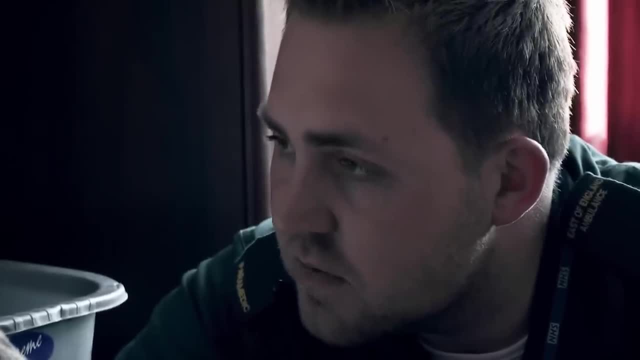 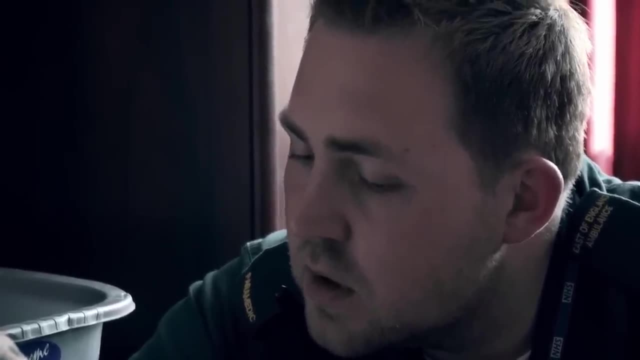 We're going to get you up from your bed. I know it's not going to be very nice or very comfortable, but we'll get you from your bed onto the chair. OK, Mm, If you need any more sort of pain relief, then we'll deal with that. 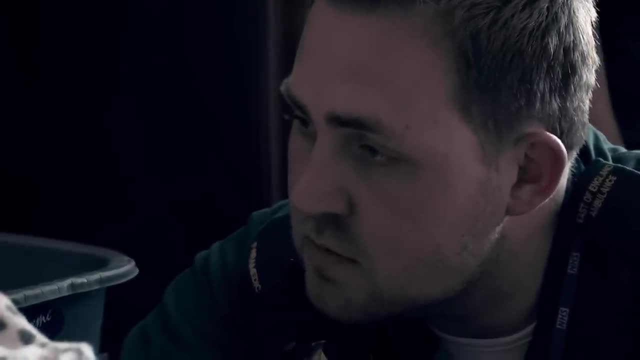 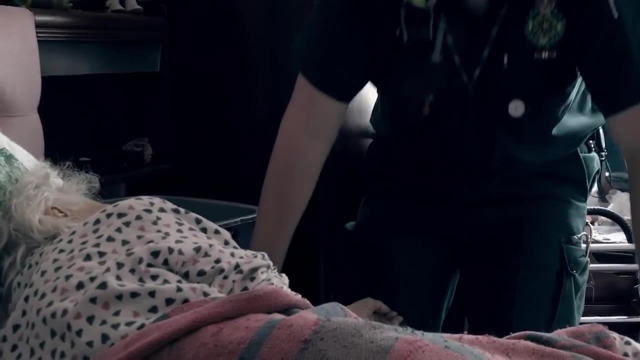 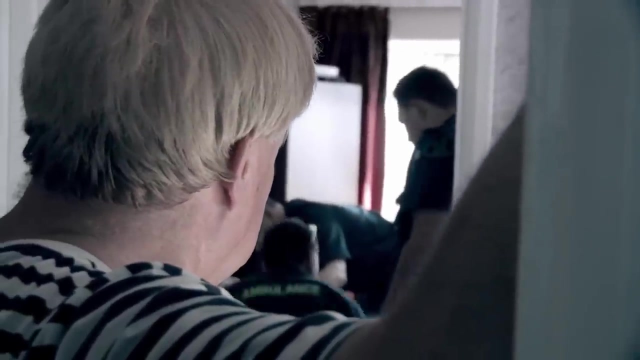 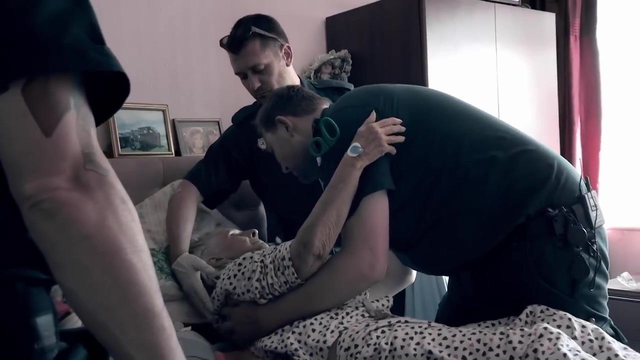 Just let us know, OK. OK, Just slowly, There we go, Betty, Betty, Betty, we're going to just sit you up. Can we give me a cuddle? There we go. This doesn't happen every day, does it? 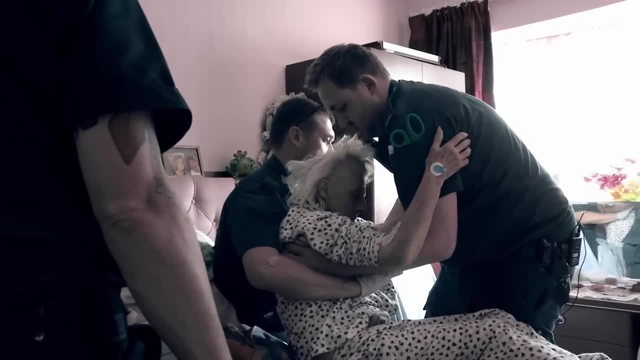 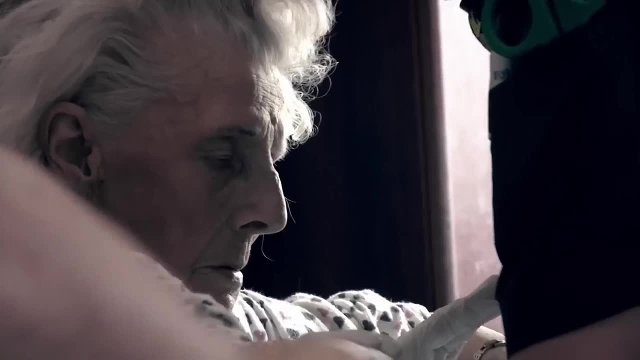 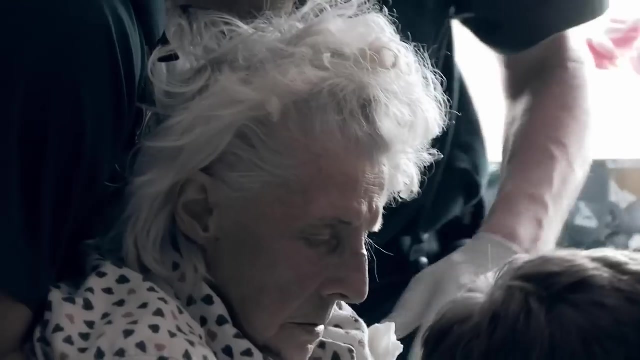 All right, OK, Can you cross your arms, Betty? That's it. Give me your hands there. There you go, One, two, three. You've got the time to spend with terminal ill patients and you can make them so much more comfortable. 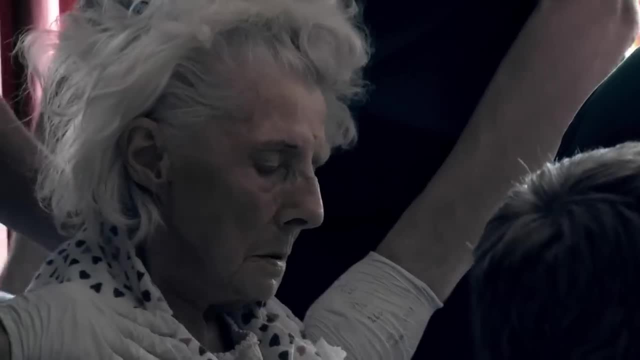 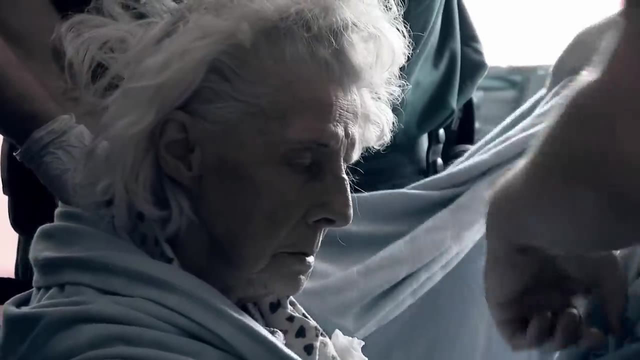 All right, You know what's an extra half an hour, sometimes a few hours out of your day, to help this person and not to take the easy route. It's probably the most important thing that we do: Birth and death. You know it's entering and exiting. 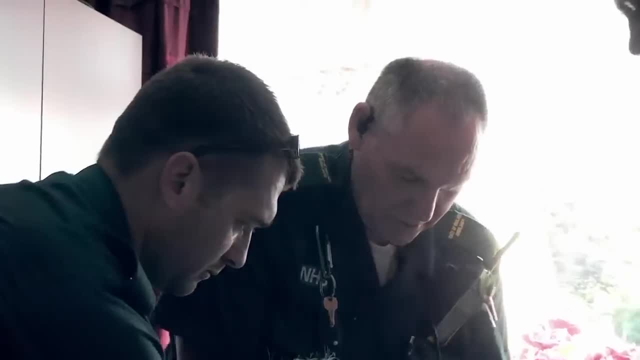 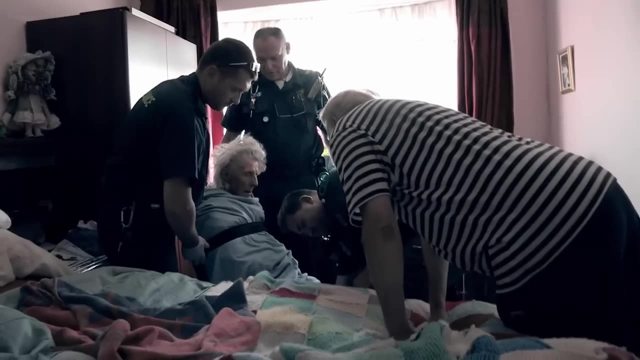 Have we got any cheer? Fair enough, You only get one chance for someone to die. You have to do that, right. Right man, I'm all with you, OK, I'm coming to the hospital with you. OK, You hear me all right. 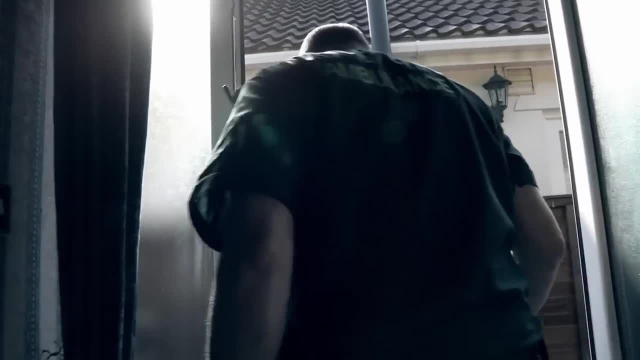 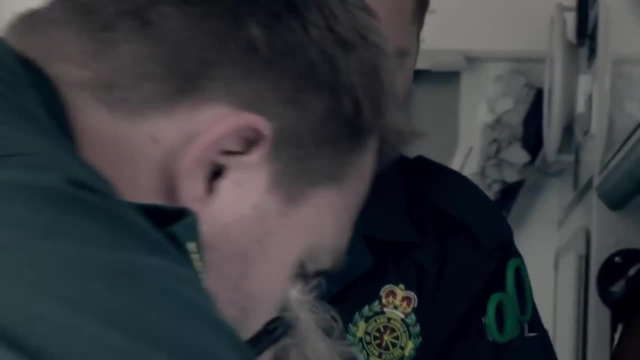 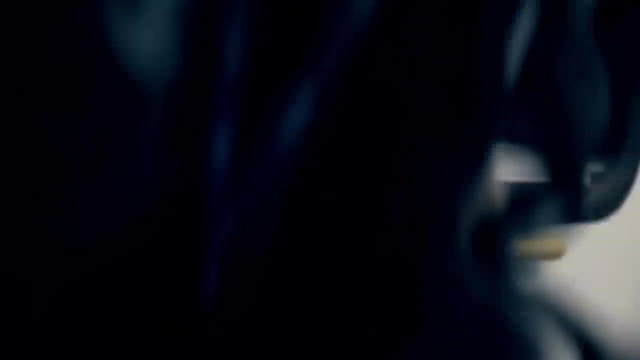 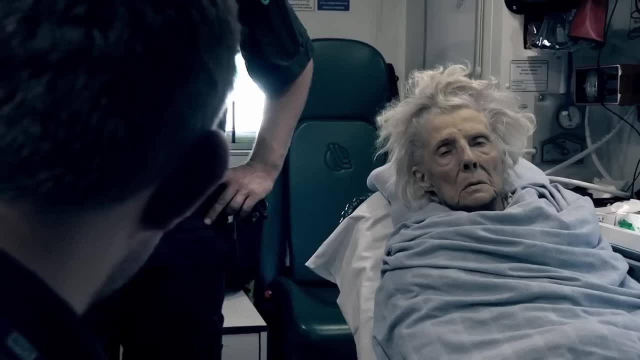 If you're happy, I'm happy not to do that. We don't need to push and pull Mum about doing it. Push and pull, yes. Yeah. no, that's fine. I'm going to give the hospital a call. 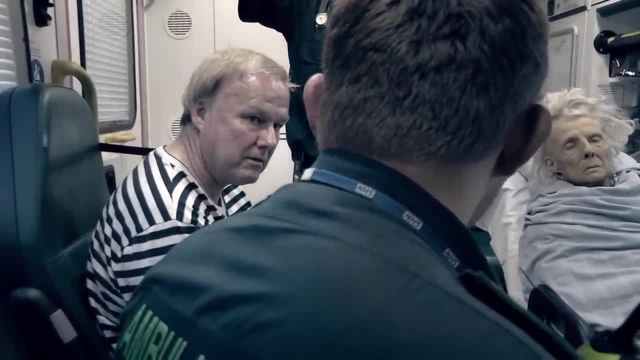 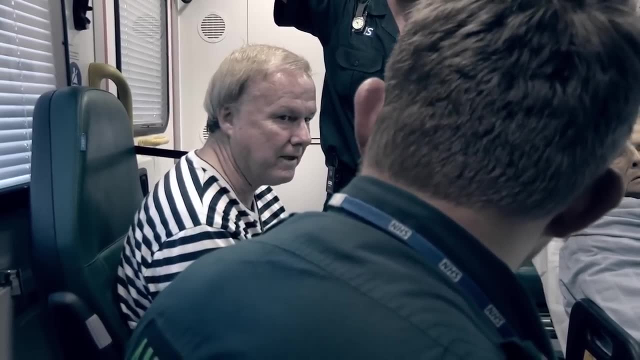 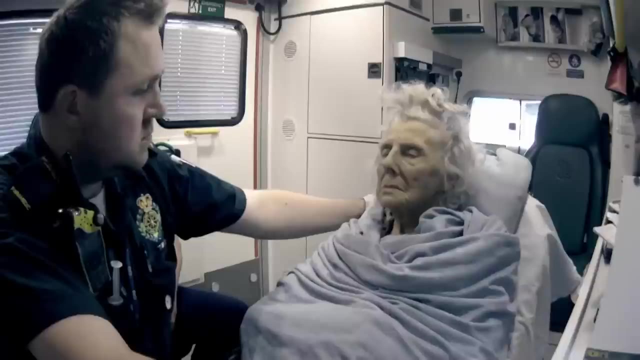 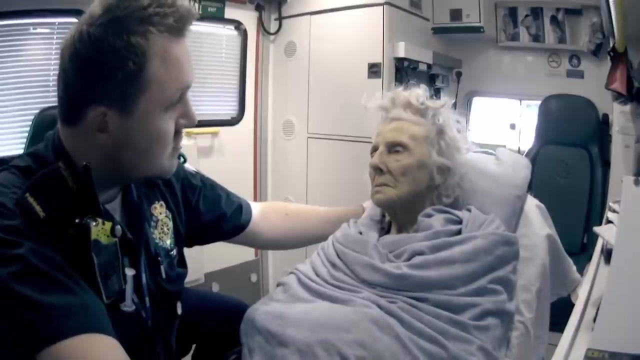 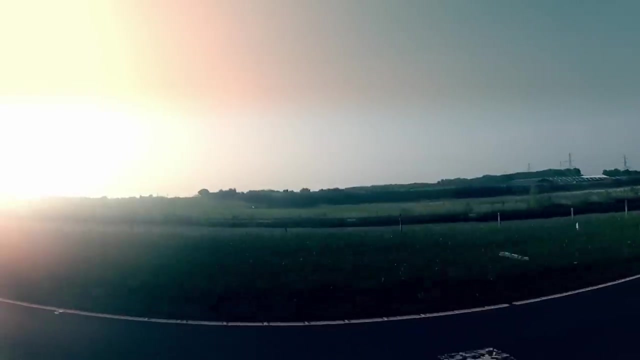 but again we can. Normally we would rush there and blue lights and so on, But again I think we'll just. Yeah, we'll take everything steadily. How's that pain Better, Is it better? Yeah, The day she died. I think I was going to see her about an hour after she actually died, but no, we dismissed it. 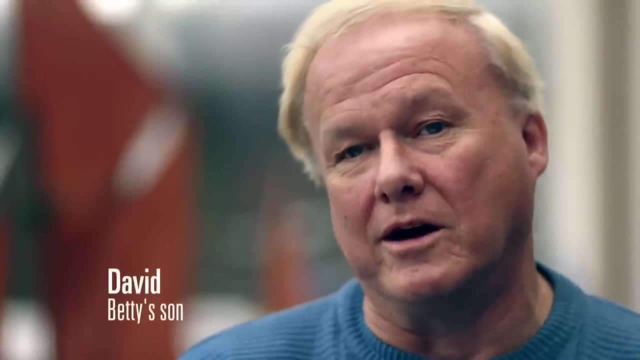 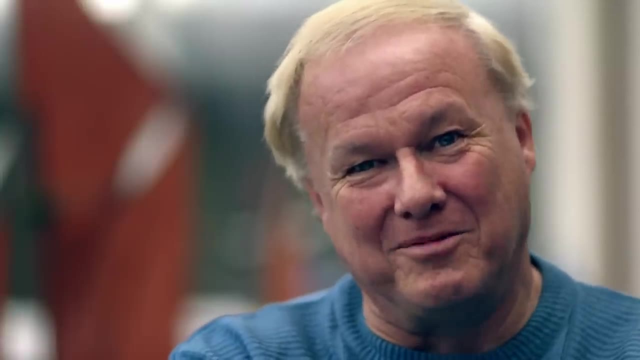 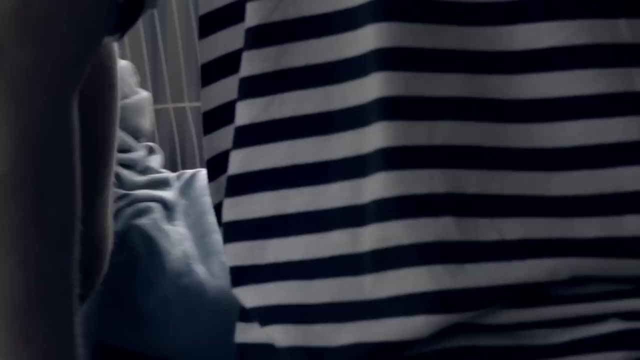 She was a massive sports fan, tennis fan, and it was a time when Andy Murray just won Wynwood and I said to her- I think it was probably the last thing I ever said to her: Andy Murray's just won Wynwood, And I think that was about the last time we had a conversation. She heard that. She smiled, but yeah. 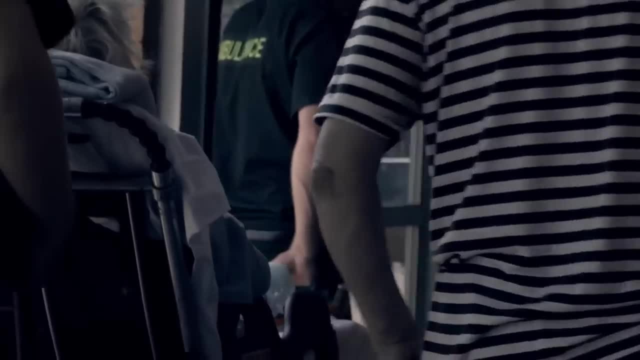 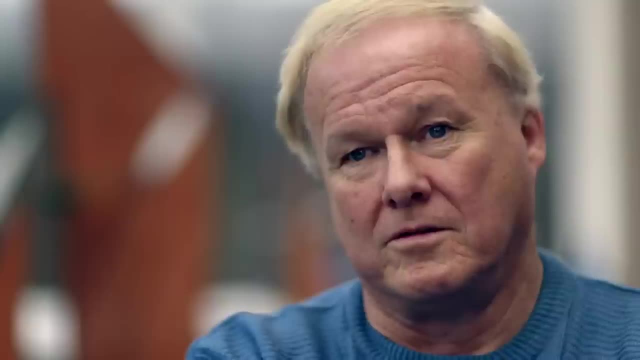 I do think if you are absolutely terminally ill, a senior doctor should be able to speak to somebody and make a decision about bringing it to an end. If it was me, I wouldn't want to be lying in a bed not knowing what's going on for year after year. I don't think there's any point. Hello, My wife's got esophageal cancer. She's just woken up in total agony and she feels like she's dying. My husband, he's had bowel cancer. It's coming up to his seventh year but he's been in such a lot of pain for two days now. Where's the pain? It's in the base of his back. Some people just want to die. Let them pass in peace. They want to go. We wouldn't keep a dog or an animal alive. sometimes Us as humans, we do. I really don't understand that sometimes. 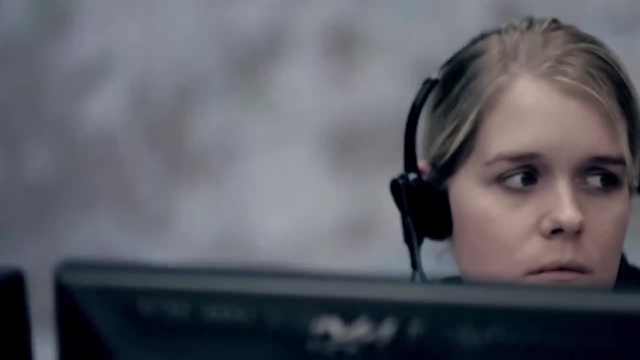 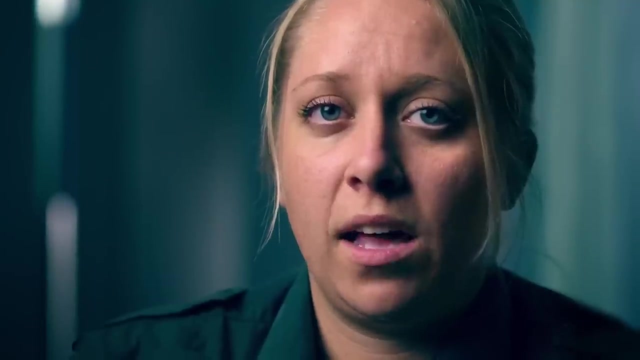 OK. Do you believe that she's beyond any help? I think we should bring in euthanasia. Sorry, I honestly think that we should, especially when you've got long-suffering cancer patients that generally just want to die because they've had enough. They've had enough of the pain. They've had enough of not being able to do anything for themselves. They've had enough of this horrible, disgusting illness that's eaten them up and they want to die. Why should that person die? Why should that person not have that? you know, it's their choice, That's what they want. 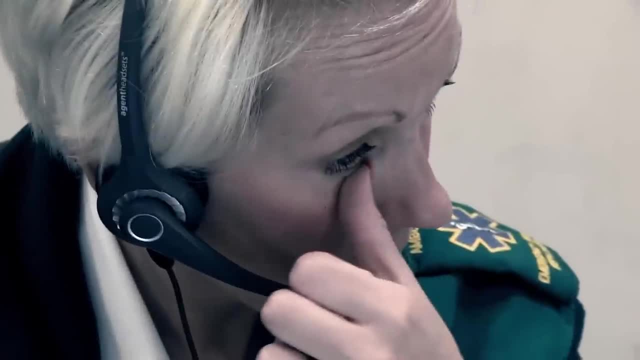 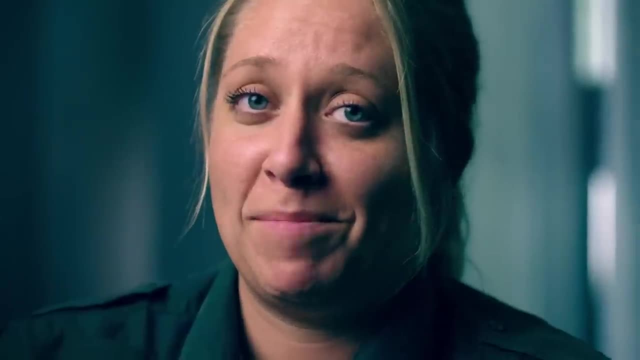 They've been suffering for long enough. Why not let them die? If it was me, that's what I'd want to do. I'd want to die. I just want to be able to go to sleep and never wake up. I'd know how to kill myself. 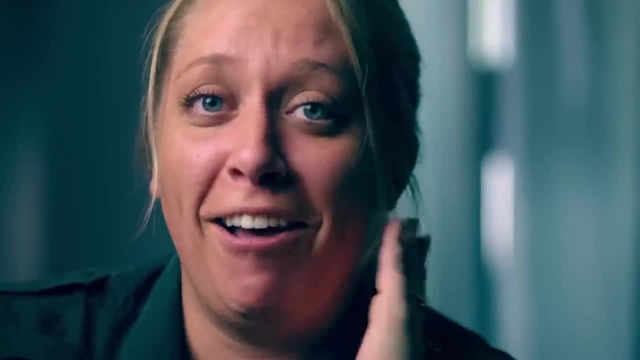 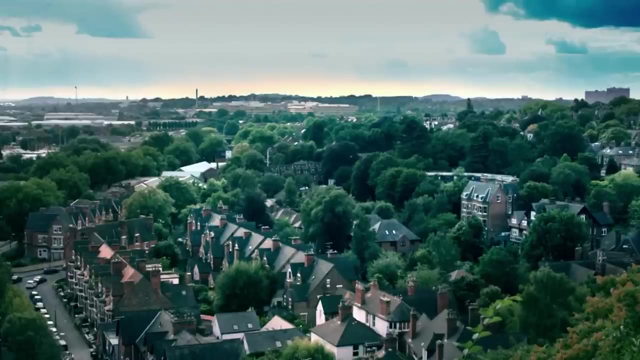 I'm not going to say how, but I'd know how to do it and that's the way that I'd go. Over 170,000 people have died. Over 170,000 people in the UK live with a terminal illness. 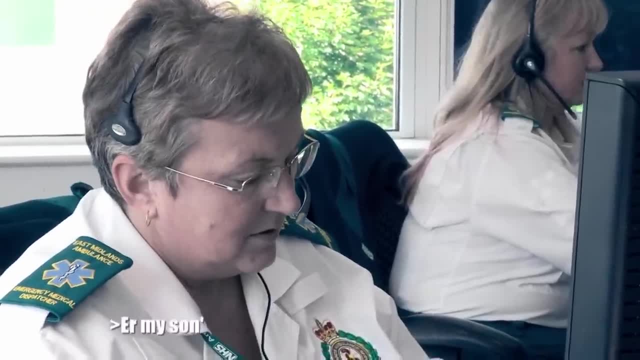 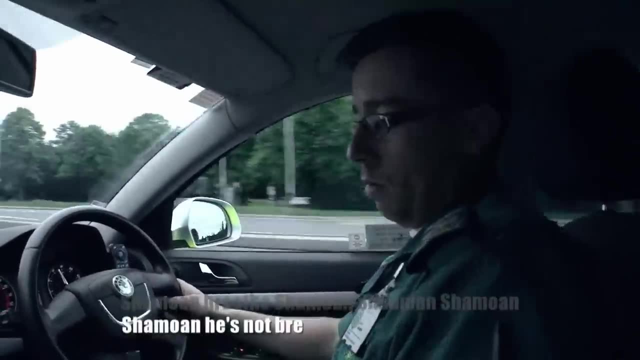 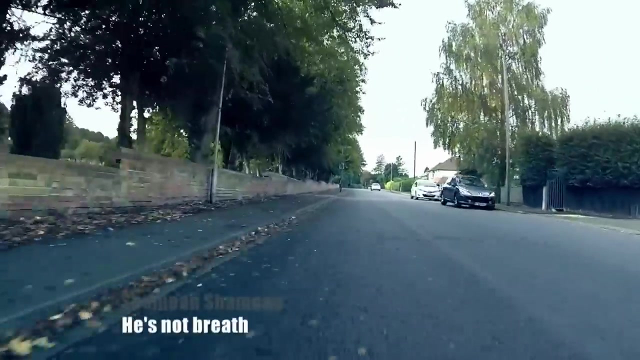 Ambulance service tell me exactly what's happened. My son's having another epileptic seizure. Shimon, breathe. Shimon, Shimon, Shimon, Shimon, He's not breathing. I'm with him, Shimon, Shimon Shimon, He's not breathing. Shimon Shimon, He's not breathing. 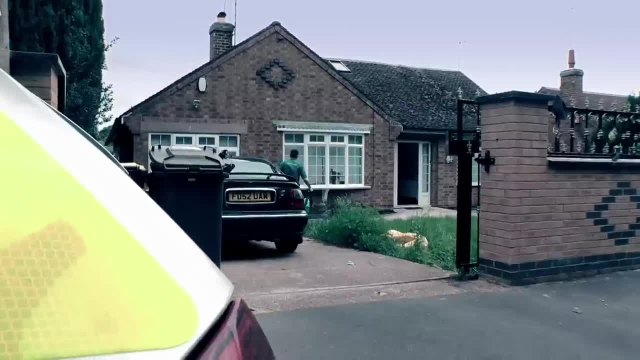 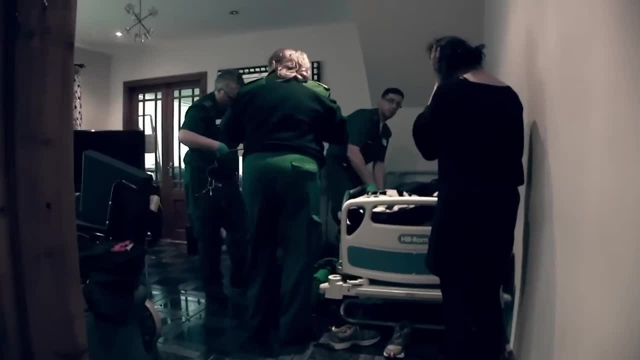 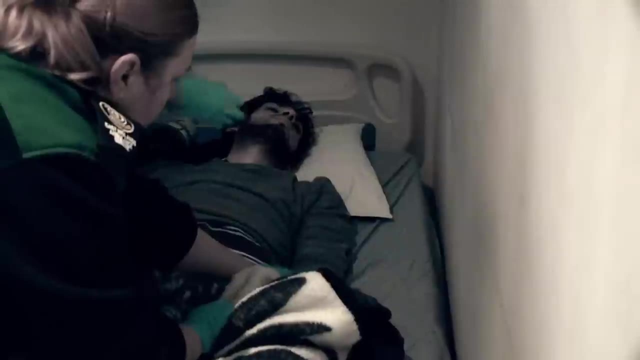 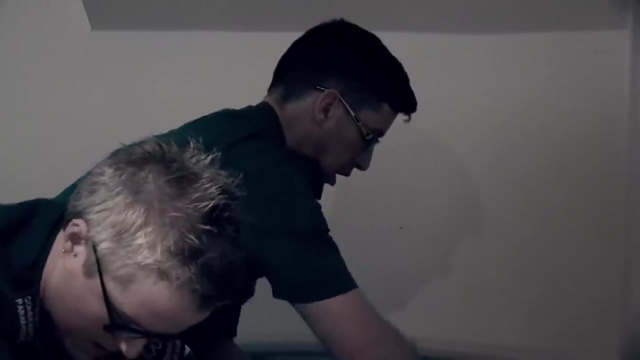 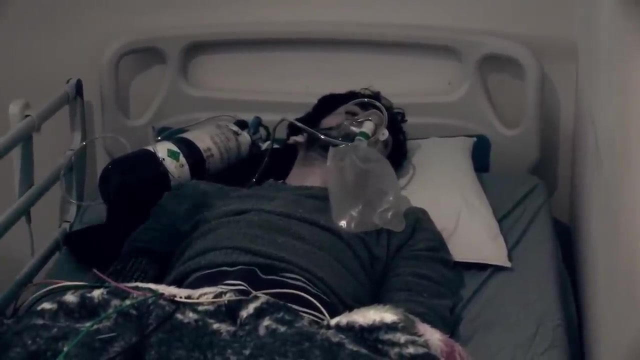 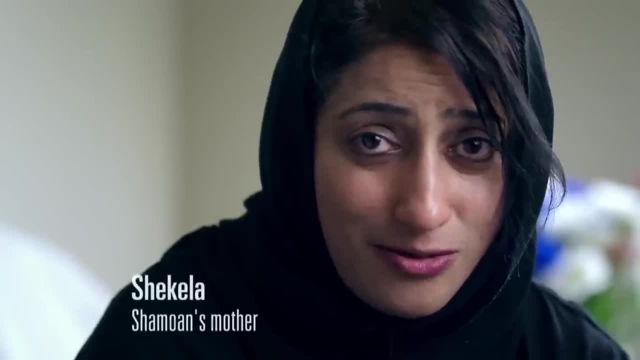 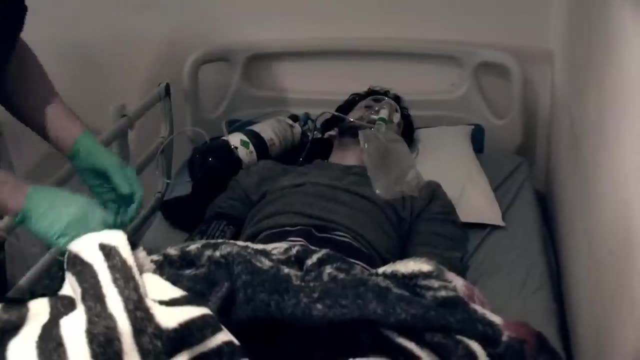 shimon's had a number of respiratory arrests and he stops breathing, and that for us is really traumatic because we don't know whether he's gonna start breathing again or not. so he was awake at the time, was he? it's not as if he's woke from it. he was awake at the time. was he talking to you? wait, he wasn't. 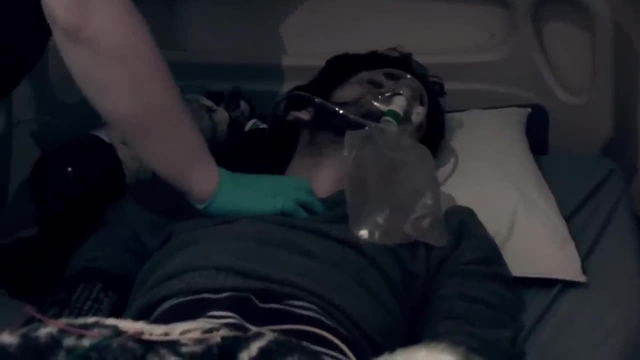 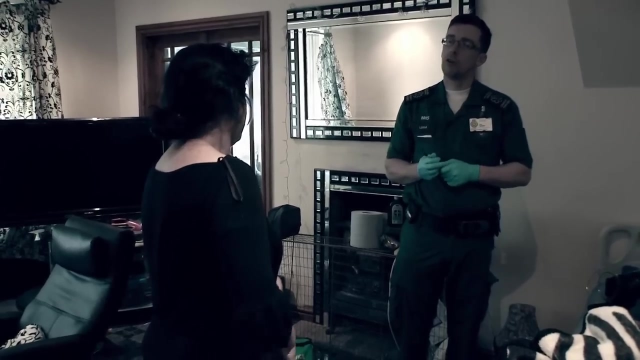 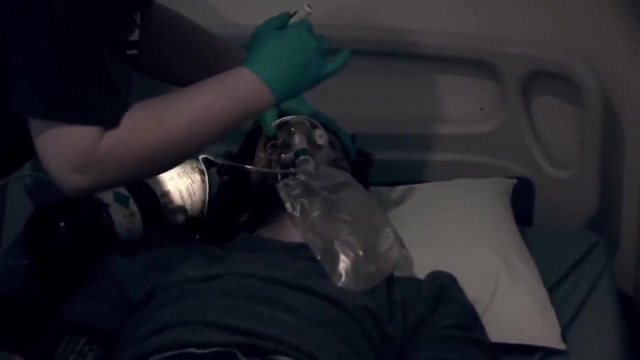 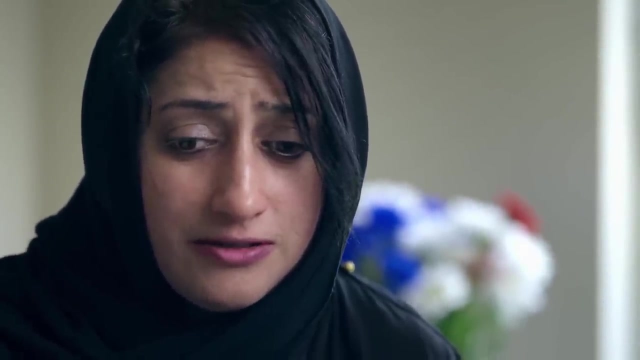 awake. he's got a genetic condition, rare genetic condition. what, what sort of condition? right, what, what, what does that do? what does that present? as he turned 10 when he had his first seizure, they diagnosed lefora. it causes epilepsy, muscle and respiratory problems, dementia, dyspnea, and it causes death within 10 years from the onset of the disease. one: 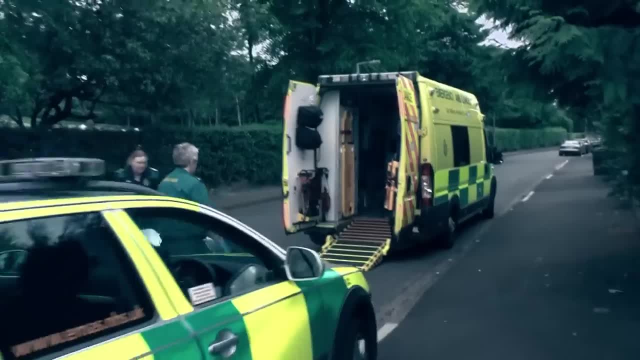 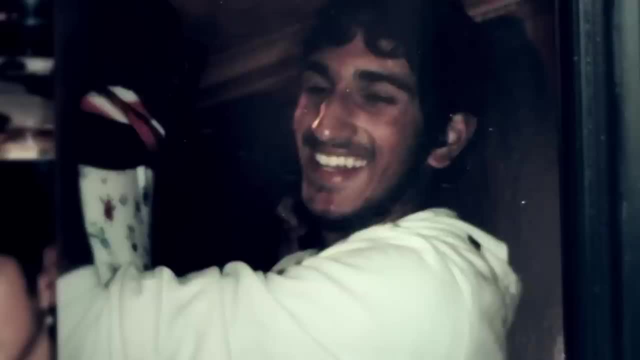 two and three. lefora is a genetic condition so rare there are only six known cases in the country. all three of shimon's had a number of respiratory arrests and he stopped breathing again. shimon's had a number of respiratory arrests and he stopped breathing again. 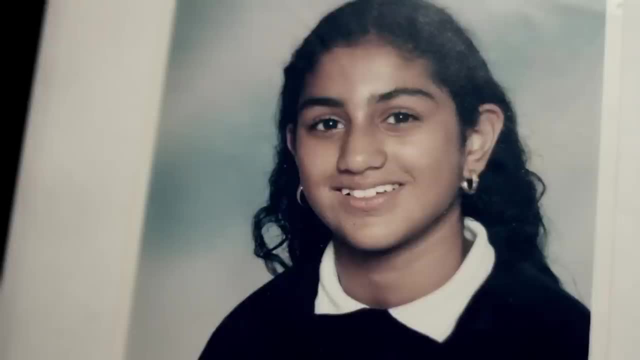 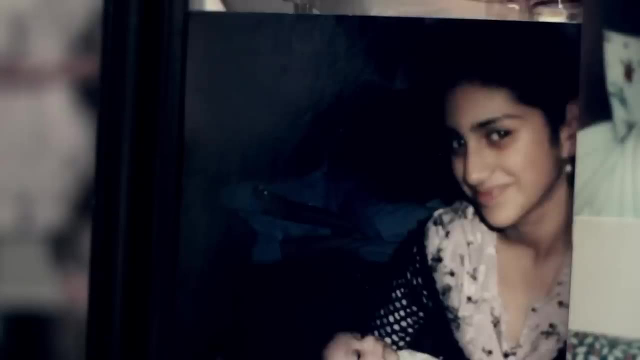 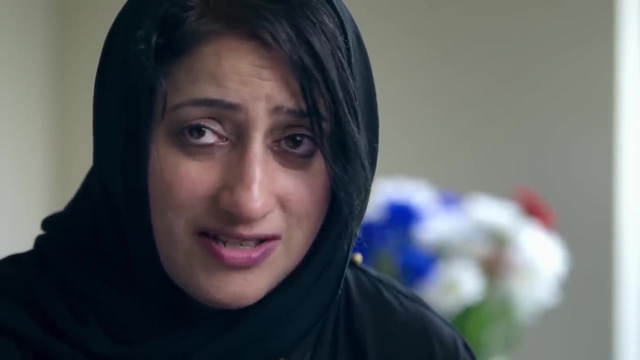 so known, was my oldest child. she became poorly just before a 14th birthday. she was 17 when she died. three years and three months from the date of the diagnosis. she just deteriorated so quickly and there was nothing that anybody could do because she was having seizures after seizures. 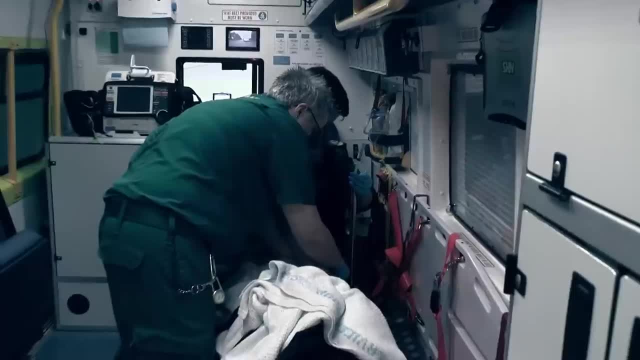 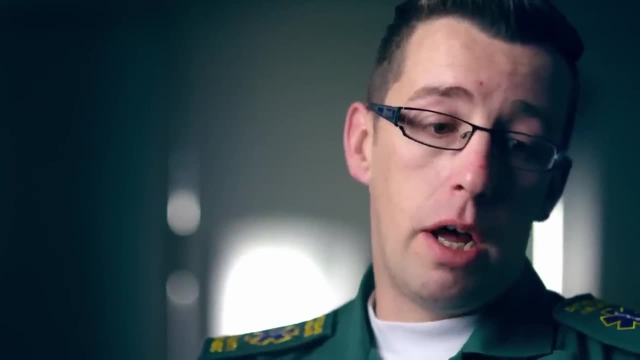 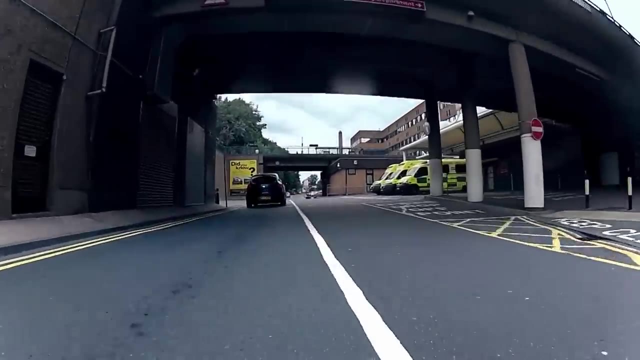 OK, It's all done. It's all done. HE GRUNTS. Nobody likes to see kids poorly. I've got my own now as well, so it's a little bit. It brings it home to you, Although she's probably in a kind of way, used to it by now. 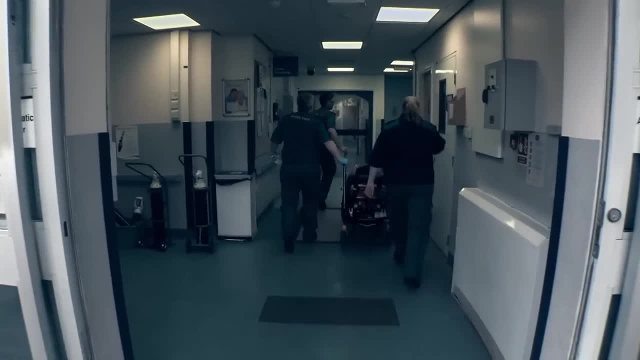 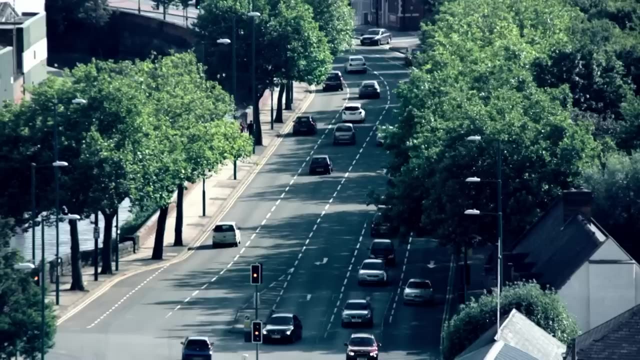 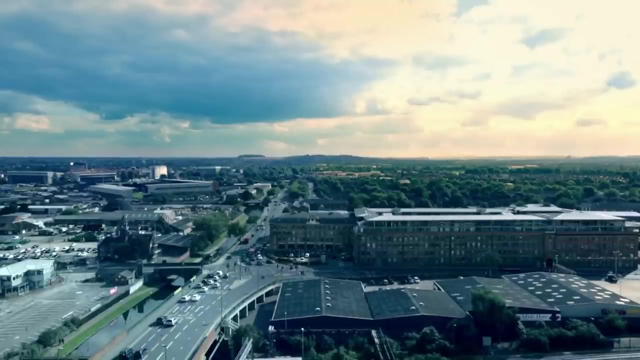 you can never be used to the fact that your kids are going to die before you. It must be really hard for her emotionally As a parent. it must be heart-wrenching. Shimon spent just two days in hospital before returning home. 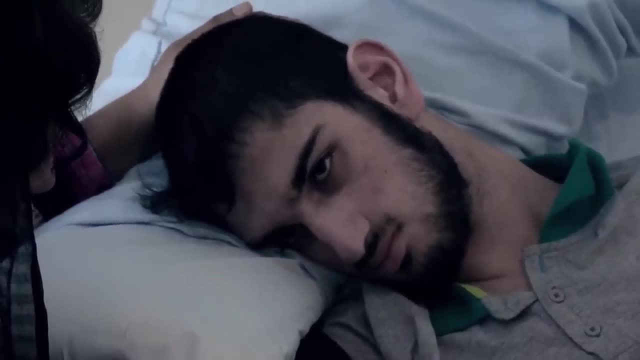 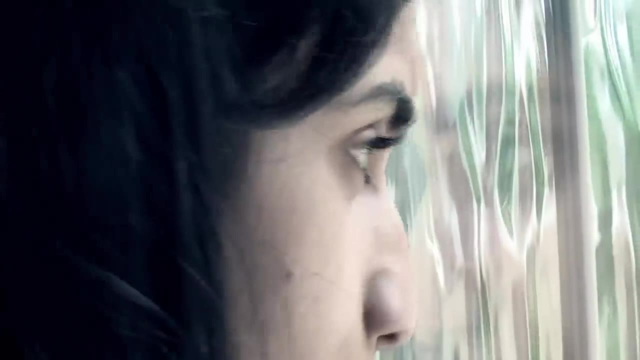 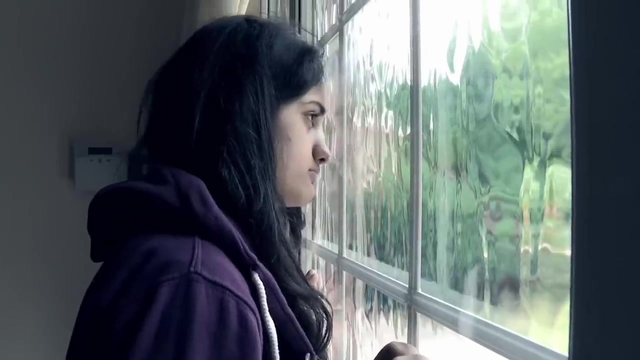 But now, aged 18, he does not have long to live. When Shimon was well, he used to do the gardening, the cleaning, the hoovering, everything, And now he can't do that, he can't even talk. 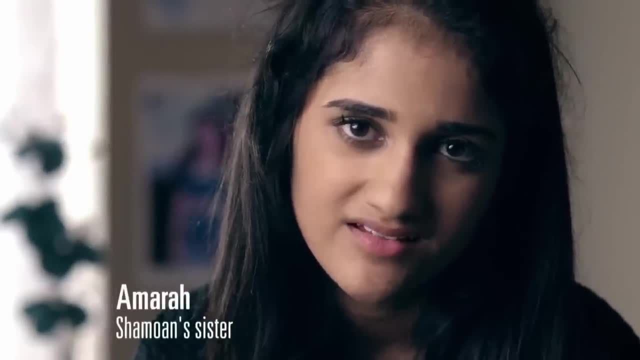 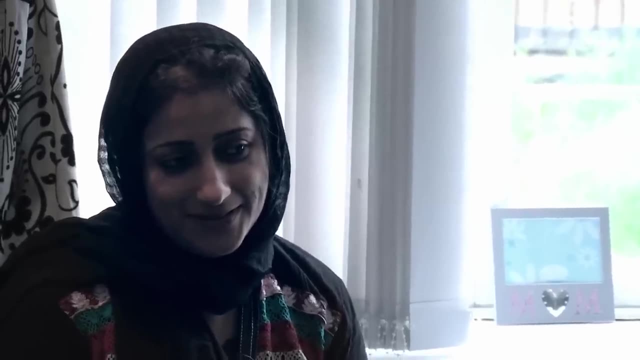 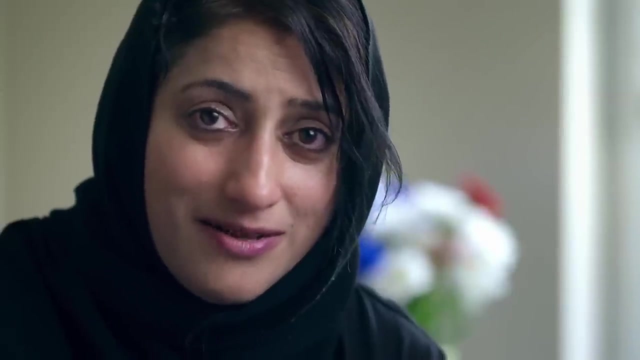 You would think that, oh, one day that could be me. Smile, Smile. Even though they're going to go, I've got to go on for their sake and for my own sake and do whatever I can to the best of my ability. 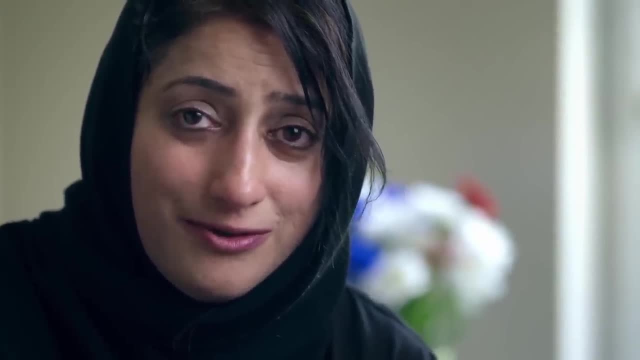 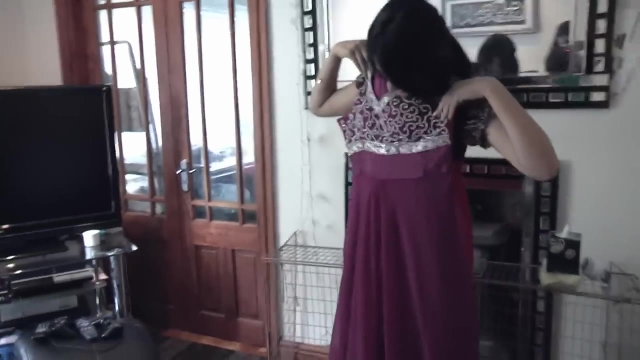 so that, whatever time they've got left, it's got to be enjoyable for them. it's got to be made as easy as possible for them and as comfortable as possible. This is my dress, Yep. The sleeves still need to be put in. 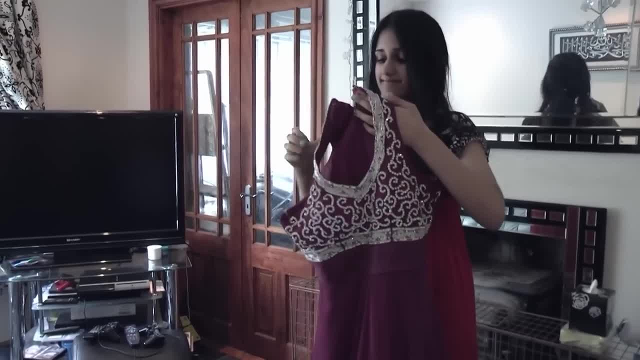 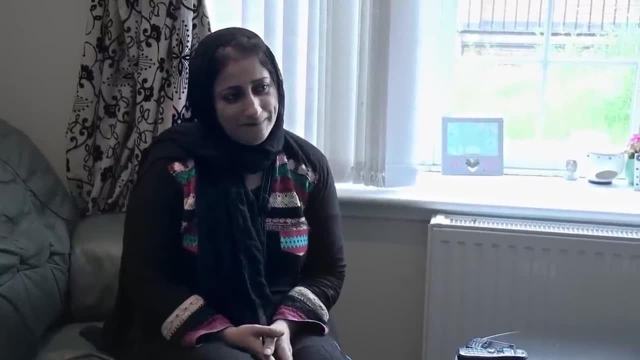 And that's what you're going to wear. When are you going to wear it? On my birthday? Can you remember how old you're going to be 14.. At no point did I show how distressed I really was, because if I showed my children that our mother's 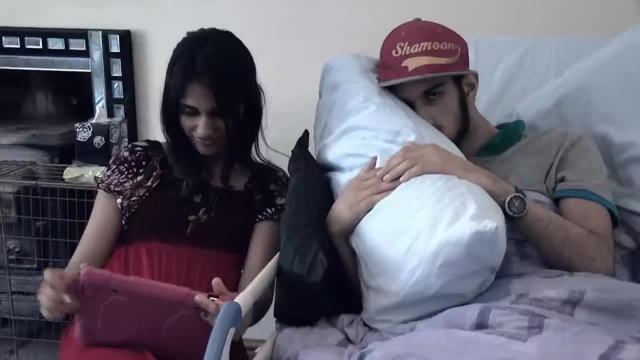 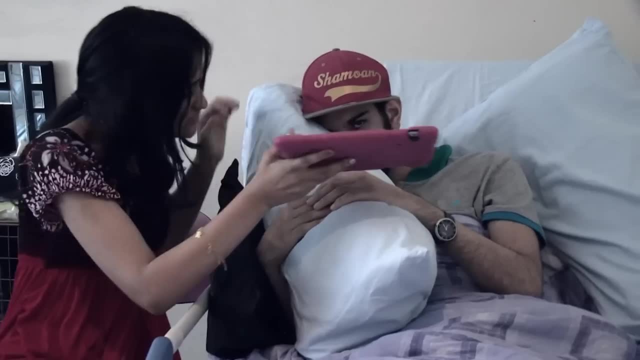 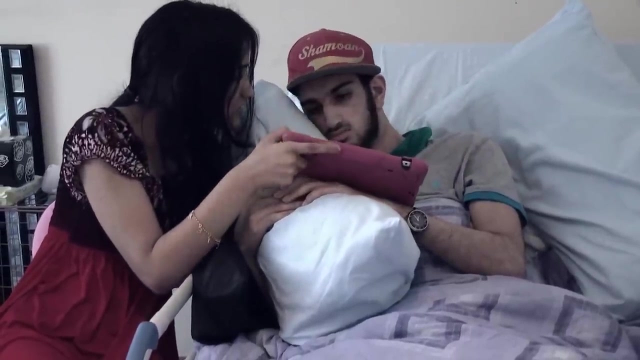 having a nervous breakdown over it all. she's upset. it wouldn't have been good and I didn't want to be a let-down to my children. Smell that. Then one comes a new song: My children, they've had this rich life. 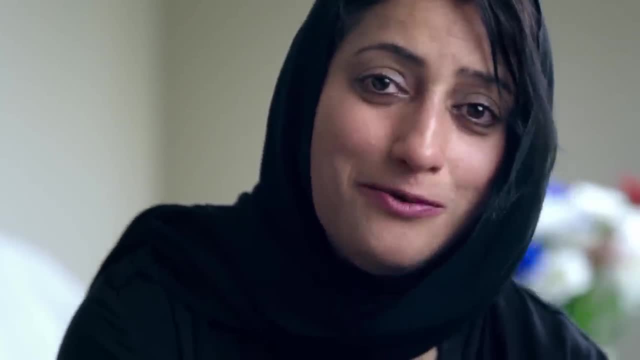 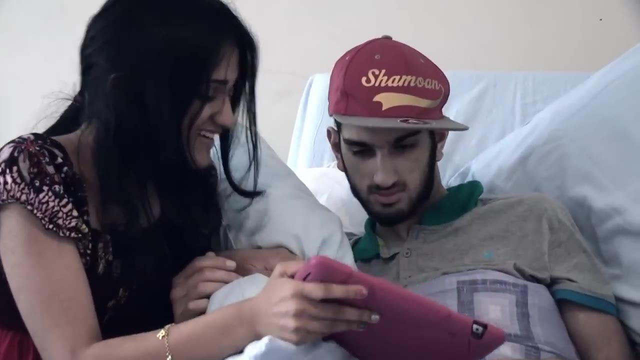 as they call it, financially and otherwise, because they've always had what they wanted. I know I can't give them a life and I can't give them good health, but it feels good to know that I could give them love and anything financial really. 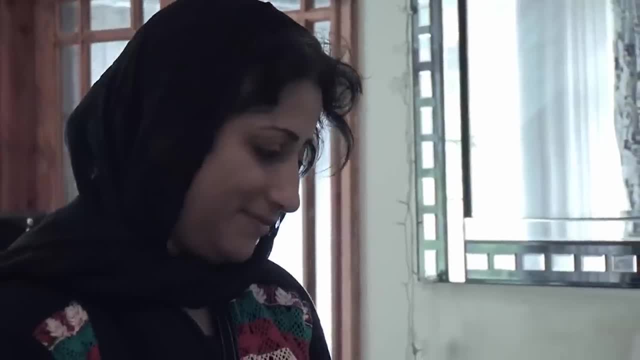 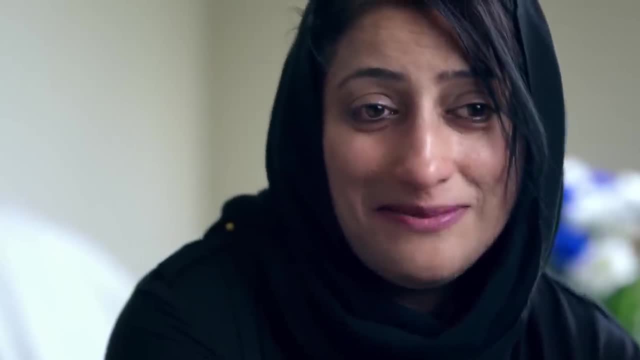 Hold it One. What I've said to the children is: let's take every day as it comes, because we don't know what's going to happen in our life tomorrow. Never take life for granted, because for one minute it could be all fine and well, and the next minute? 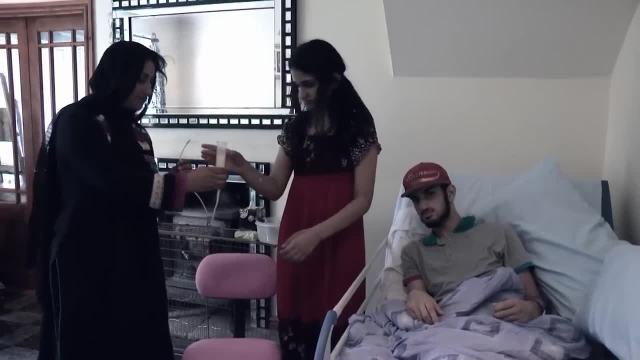 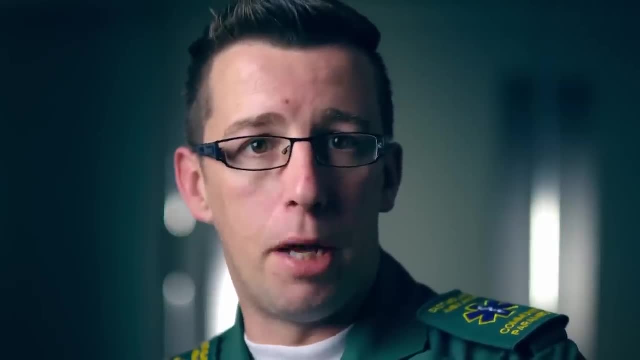 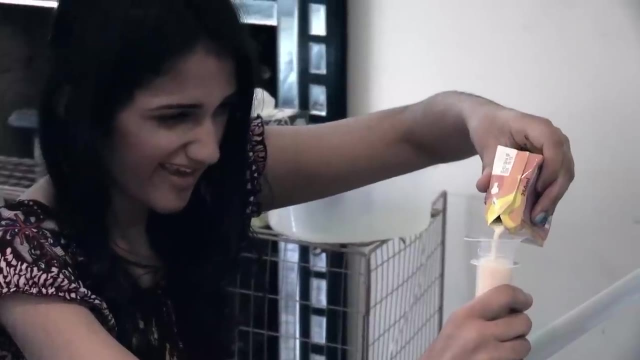 it could all come tumbling down Hold, Knowing inevitably what's going to happen to them. to actually deal with that on a day-to-day basis and still keep a smile on their face is remarkable. It's absolutely amazing. It's not something I could do. 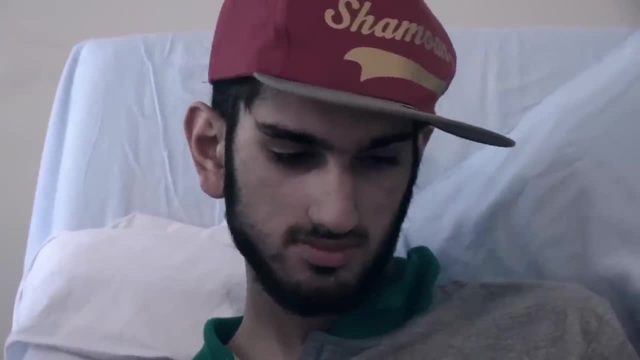 You know it's all right. people say I couldn't do your job, but my job is my job. This is not a job, this is a life. I don't know how I'd cope with it, even given all my medical training. 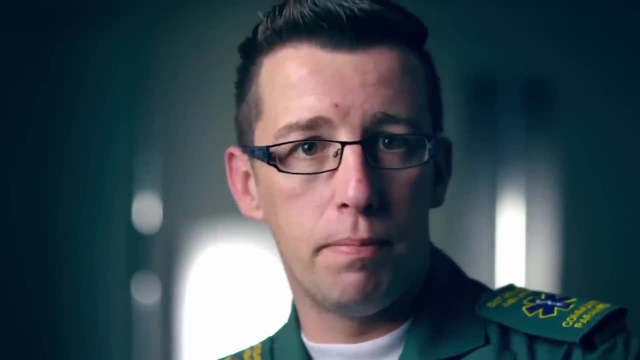 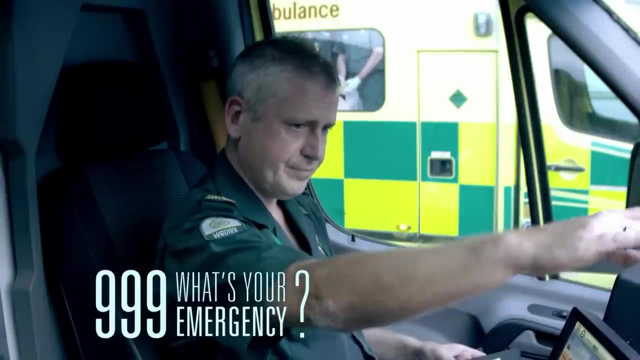 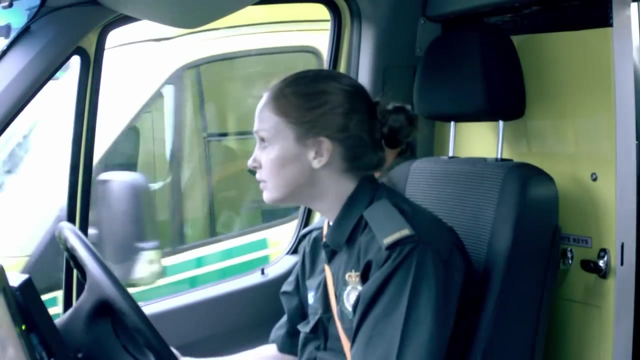 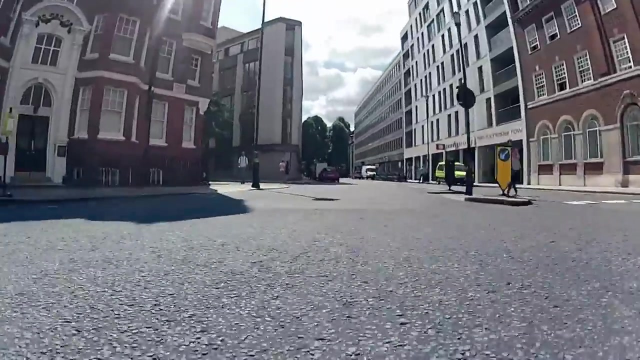 I don't know how I'd cope with a member of my family, or three members of my family, going through that. We have got An emergency. Oh bless. 87-year-old female fallen query, fractured wrist and shoulder injury. What's hurting, darling. 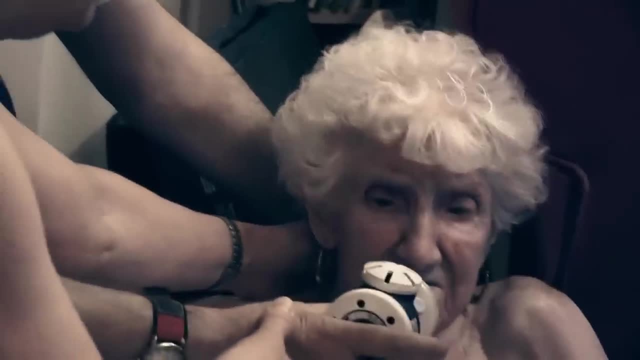 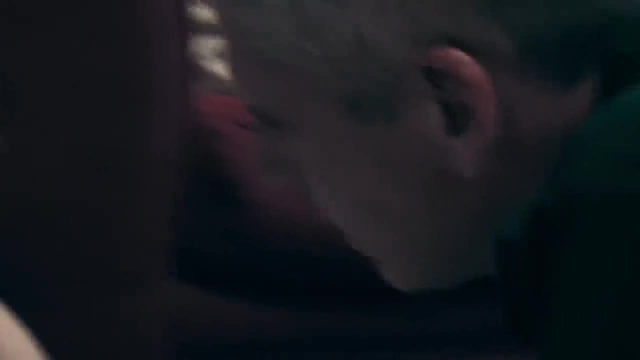 Your leg, Your leg Right. let's take some deep breaths for this. Ida. how's that magic gas doing? Is that all right? That's a lovely wink, isn't it? She's winked at him. It's just my tumour. 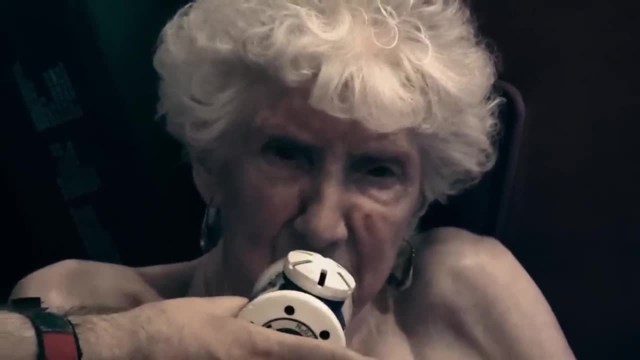 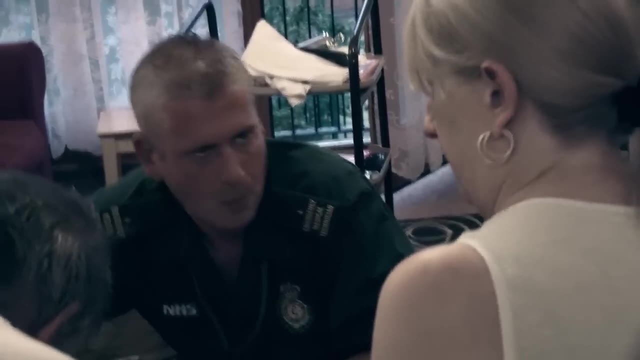 Are you in it, Ida? No, Obviously. what we think has actually happened is that she may have actually fractured her hip Again, again. OK, You can see the way it's, You can see the angle it is. 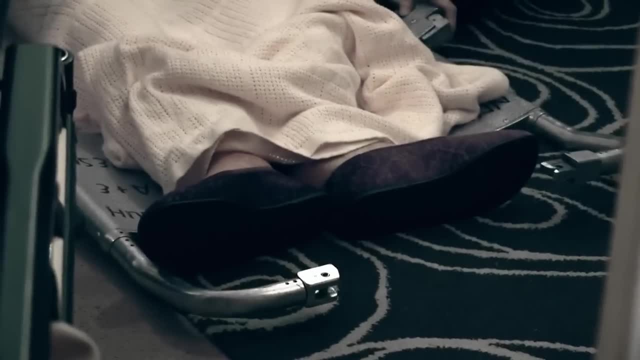 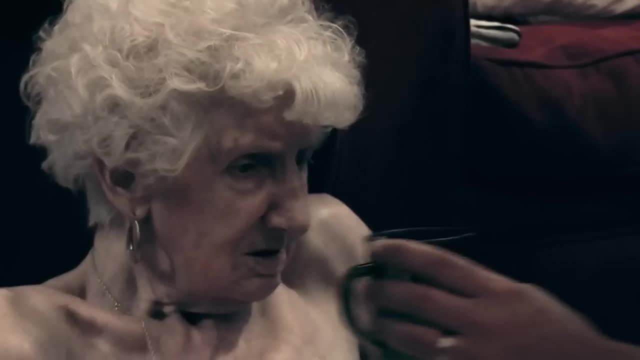 You know, it's not rocket science that it's probably broken. I bet she was getting ready to get undressed herself in her nightie and that's how she's fallen lost her balance. Here you go, sweetheart. I think the family had an idea. 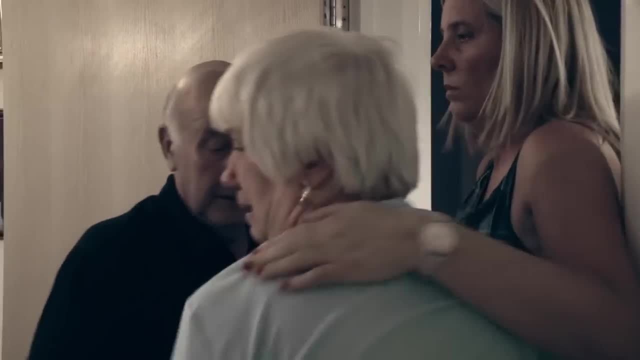 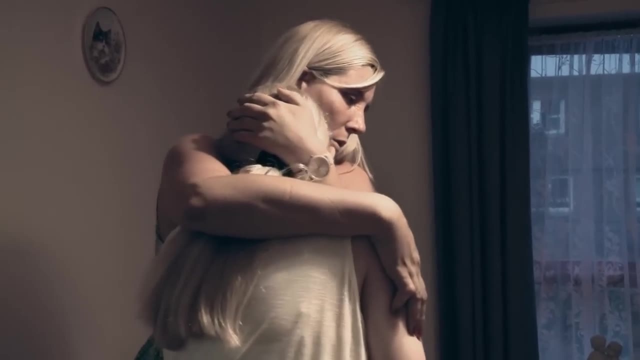 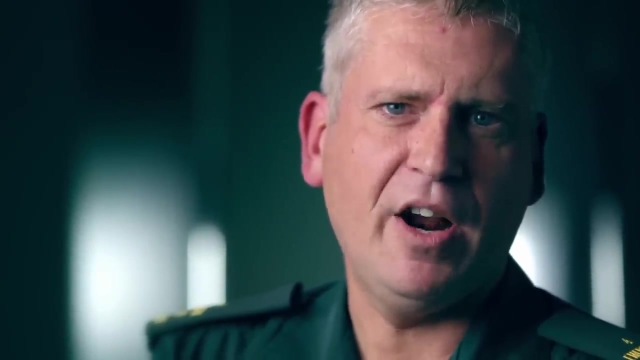 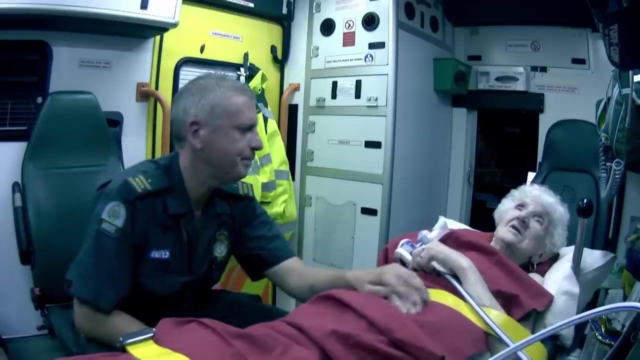 especially one of the daughters, that Mum wasn't quite right. She ain't got to survive this. Some people have this instinct that they know that they're not going to be with us for much longer. You all right. Yeah, that does hurt, though. 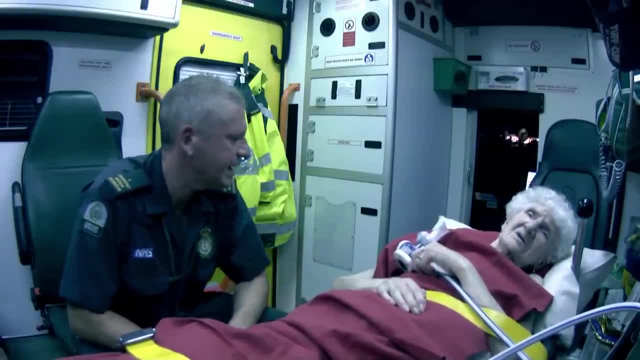 I know, don't I? What we'll do is, when it gets to us, we'll look for some stronger pain for this. Oh, it'll do, eh, I know. All right, Mum. Mum, we're nearly there. 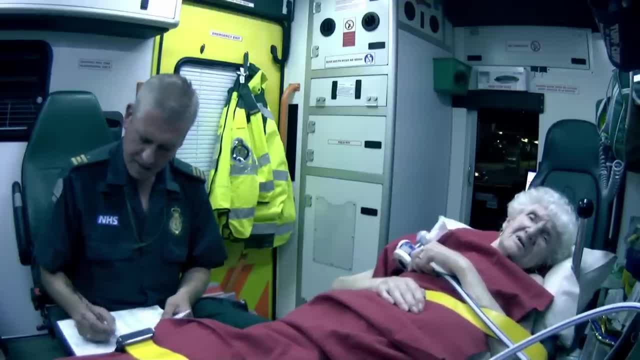 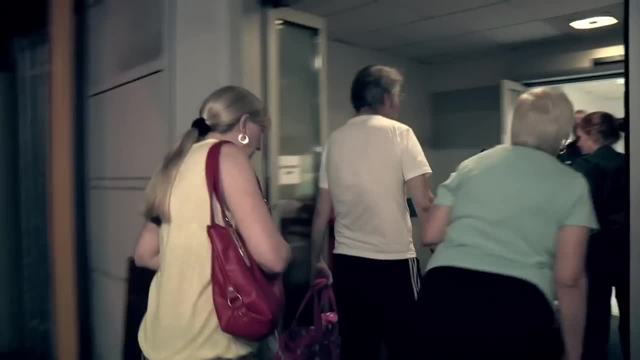 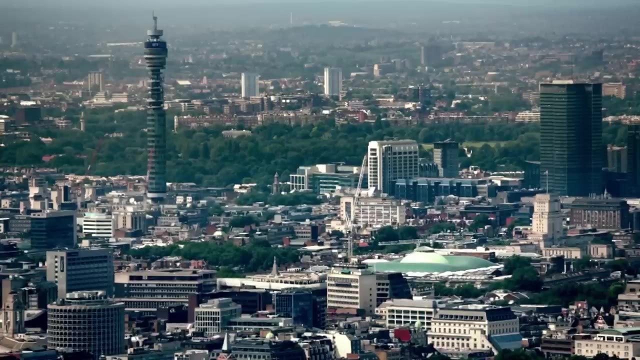 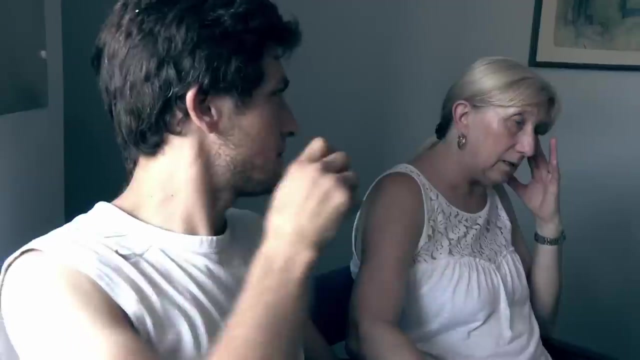 He did so much for Mum. We calmed her, made her comfortable. They were so gentle, He was a star. The hardest thing I've done is to say: do not be sad. But you didn't do. I don't want it to stop, no more. 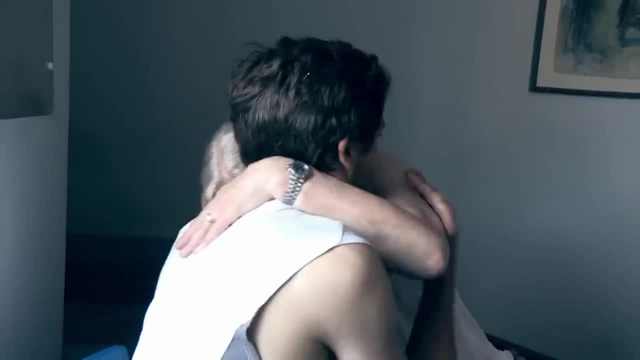 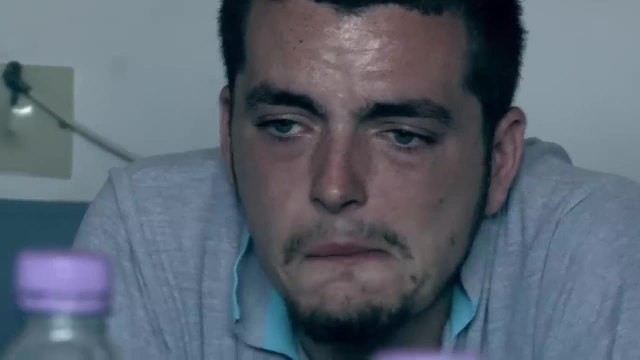 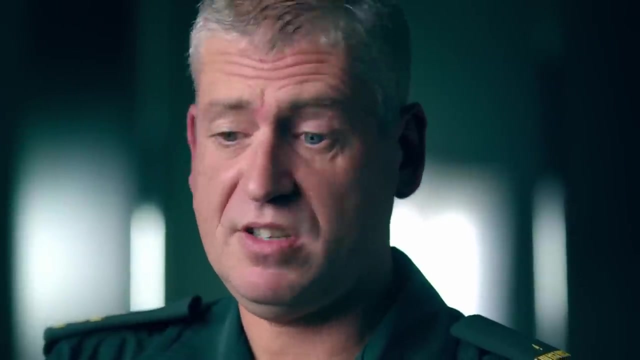 cos I love that Death is always painful. Everything is churning up. All of a sudden it just explodes and it just it has an outpouring, Because we all know we're going to die. You know, say death is natural. 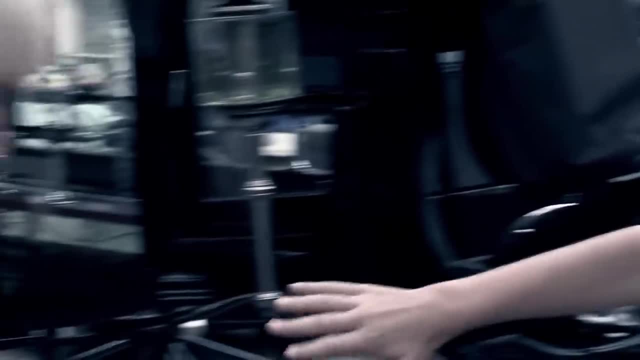 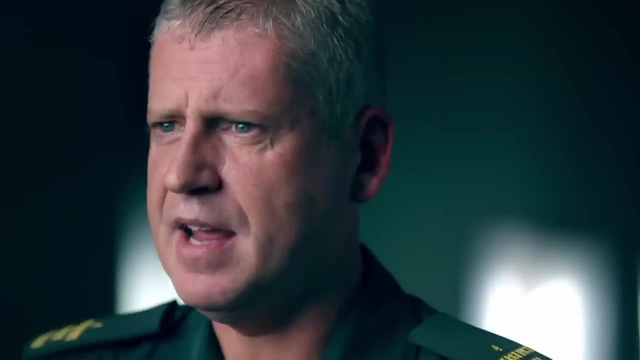 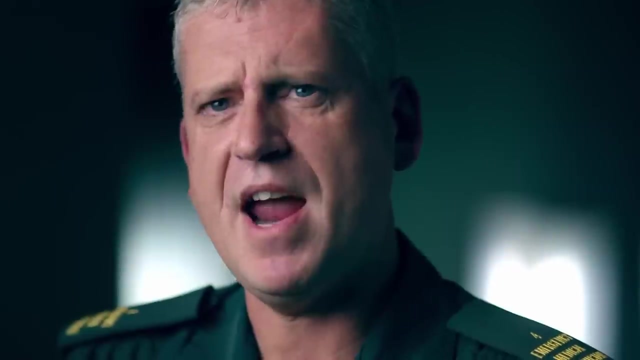 But we are human at the end of the day. We do have feelings. I lost my mum three years ago to cancer And then, five weeks later, I lost my dad to a massive heart attack just after Christmas, So lost both parents within the space of five weeks. 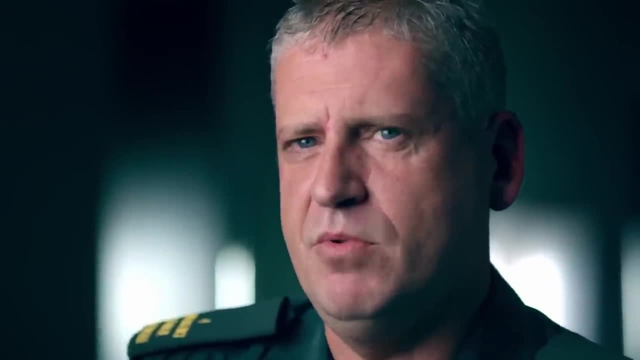 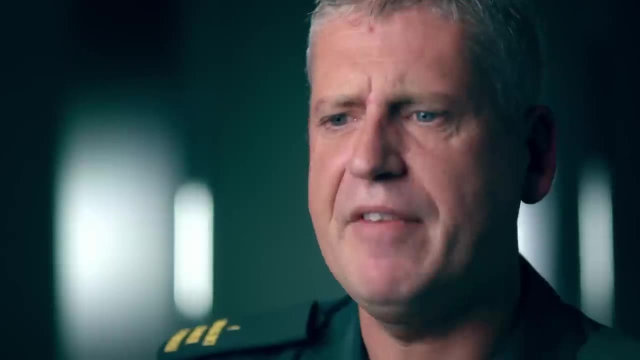 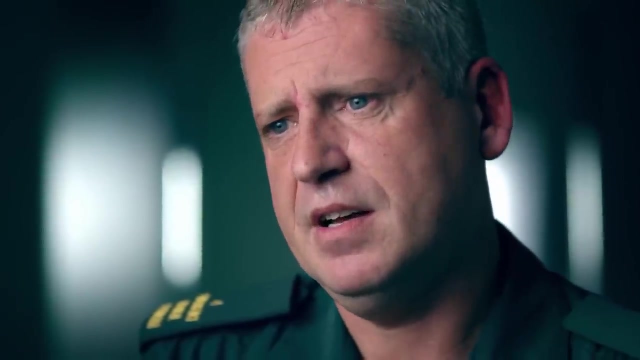 So it does make you question your mortality slightly. But when you actually go in day in, day out dealing with life, death situations, seeing children being or babies being born, and then dealing with a deceased person, you know we've had many a shift. 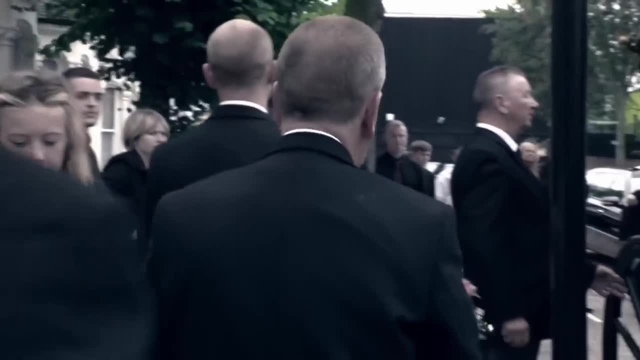 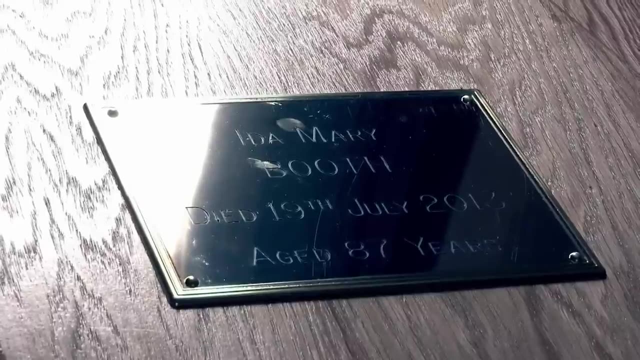 where we've dealt with a patient who's died, Then on to the next call, where we've actually delivered a baby. Where there's death, there is life. SHE SNIFFS, SHE SNIFFS. Mum, I love you so much. 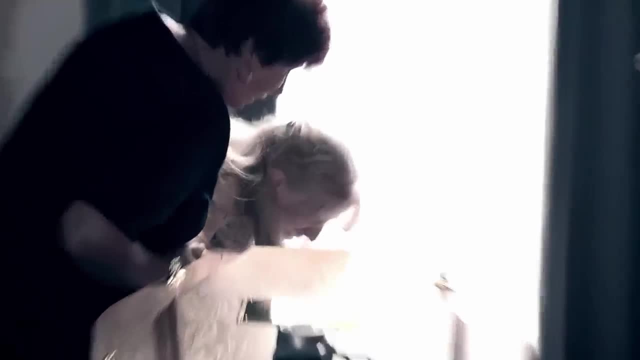 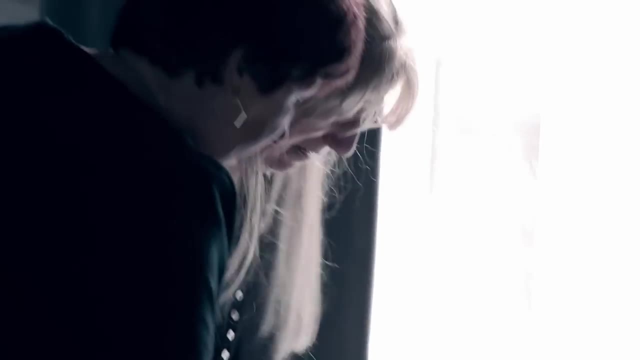 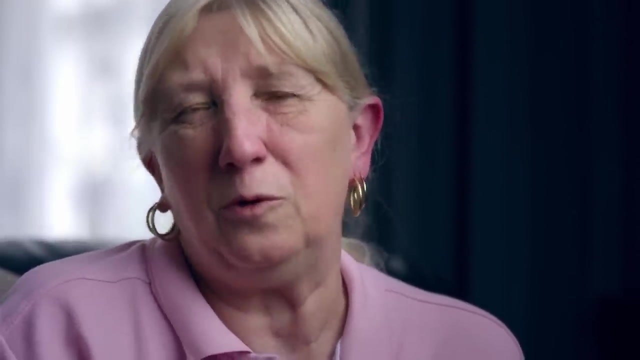 I love you so much. Please come and see me, Be with me. I love you. She was a joker, She was a tough lady And she was very stubborn, But we all knew how Mum was and we just loved her to bits for everything. 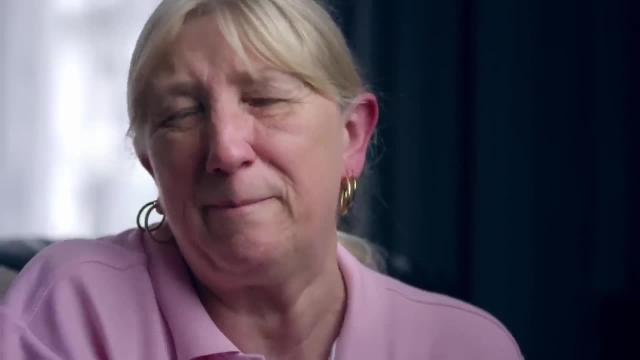 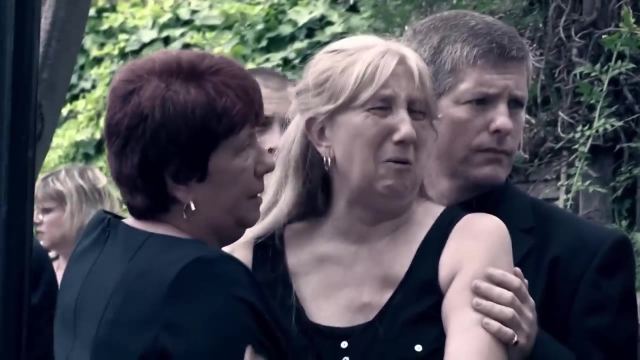 that how she was and who she was. wouldn't want her any other way. I know you're going. You're going in style love. You're going in style Beautiful. Funerals, inevitably, are sad occasions. They speak to us too eloquently. 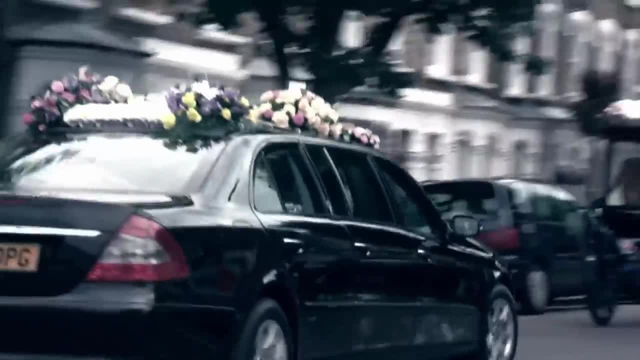 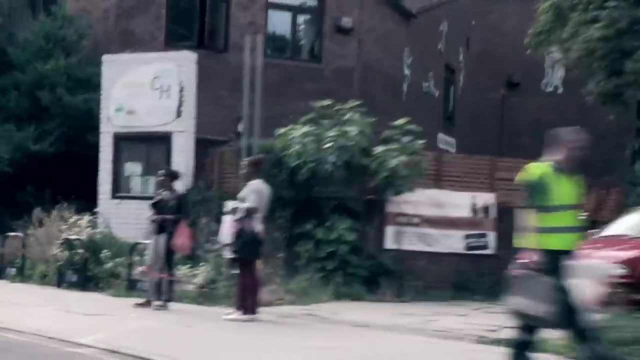 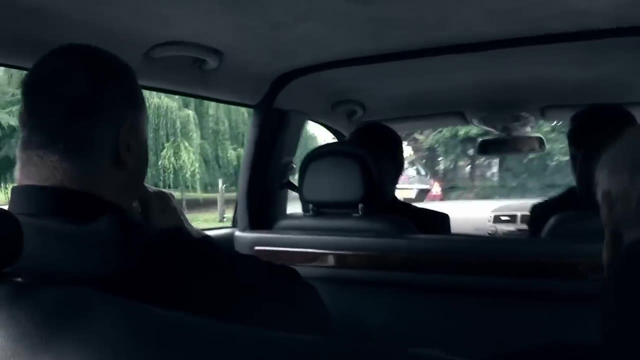 about the reality of death And our own sense of personal loss. Maybe they say something also about just how very precious is the gift of life, Not only of the life that was Ida, but your lives and what you do with them. Ida Mary Smith was born on the 28th of March in 1926. 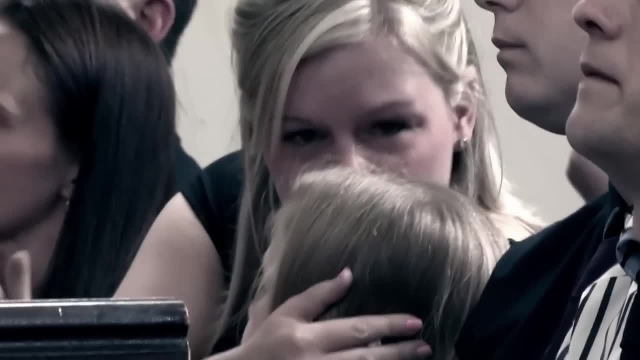 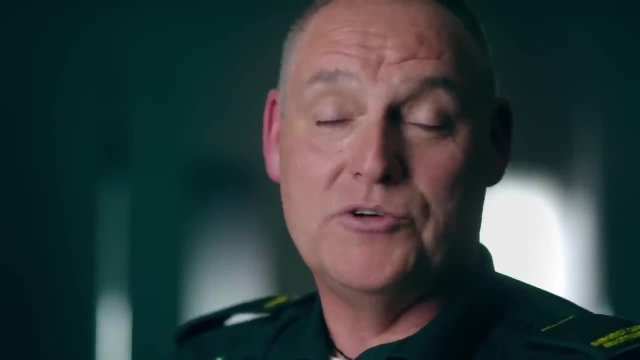 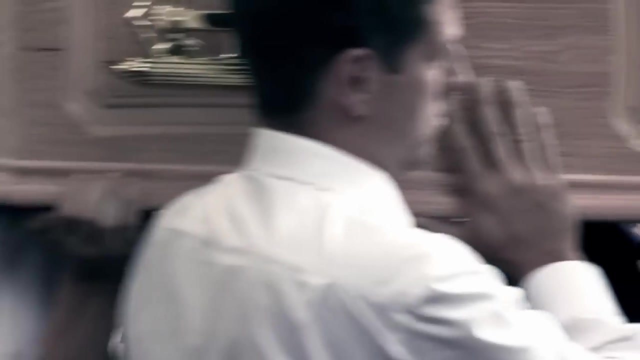 in Stone, Stoke-on-Trent. You'll never forget the people that pass. You just don't see them anymore. They'll always be in your heart, in your head, in your thoughts. I miss my sister-in-law and my father-in-law really badly. 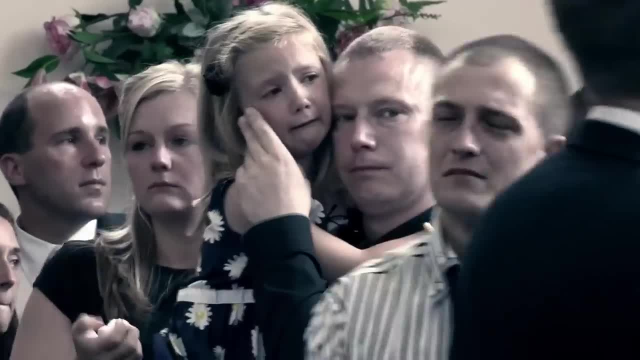 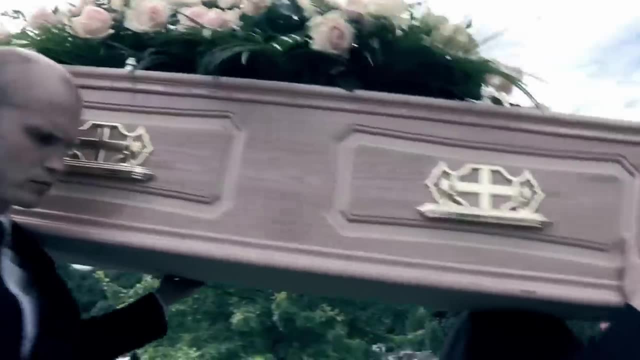 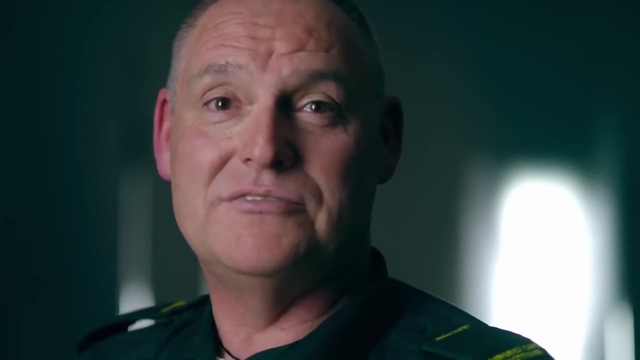 but I've got to think of all the good things they gave me. It does help to mourn. It's for your own benefit, not for theirs. You've got to mourn, you've got to talk to people. It's our way of dealing with life. 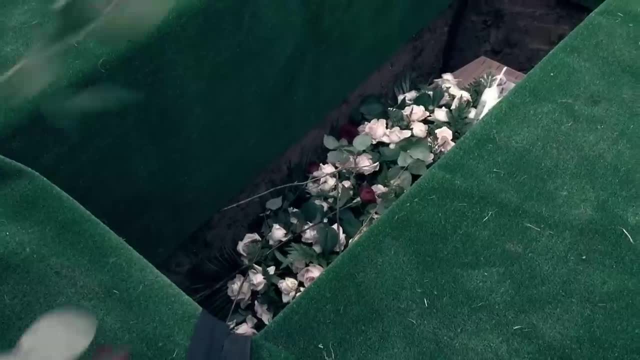 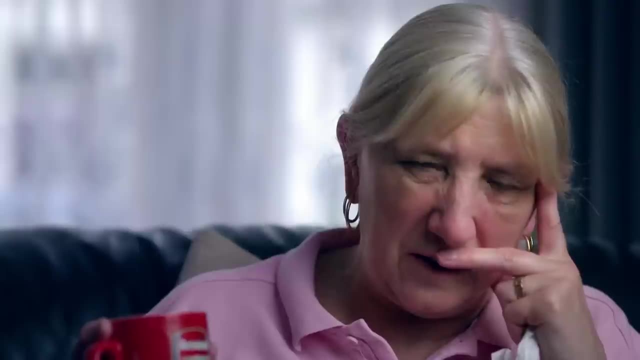 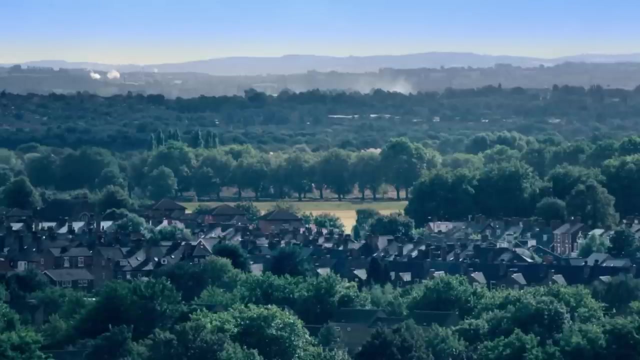 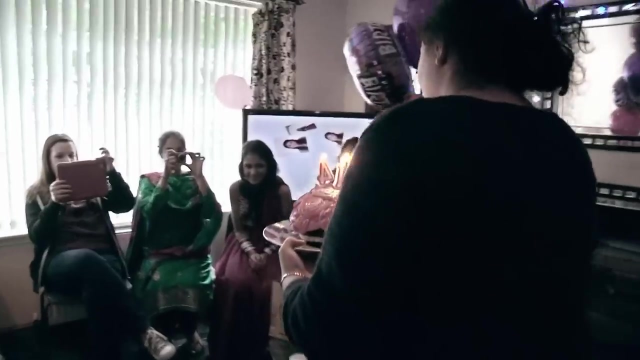 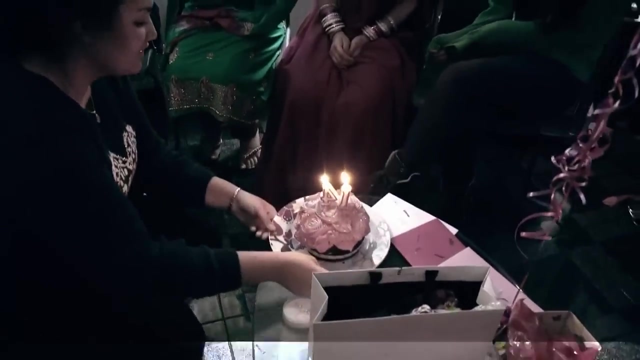 Love you, Mum. May she rest in peace and rise in glory. Amen, Amen. She would have loved. She would have loved every bit of it. I'm sure she was watching. Happy birthday to you. Happy birthday to you. Happy birthday, dear Amara. 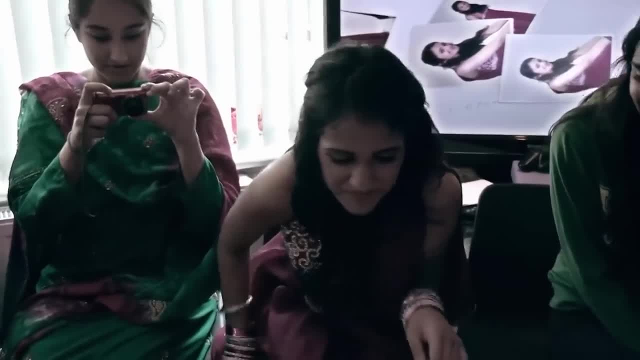 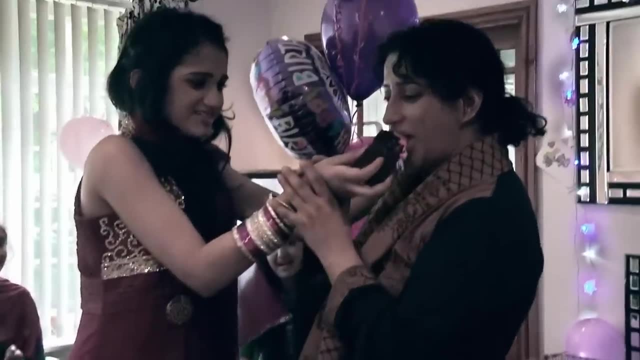 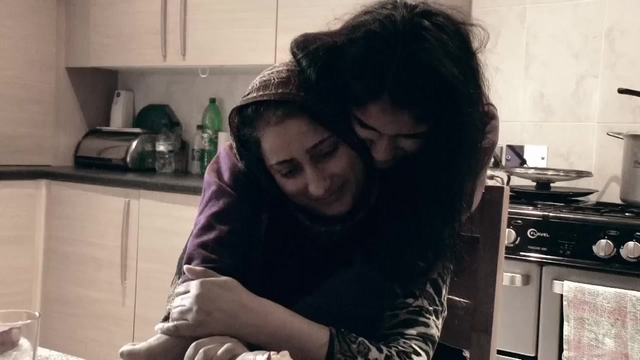 Happy birthday to you, Whoo. I think my mum. she's really strong and brave Because after what she's been through with my sister and now my brother- next knowing it will be me- you could say she's the best mother in the world. 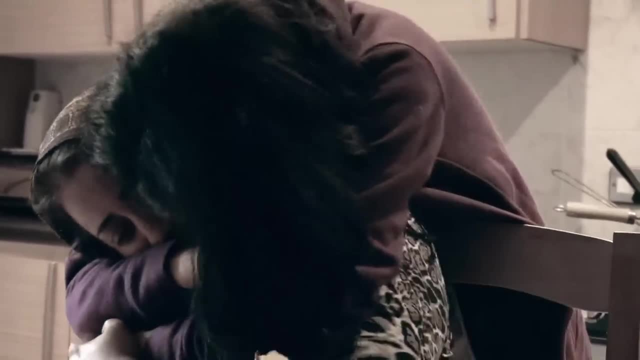 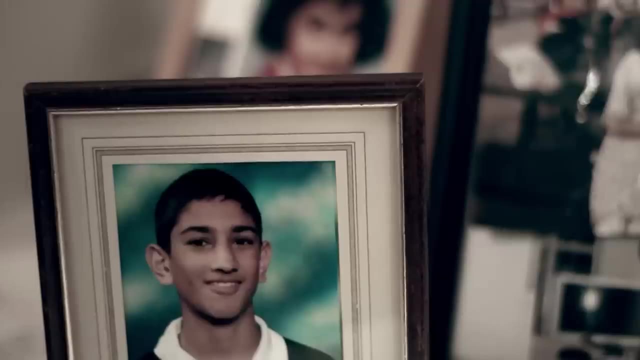 I think they've all been strong-willed and remarkable children. really, It's not easy for you to watch your older sibling die and then for yourself to deteriorate, and then you know that your other sibling's going to go. They've been considerably strong. 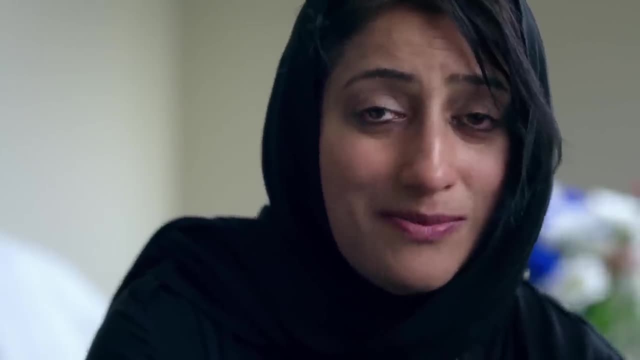 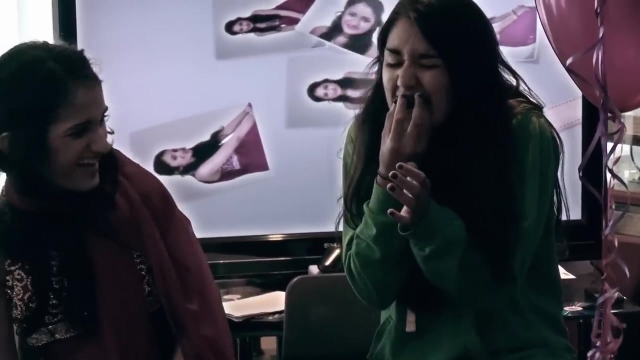 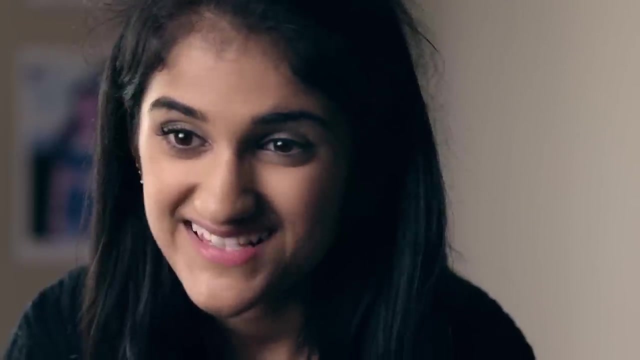 And the fact that they keep going, despite knowing that things could deteriorate at a moment's notice. You must be like a really strong, tough teenager. You deal with a lot more than most other people your age, I guess. it's life: you have to cope with it. 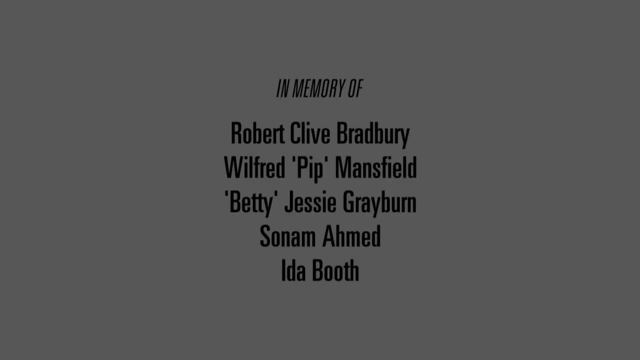 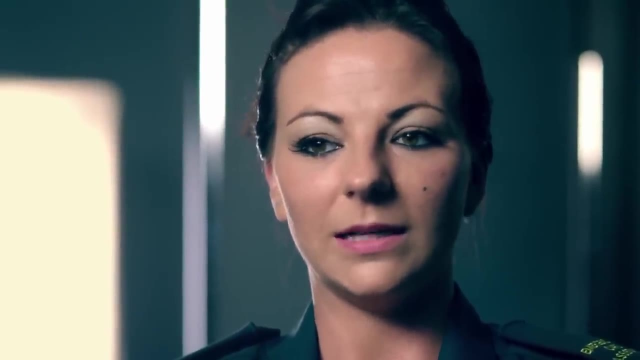 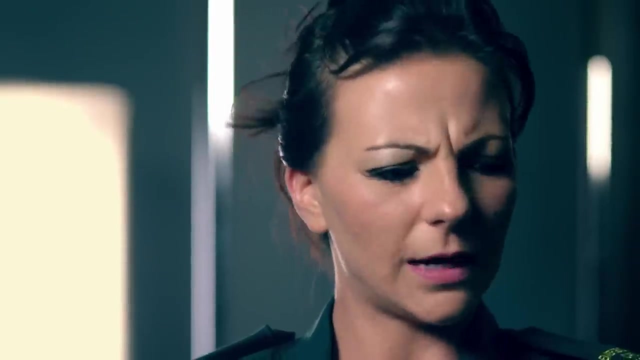 You know, at the point of death, obviously it is horrible for any family and relatives. So you don't want the added extra of trying to figure out what that person would have wanted, what flowers they would have wanted, what music they would have wanted.